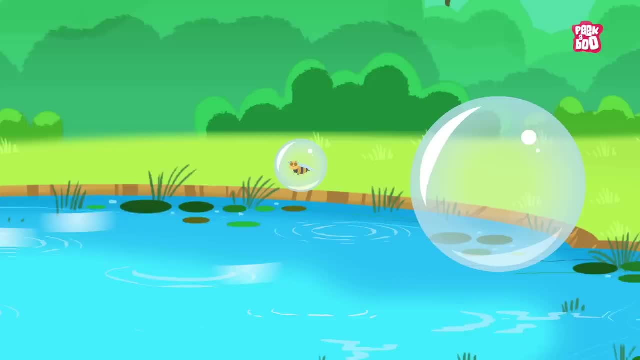 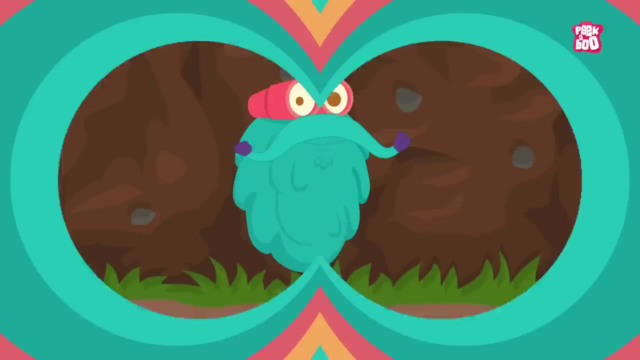 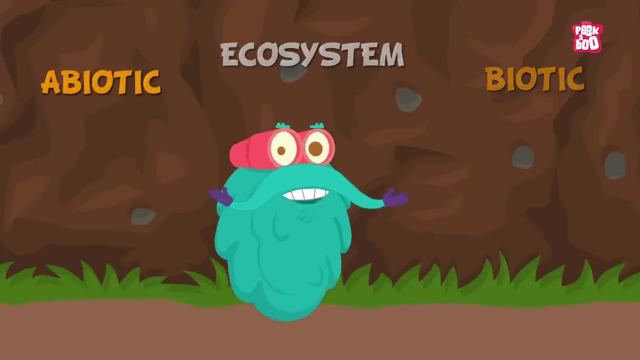 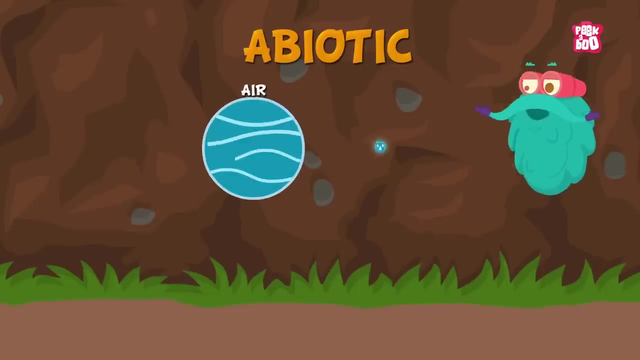 An ecosystem could be a pond, could be your house as well, and some believe that our earth is an ecosystem too. Ecosystem includes two major components: biotic and abiotic components. Abiotic components are the non-living elements of the system, such as air, water, sunlight, nutrients and temperature. 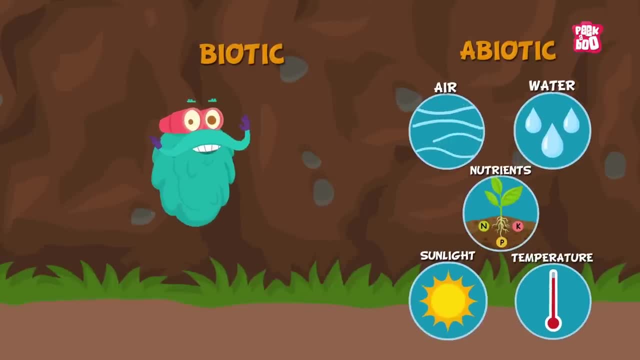 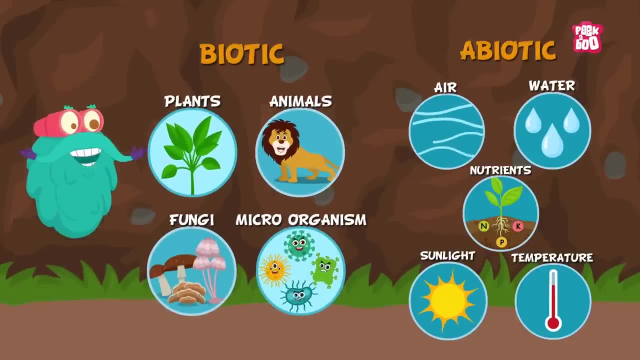 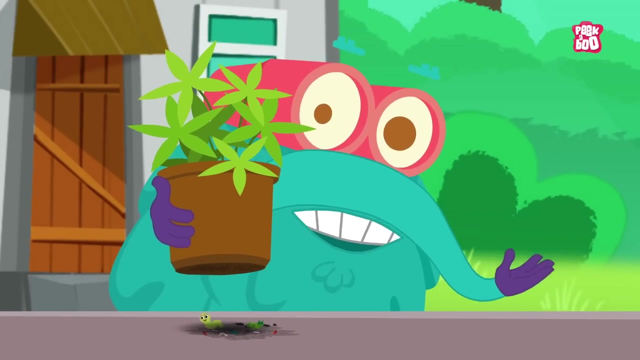 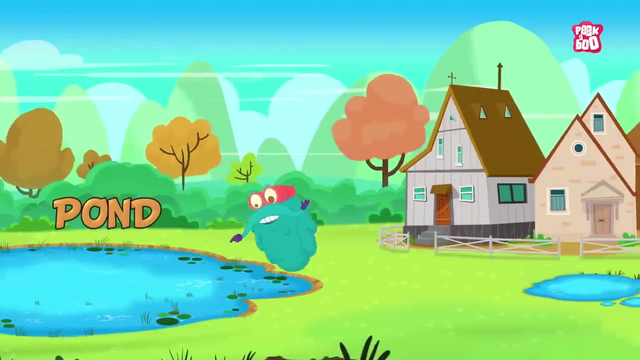 Biotic component are all the living organisms living in the system, like plants, animals, fungi, microorganisms and you. Ecosystems can be of any size, The area under your plant pot, under this rock, a pond, a puddle. 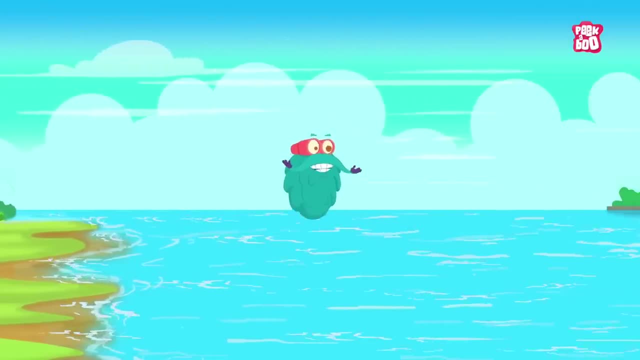 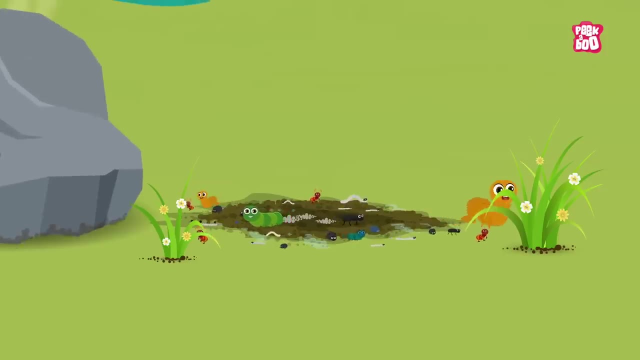 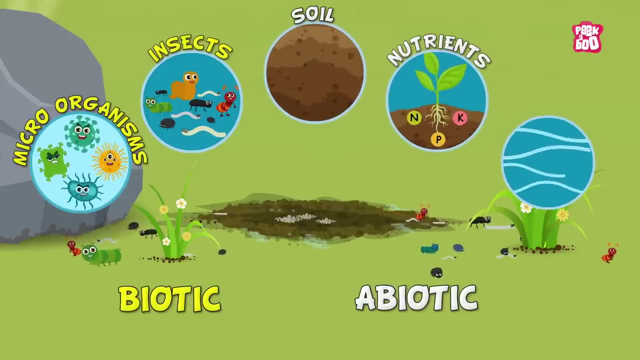 the vast ocean, the city you live in or your country. Take the area under a rock, for example. In this ecosystem you'll find biotic components like the microorganisms, insects, and abiotic components like soil, nutrients, air, etc. 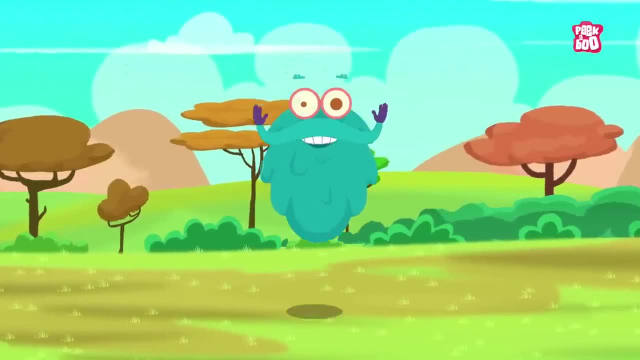 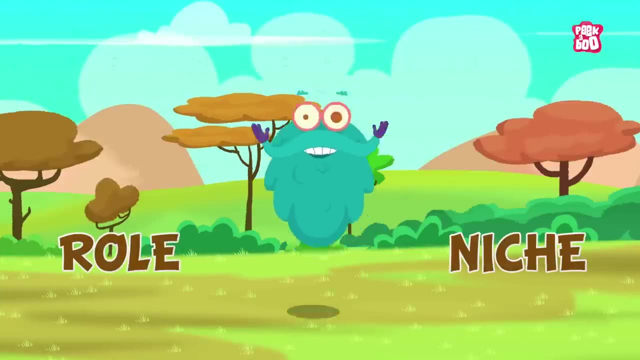 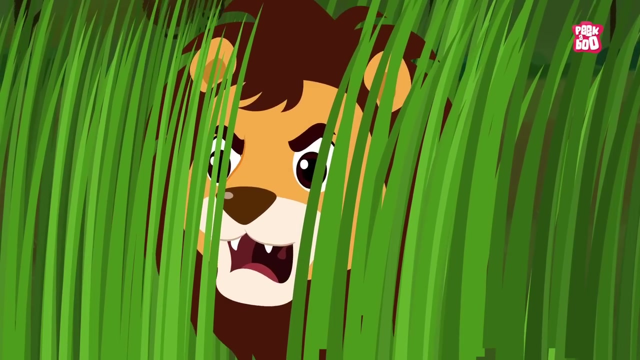 Now, this is an important piece of information. Each organism living in an ecosystem has a role or need. For example, a deer living in a forest is a prey. Lions, tigers, coyotes and other animals eat them for food. Now imagine: 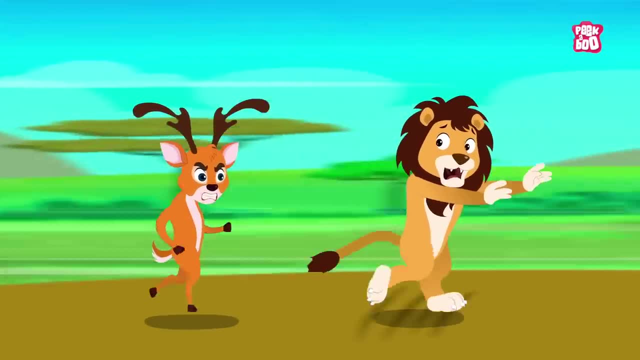 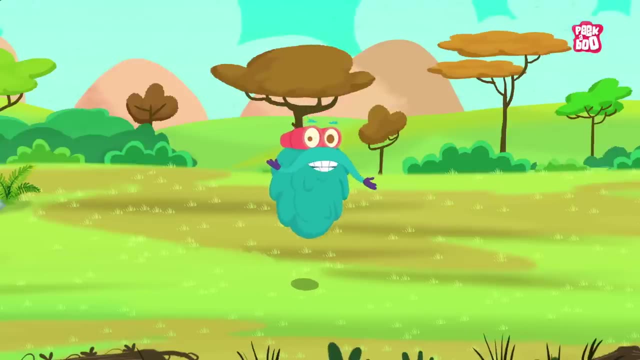 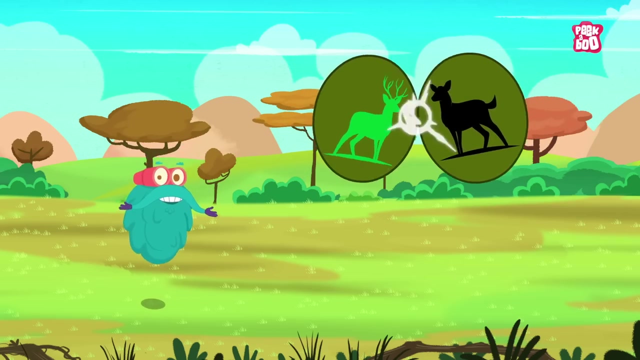 if a deer was supposed to eat lions, coyotes and wolves, wouldn't that make things difficult for an ecosystem? Hmm, we must remember that no two organisms can have the same niche for too long. After a while, one has to either leave or go extinct. 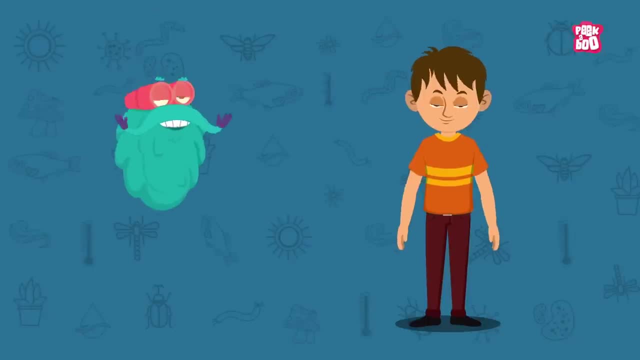 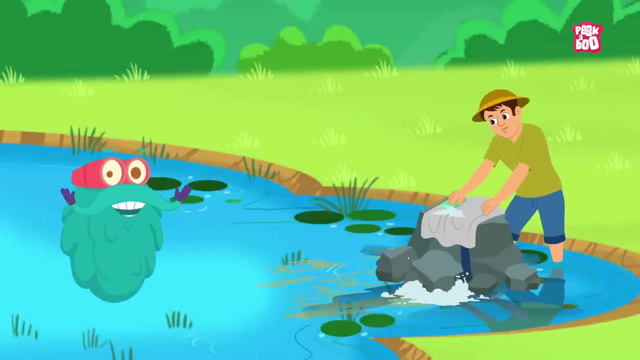 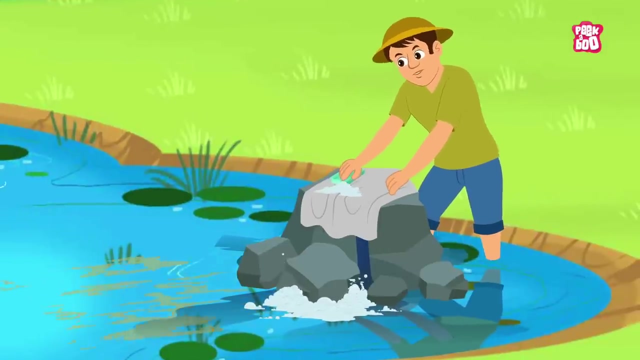 Trivia Time. Did you know that even you are an ecosystem? Yes, you are an ecosystem to the thousands of microorganisms that inhabit you. Our ecosystem is really important. If we keep polluting our ecosystem like that, we would soon go extinct and Earth wouldn't be a habitable ecosystem ever. 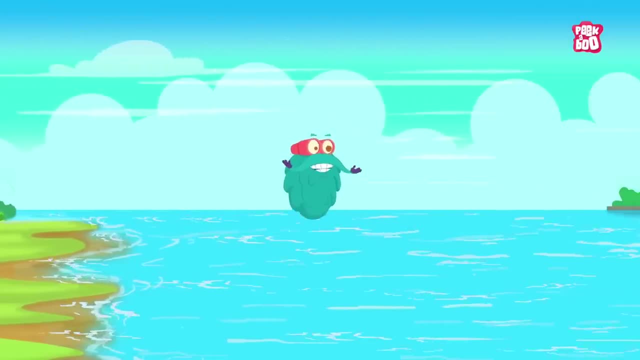 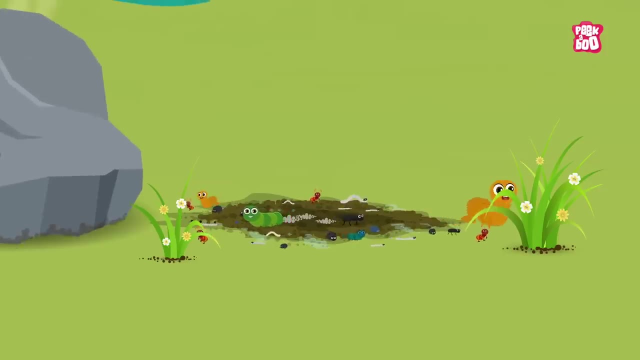 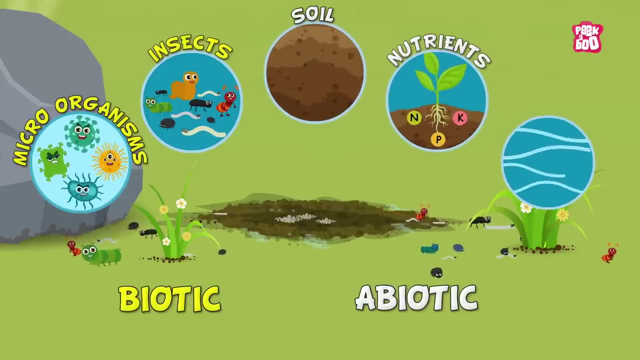 the vast ocean, the city you live in or your country. Take the area under a rock, for example. In this ecosystem you'll find biotic components like the microorganisms, insects, and abiotic components like soil, nutrients, air, etc. 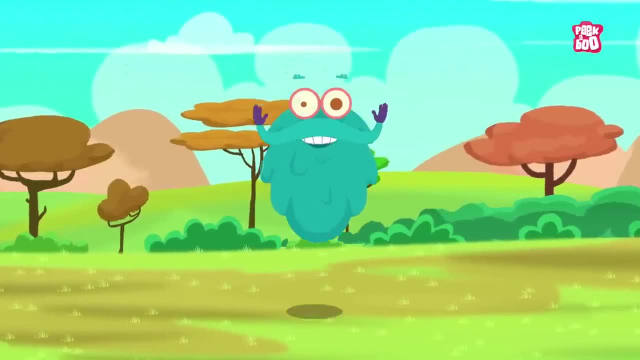 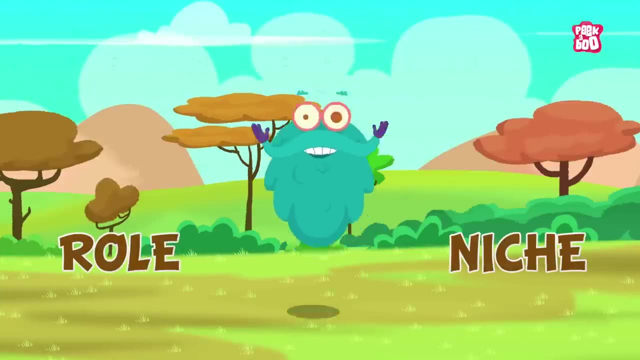 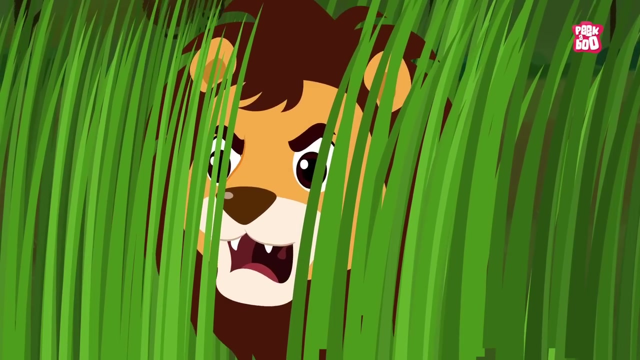 Now, this is an important piece of information. Each organism living in an ecosystem has a role or need. For example, a deer living in a forest is a prey. Lions, tigers, coyotes and other animals eat them for food. Now imagine: 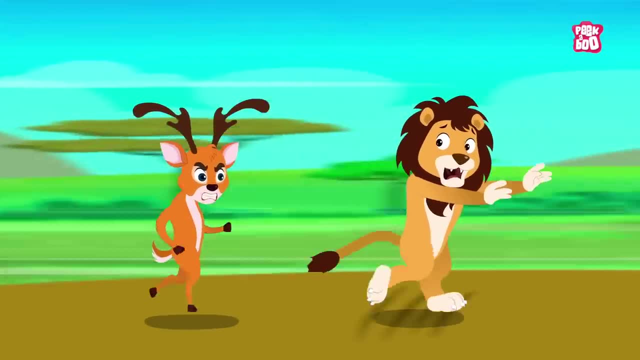 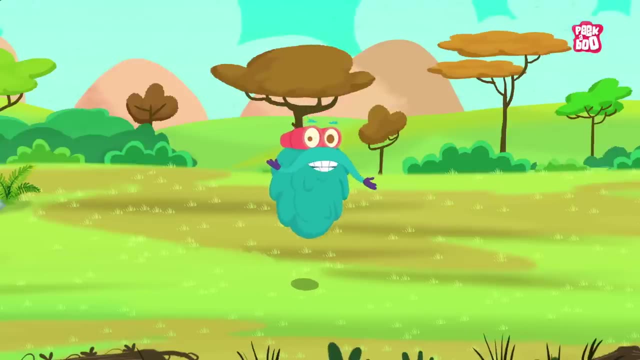 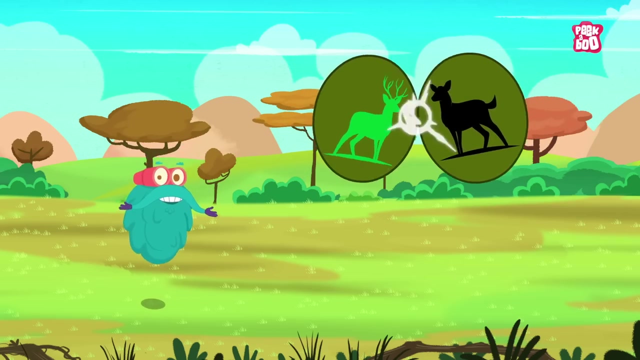 if a deer was supposed to eat lions, coyotes and wolves, wouldn't that make things difficult for an ecosystem? Hmm, we must remember that no two organisms can have the same niche for too long. After a while, one has to either leave or go extinct. 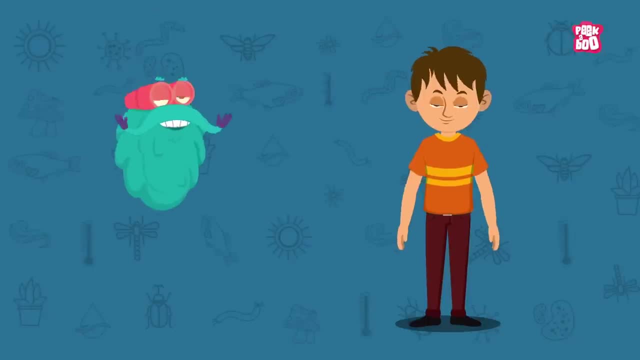 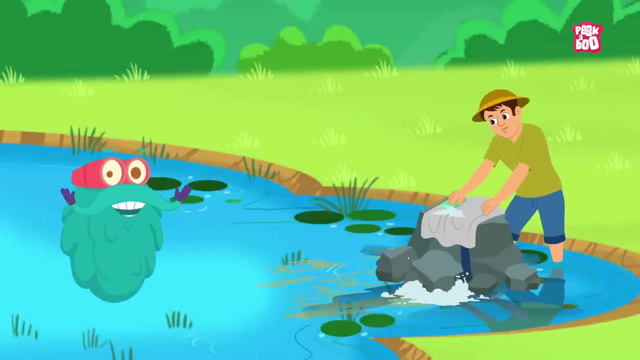 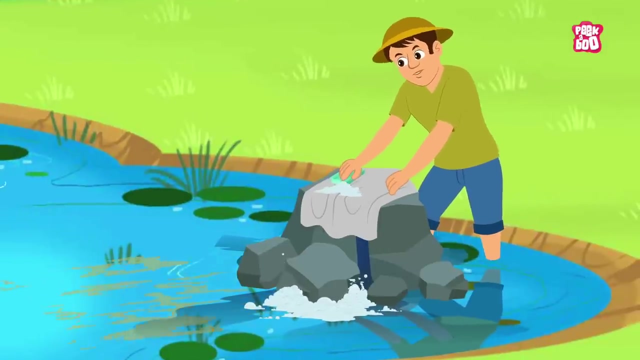 Trivia Time. Did you know that even you are an ecosystem? Yes, you are an ecosystem to the thousands of microorganisms that inhabit you. Our ecosystem is really important. If we keep polluting our ecosystem like that, we would soon go extinct and Earth wouldn't be a habitable ecosystem ever. 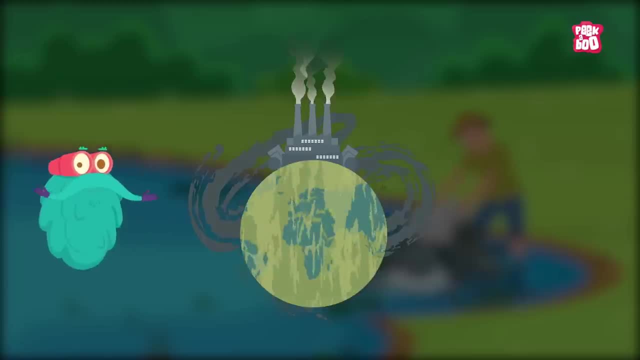 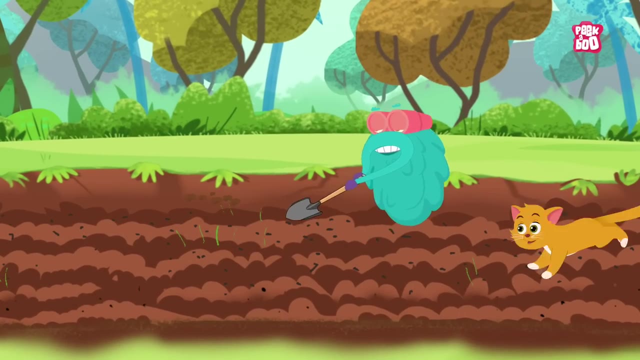 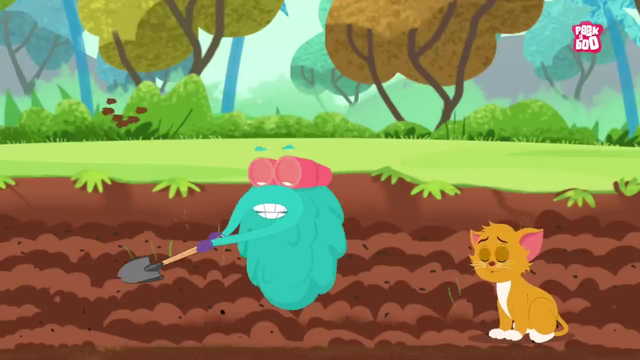 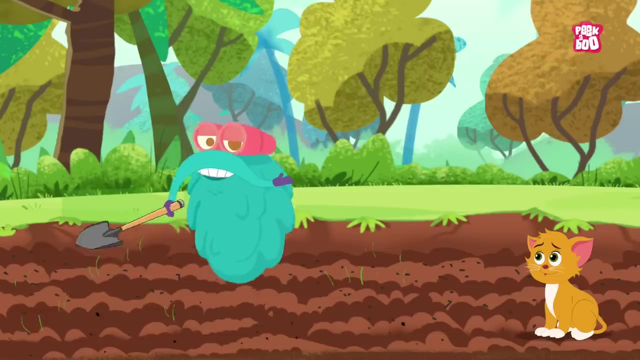 On this note. this is me zooming out. Tune in next time for more fun facts. What, Dr Dweck? Oh, little kitty, I am making arrangements for soil conservation. Soil conservation, What? Ha, ha, ha ha, It's soil conservation kitty. 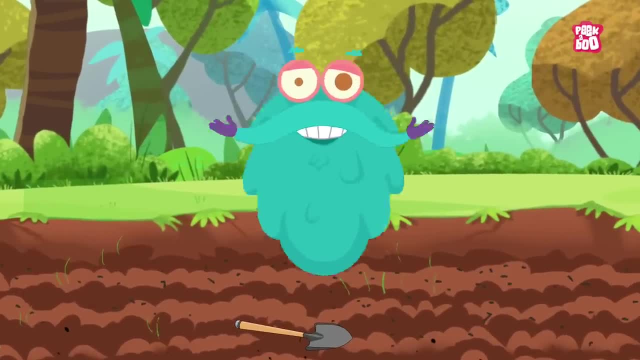 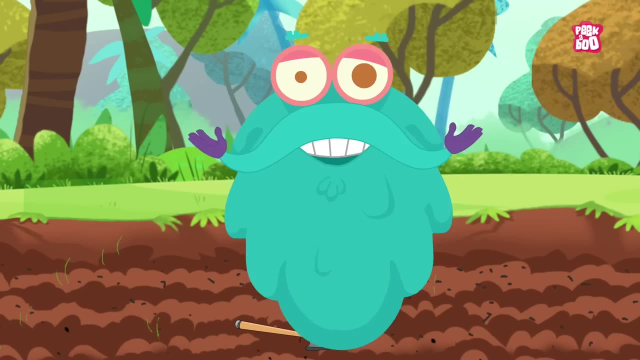 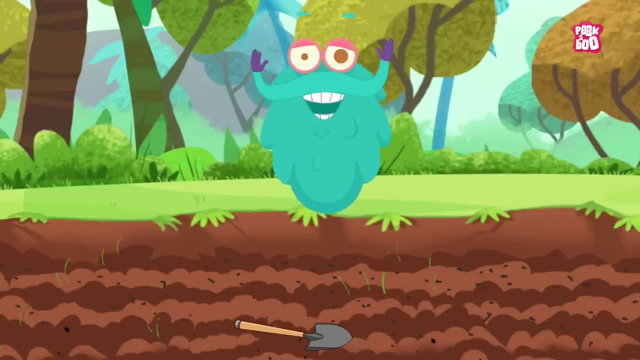 Hey friends, in today's episode, let us learn about one of the most crucial practices we must undertake, known as soil conservation, And learn about its importance, causes and methods by answering a world saving question: What is soil conservation? Zoom in. 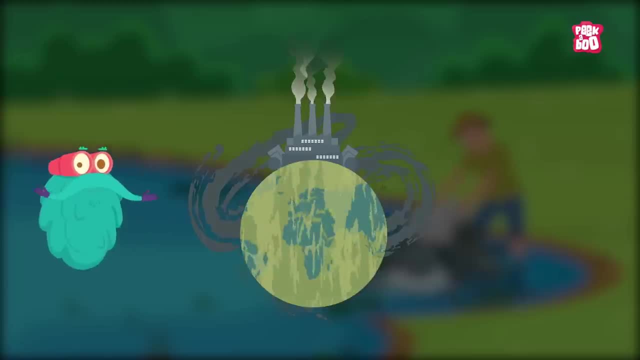 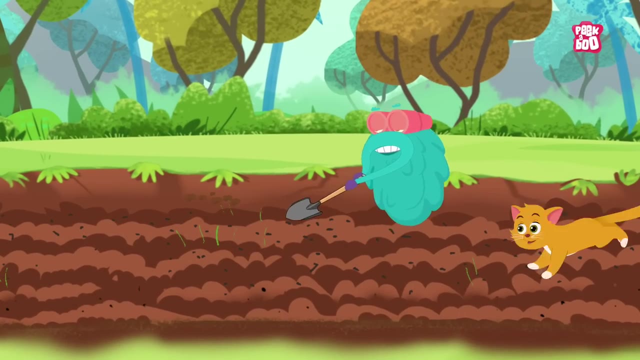 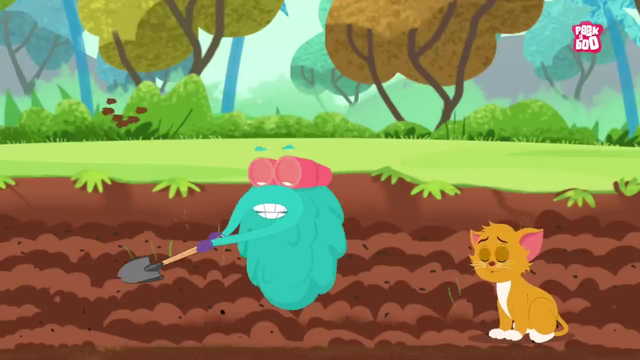 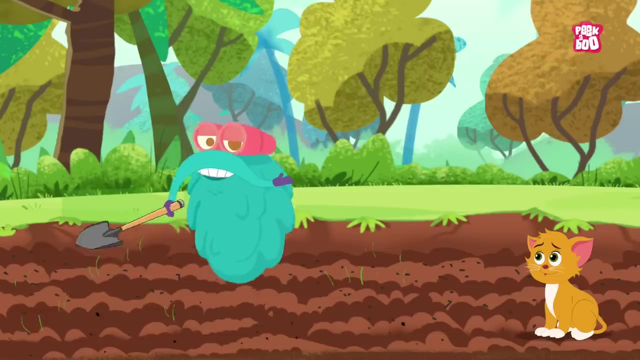 On this note. this is me zooming out. Tune in next time for more fun facts. What, Dr Dweck? Oh, little kitty, I am making arrangements for soil conservation. Soil conservation, What? Hahaha, it's soil conservation kitty. 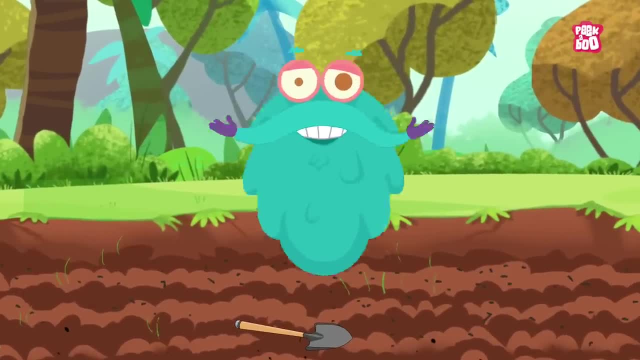 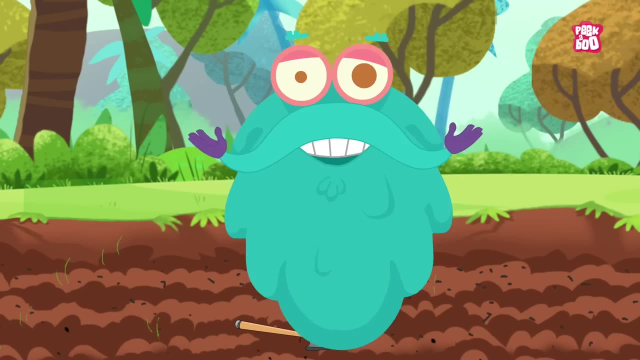 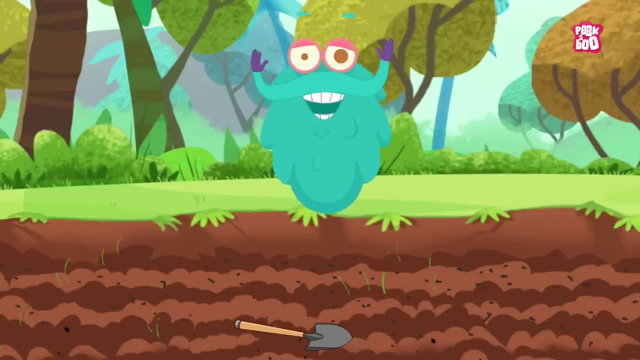 Hey friends, in today's episode, let us learn about one of the most crucial practices we must undertake, known as soil conservation, and learn about its importance, causes and methods by answering a world saving question: What is soil conservation? Zoom in. 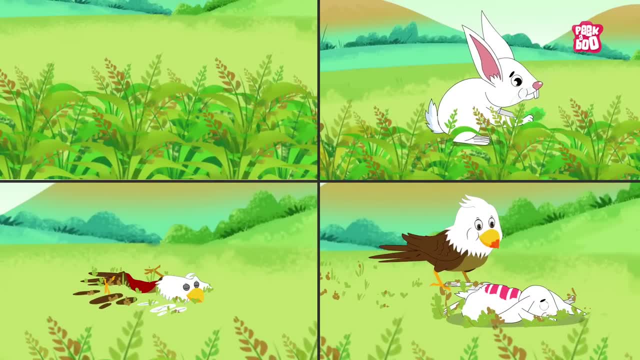 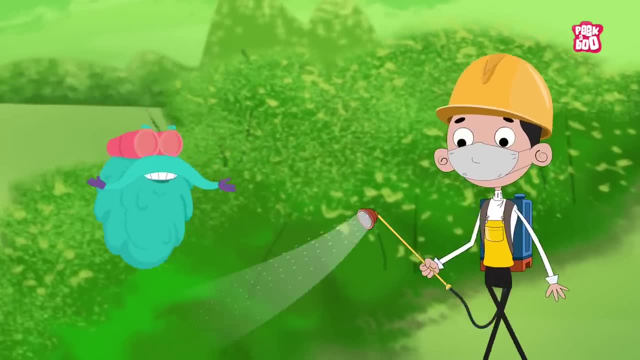 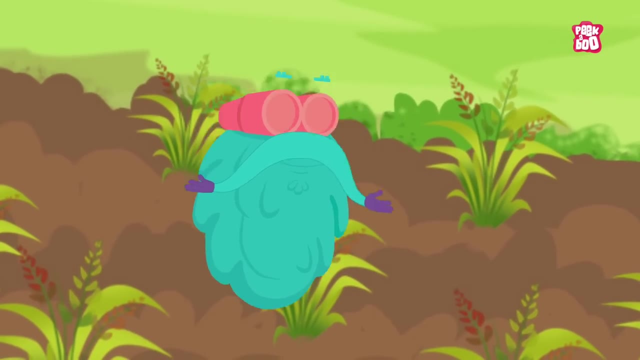 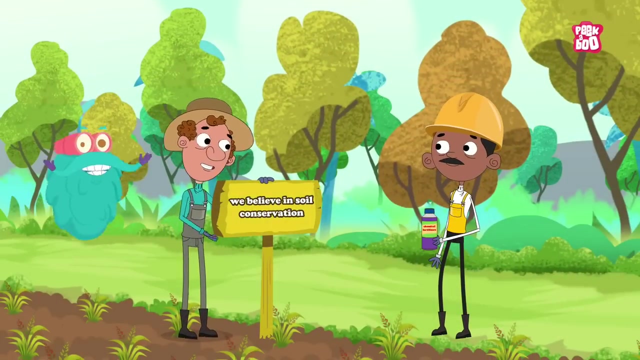 Nature works in a cycle and everything around us is interdependent. But this dependency sometimes proves harmful to many vital natural resources, And one of these resources is soil, whose quality is degrading with passing time. So to stop this degradation of soil, 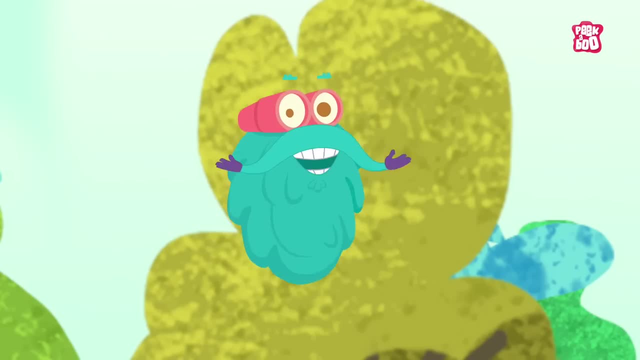 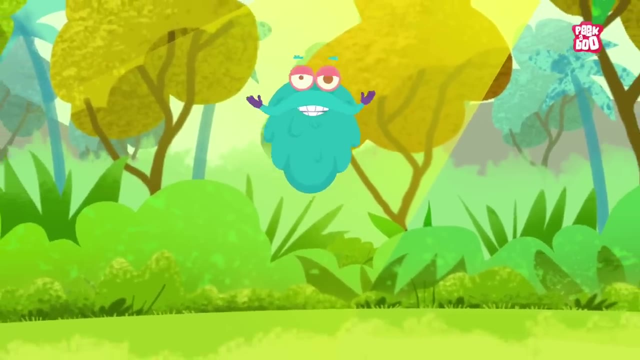 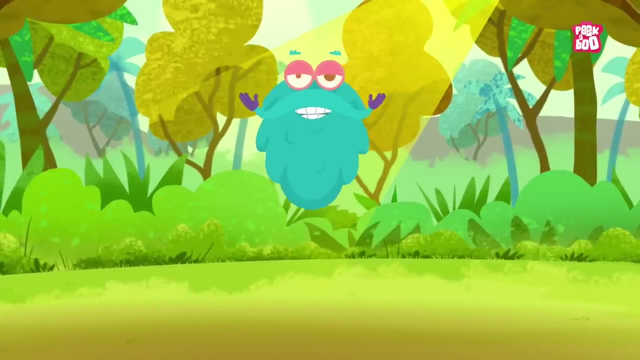 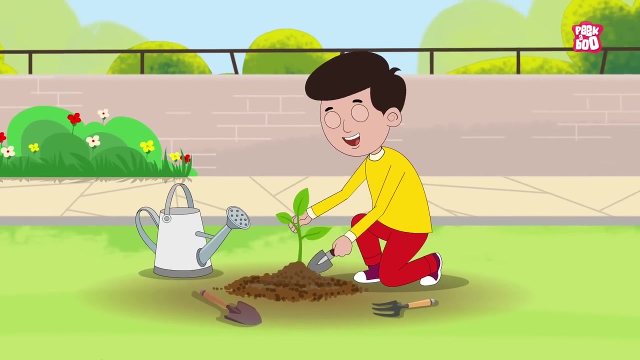 soil conservation is essential. Soil conservation is exercised, And what is that? Well, conservation is the act of saving or protecting a resource, And soil conservation is a practice that helps to retain and maintain the quality of the soil by preventing soil erosion through planting new plants. 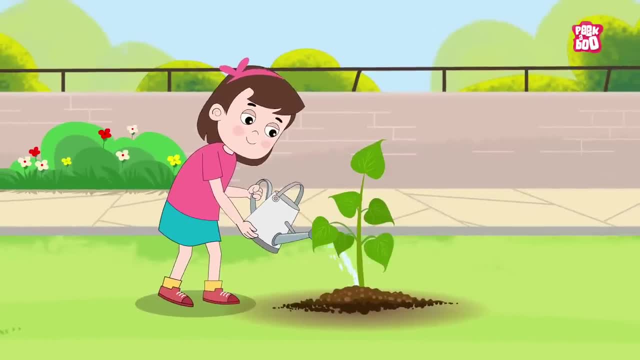 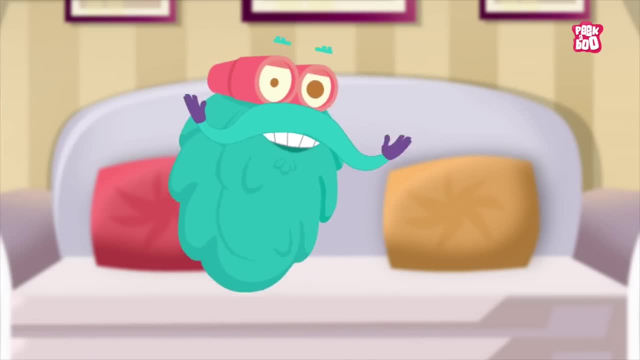 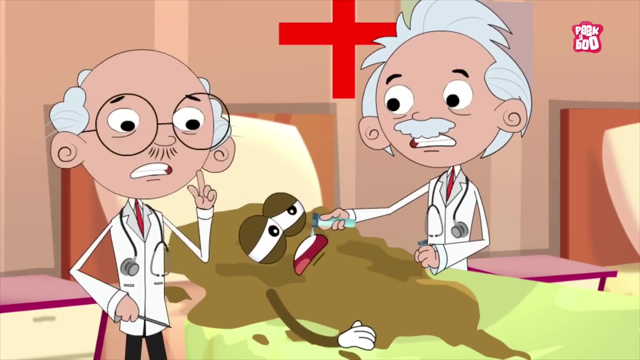 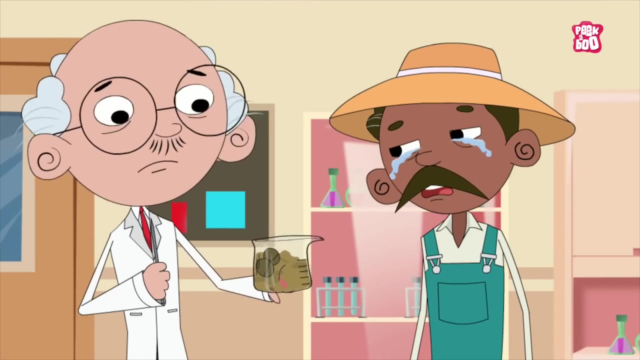 taking care of plants or keeping soil from being contaminated. But the crucial question is: why is it required in the first place? Well, soil conservation is necessary because if we run out of healthy soil, we won't be able to carry out agricultural and planting activities. 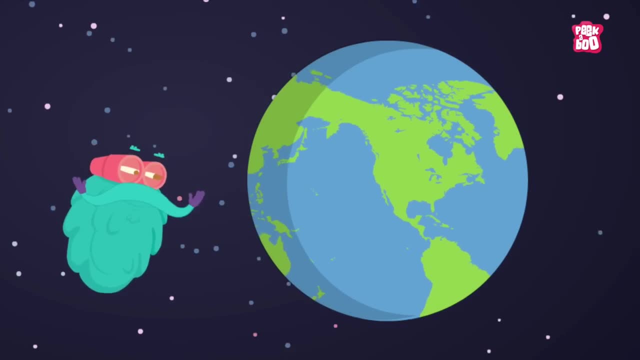 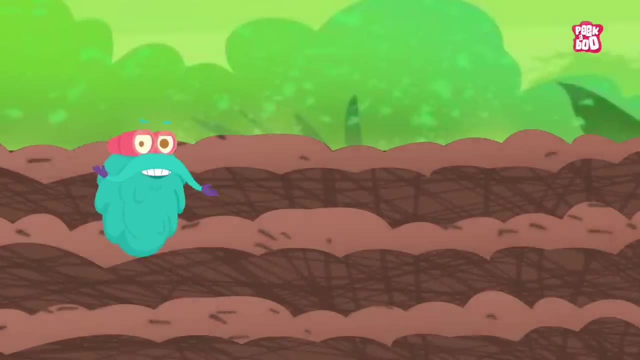 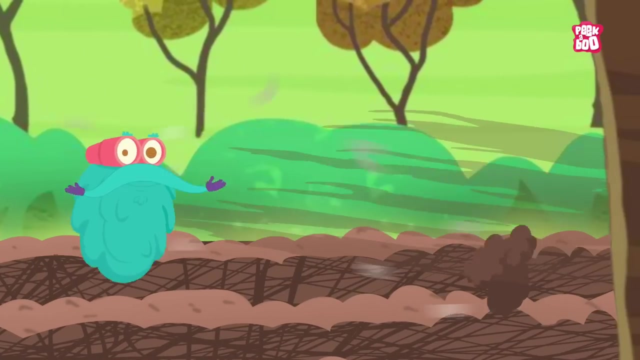 that are necessary to feed all of the living beings on earth And, unfortunately, in recent times, the quality of soil has been degrading at an alarming rate due to many human and natural activities, through a process called soil erosion. And what is that? 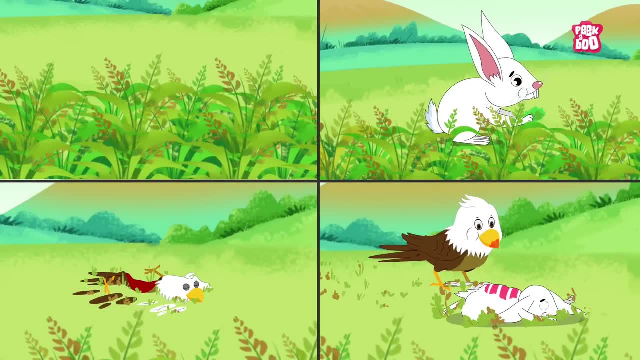 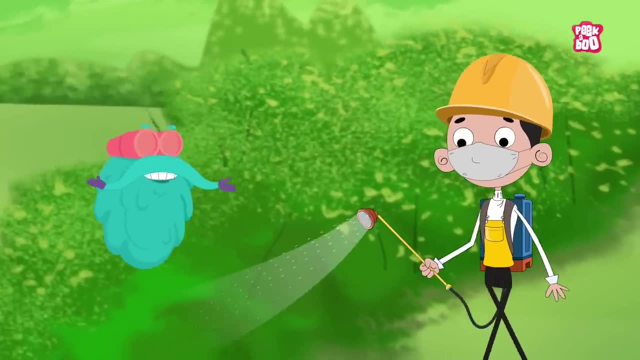 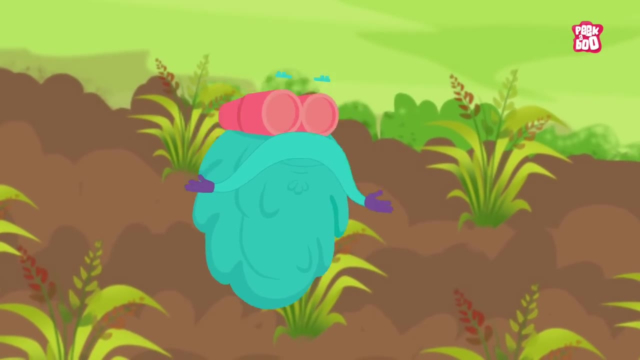 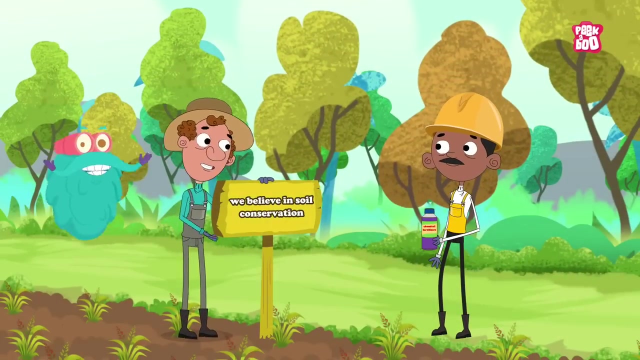 Nature works in a cycle and everything around us is interdependent, But this dependency sometimes proves harmful to many vital natural resources, And one of these resources is soil, whose quality is degrading with passing time. So to stop this degradation of soil, soil conservation is essential. 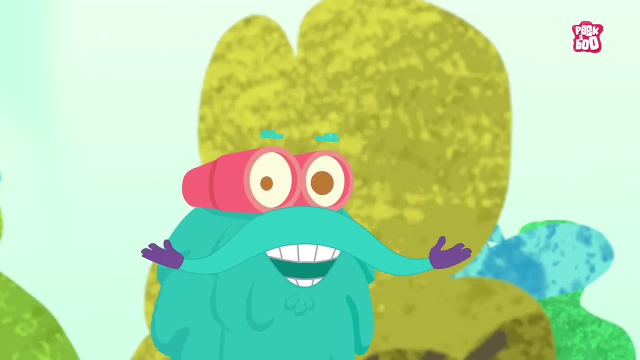 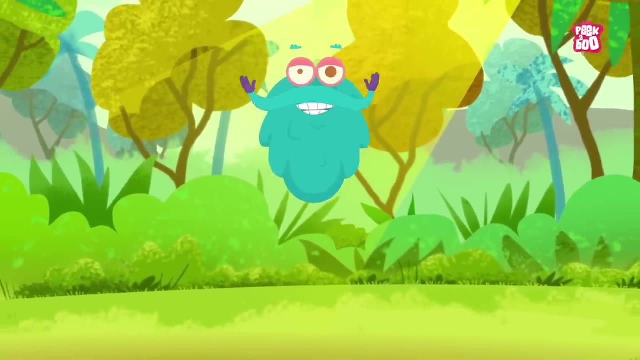 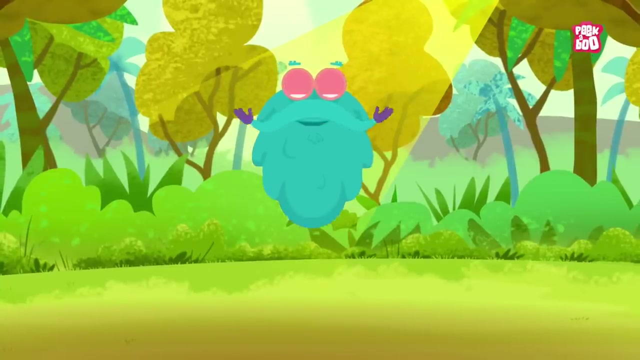 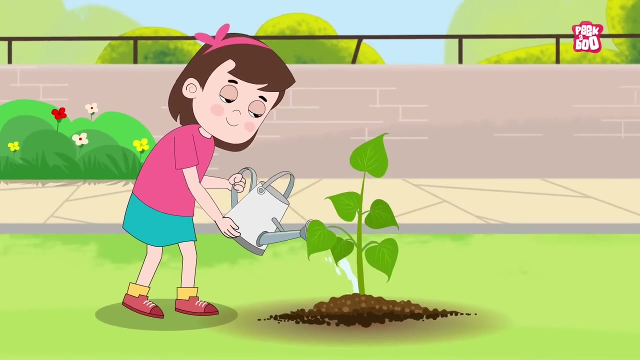 Soil conservation is exercised. And what is that? Well, conservation is the act of saving or protecting a resource, And soil conservation is a practice that helps to retain and maintain the quality of the soil by preventing soil erosion through planting new plants, taking care of plants or keeping soil from being contaminated. But the crucial question is: why is it required in the first place? Well, soil conservation is necessary because if we run out of healthy soil, we won't be able to carry out agricultural and planting activities that are necessary to feed all of the living beings on earth. 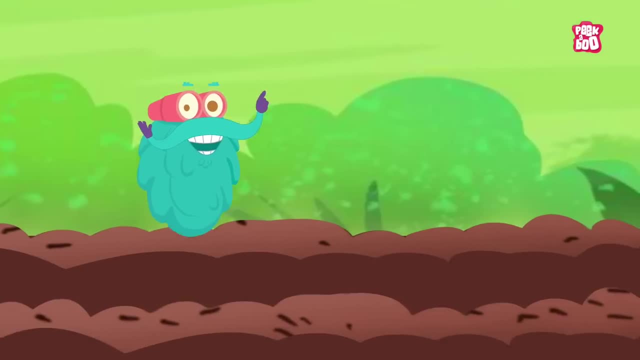 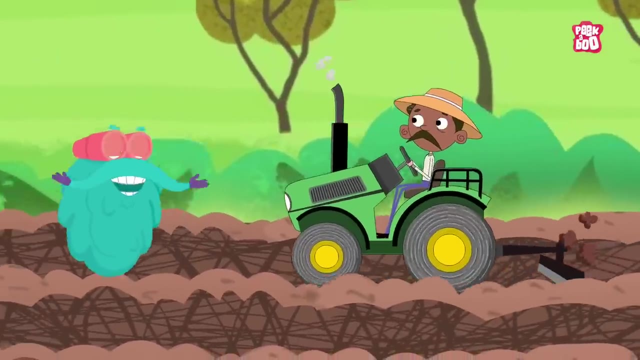 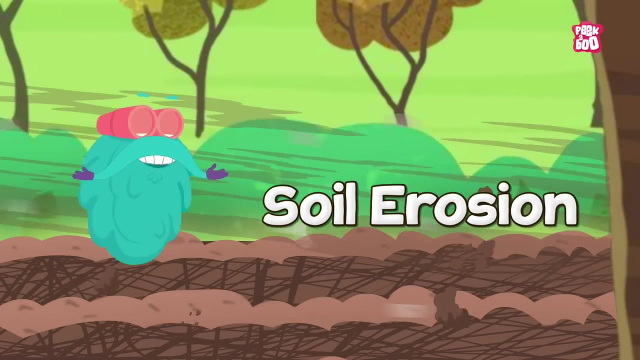 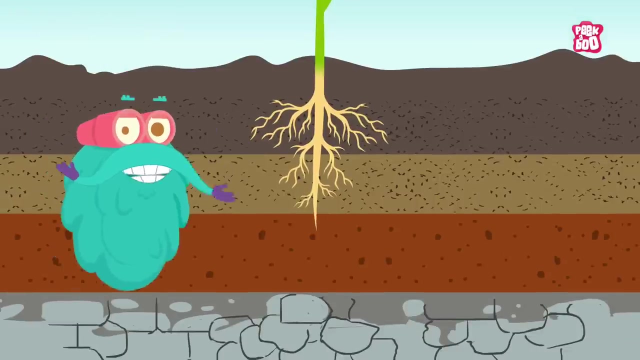 And, unfortunately, in recent times, the quality of soil has been degrading at an alarming rate due to many human and natural activities through a process called soil erosion. And what is that? Soil erosion is a process in which the topsoil of a field containing the highest number of nutrients 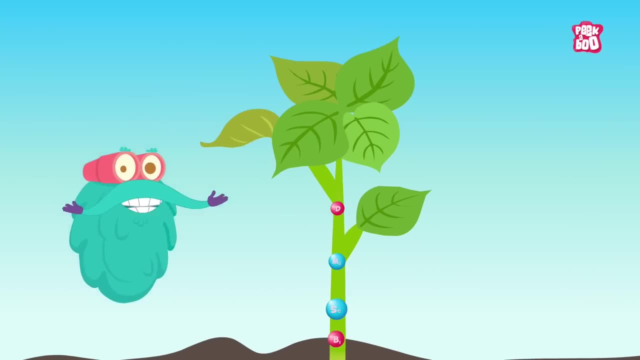 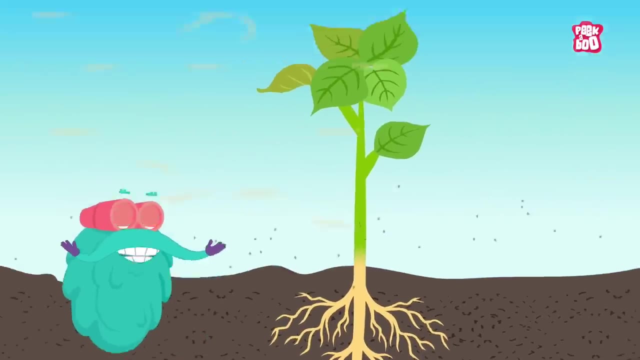 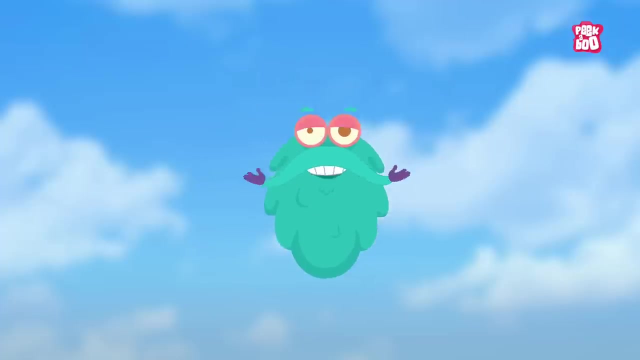 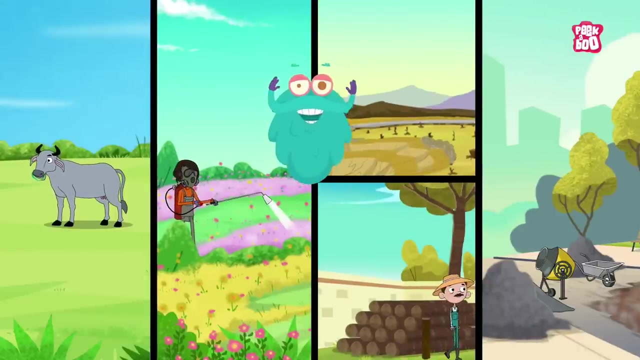 microorganisms and minerals vital for plant growth is washed away from one place to another by natural sources such as wind and water. Not only that, but aggressive human activities such as overgrazing of cattle, overuse of pesticides, mining and logging, construction of roads and buildings. 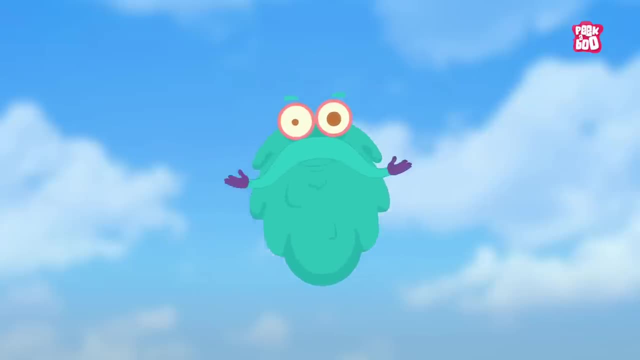 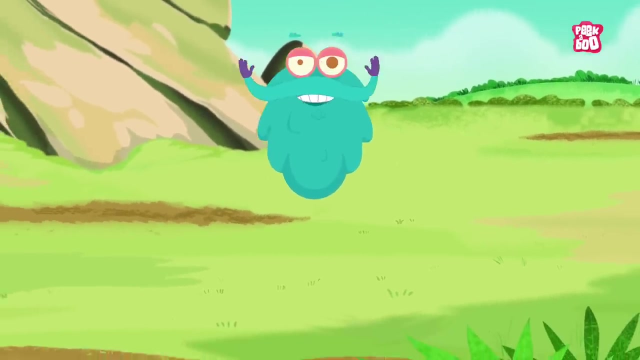 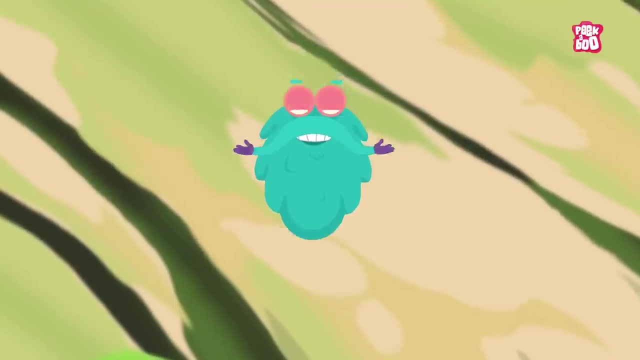 have fastened the process of soil erosion, So the need for soil conservation has increased more than ever before. But the vital question is: what can we do to save the soil? Well, there are various methods we can undertake for it. Let's have a look at some of them. 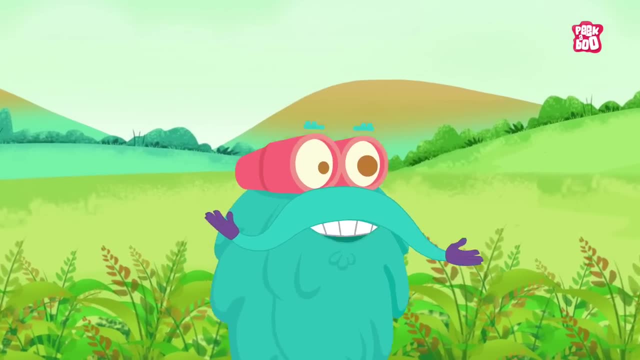 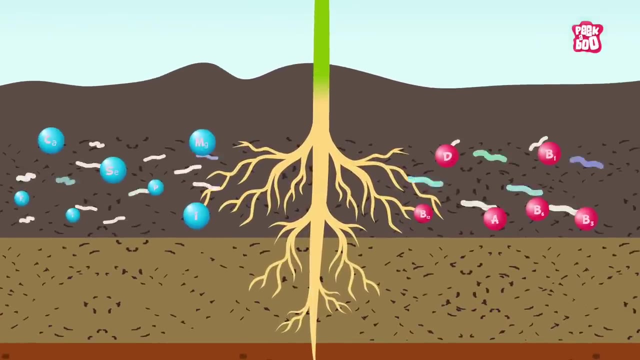 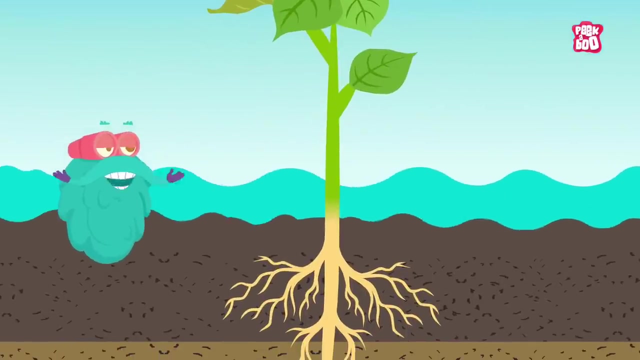 Soil erosion is a process in which the topsoil of a field containing the highest number of nutrients, microorganisms and minerals vital for plant growth is washed away from one place to another by natural sources such as wind and water. Not only that, 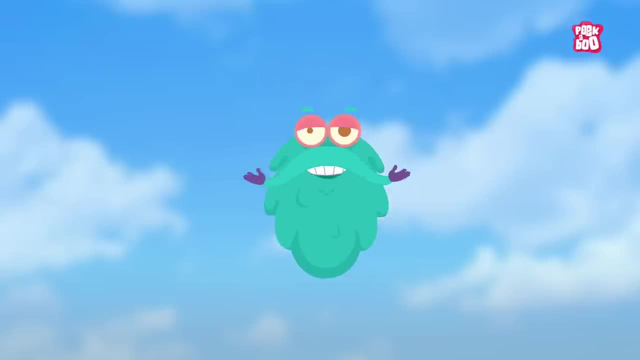 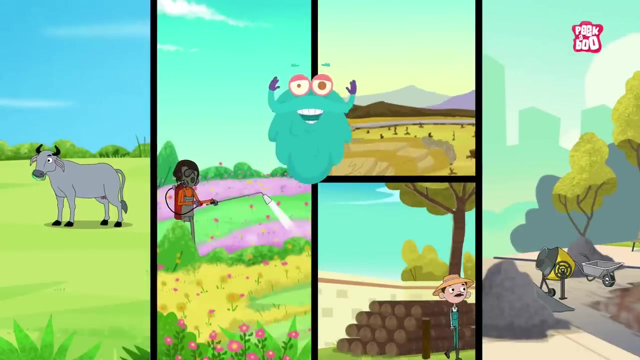 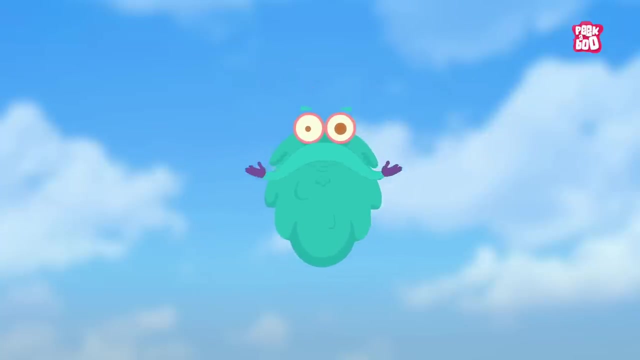 but aggressive human activities such as overgrazing of cattle, overuse of pesticides, mining and logging, construction of roads and buildings have fastened the process of soil erosion, So the need for soil conservation has increased more than ever before. 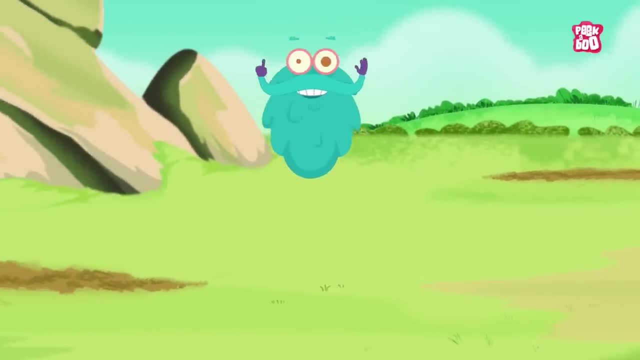 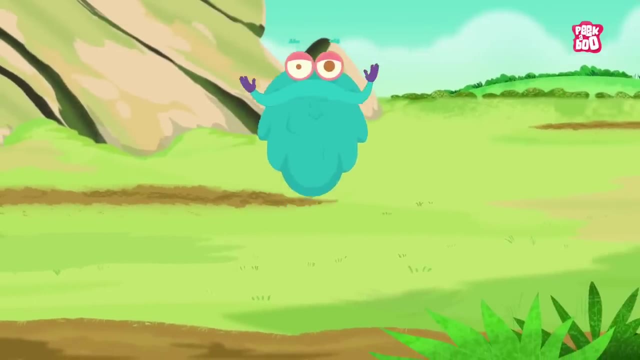 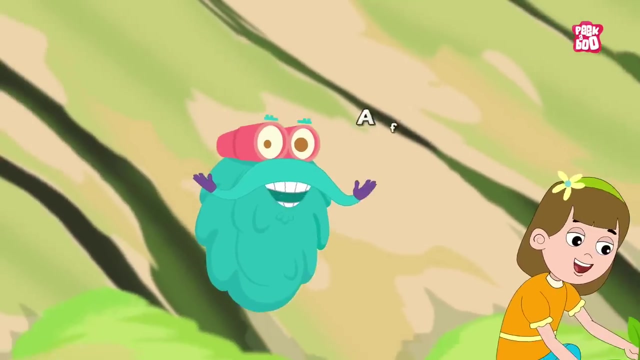 But the vital question is: what can we do to save the soil? Well, there are various methods we can undertake for it. Let's have a look at some of them. First, we must practice earth forestation, in which we can plant new trees and reduce down their cutting. 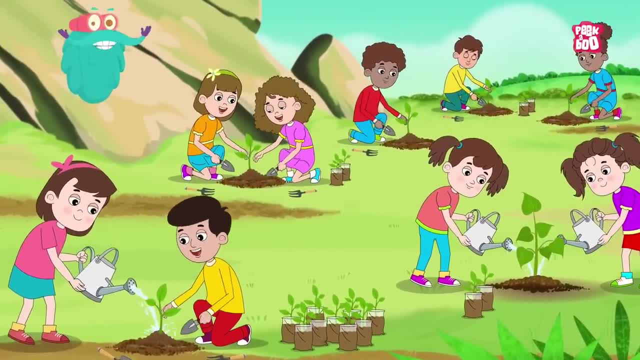 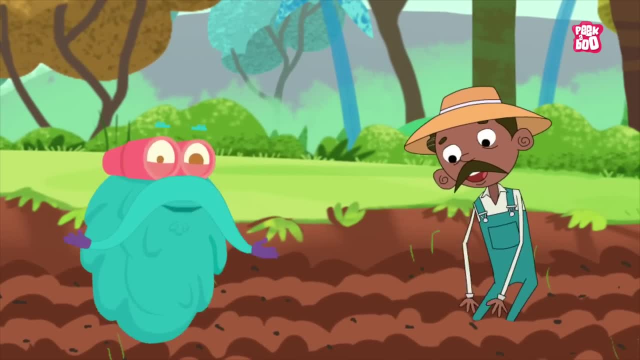 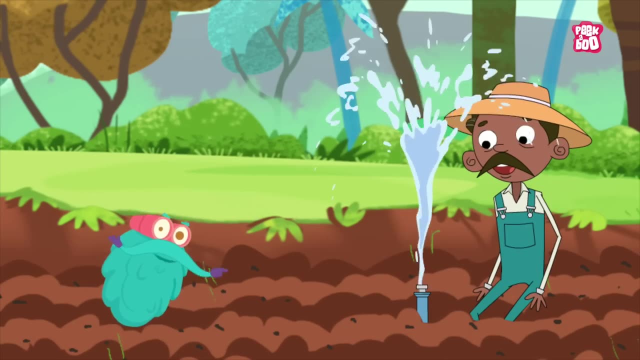 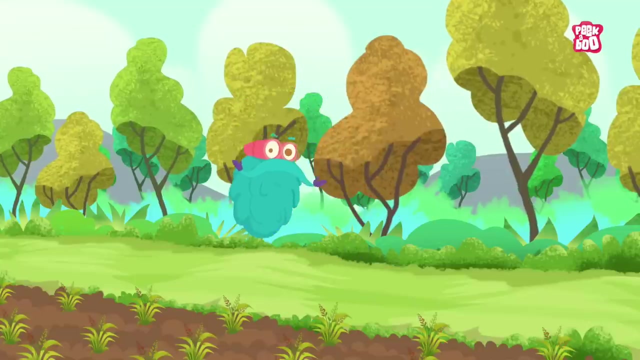 leading to the reduction of soil erosion. The next thing we could do is minimize the use of water during farming and gardening so that it does not wash off the rich and nutrient-filled upper layer of soil. Another vital step we can take is by planting windbreaks. 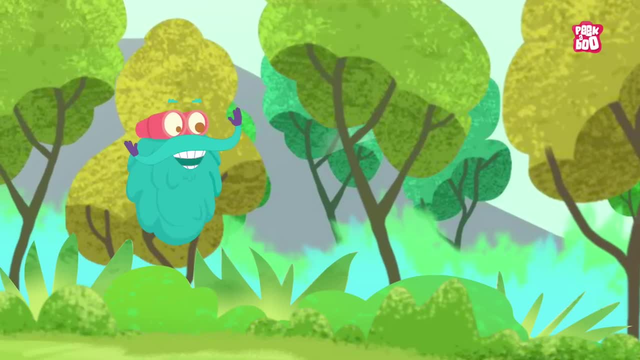 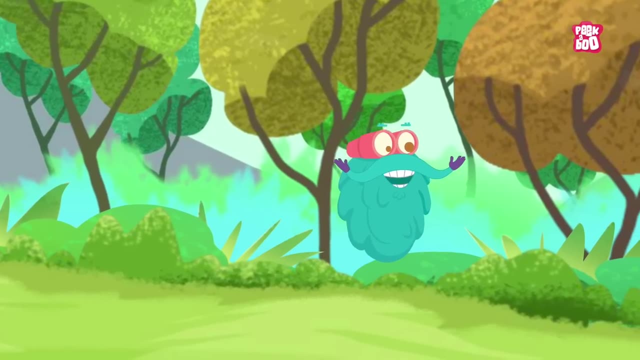 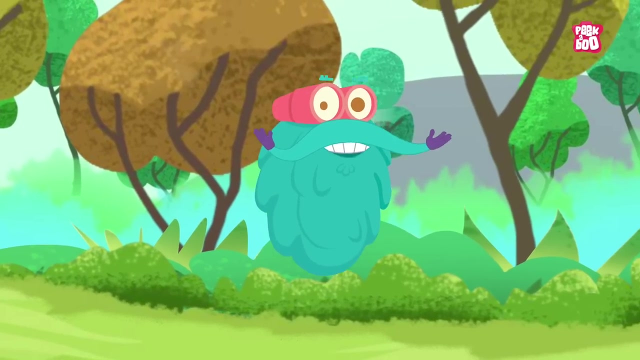 Yes, a windbreak is a line of plants planted to stop or slow the wind. A thick row of bushes planted next to a field of plants can control the wind from blowing the soil away. This system also helps against water erosion, as the soil gets caught up against the roots of the bushes. 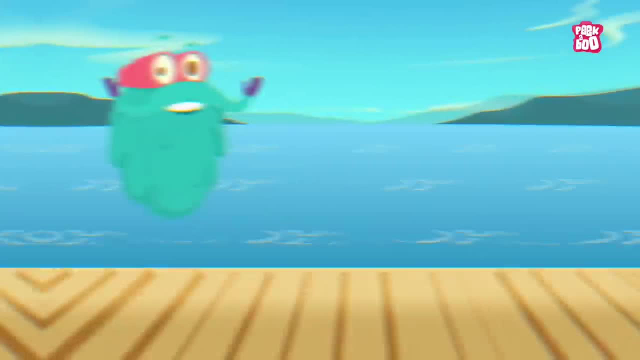 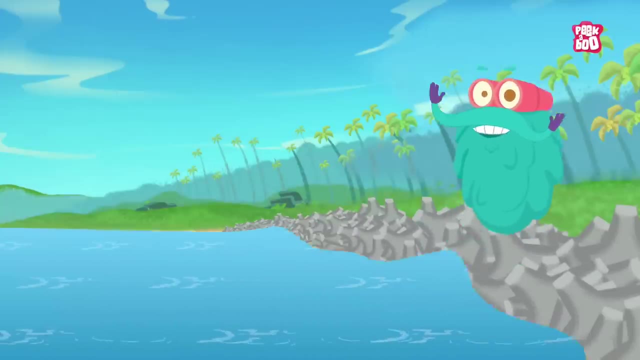 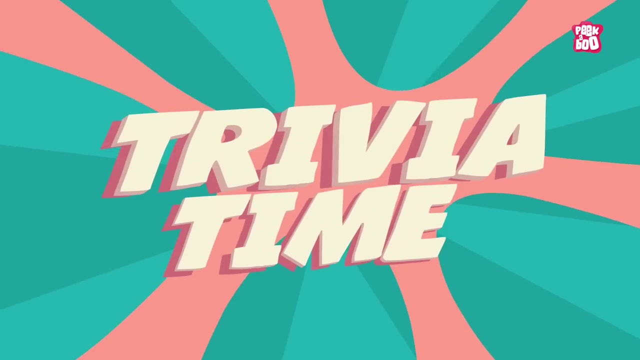 rather than washing away. And lastly, we can put up wooden planks along the beaches or build seawalls against the cliffs to prevent water from eroding the soil. Did you know the word erosion comes from the Latin word. 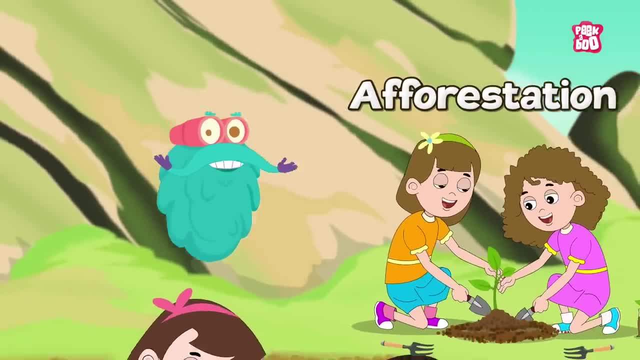 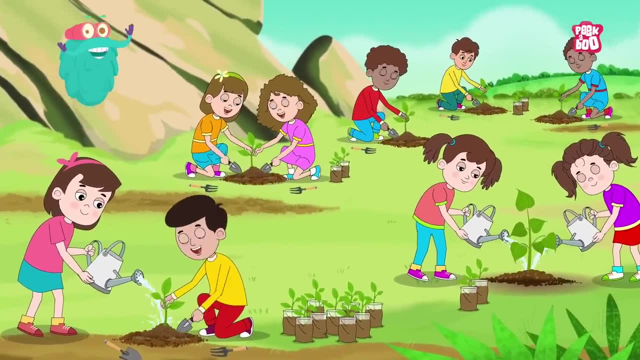 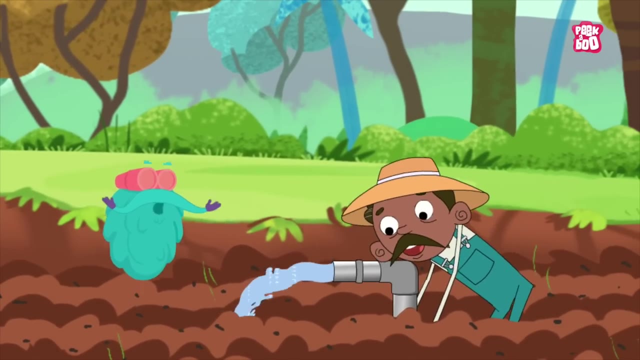 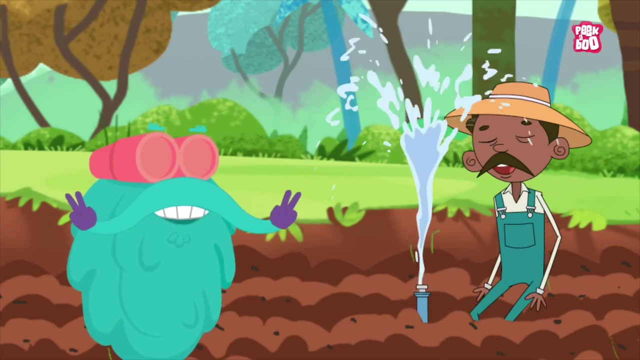 First, we must practice earth forestation, in which we can plant new trees and reduce down their cutting, Leading to the reduction of soil erosion. The next thing we could do is minimize the use of water during farming and gardening, so that it does not wash off the rich and nutrient-filled upper layer of soil. 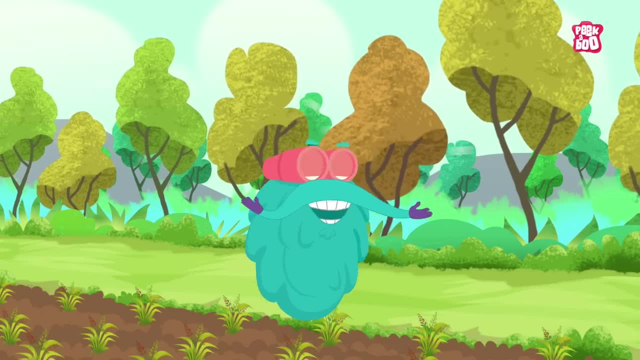 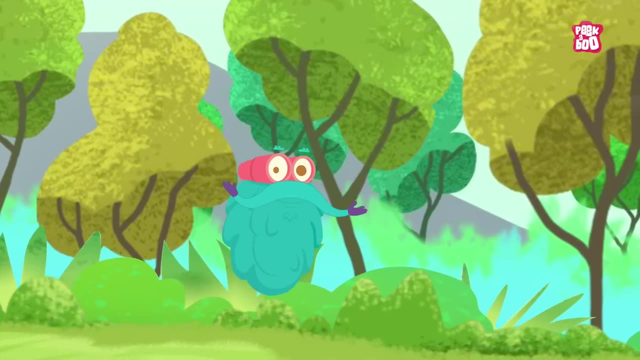 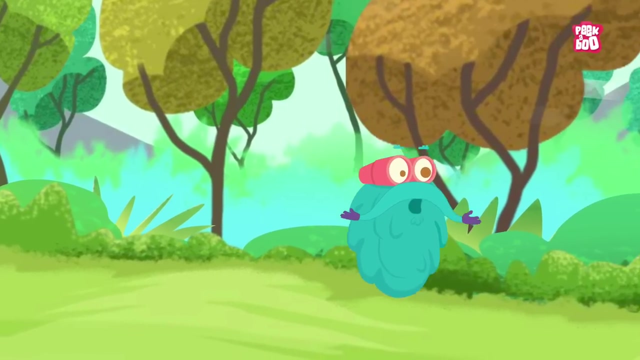 Another vital step we can take is by planting windbreaks. Yes, a windbreak is a line of plants planted to stop or slow the wind. A thick row of bushes planted next to a field of plants can control the wind from blowing the soil away. 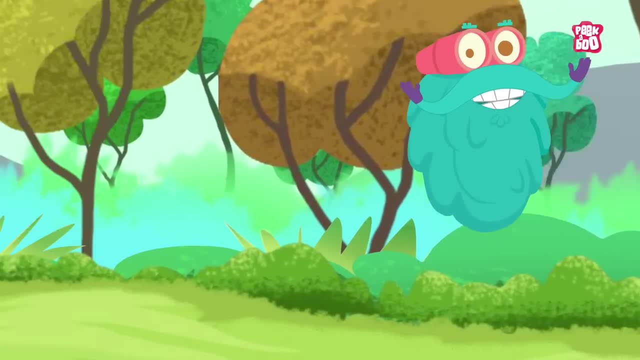 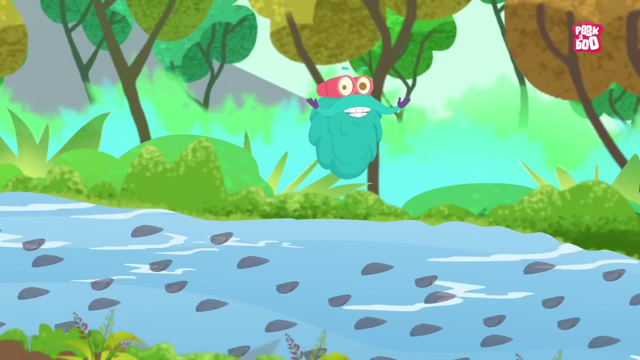 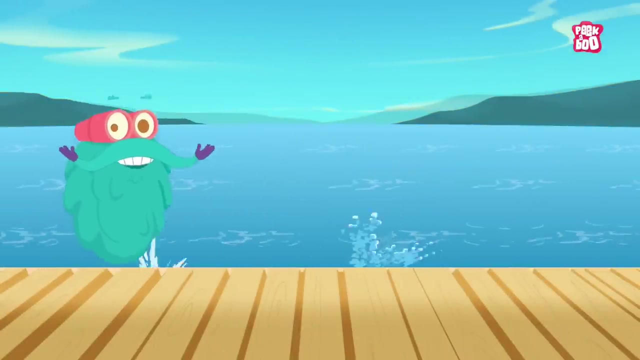 This system also helps against water erosion, as the soil gets caught up against the roots of the bushes rather than washing away. And lastly, we can put up wooden planks along the beaches or build seawalls against the cliffs to prevent water from eroding the soil. 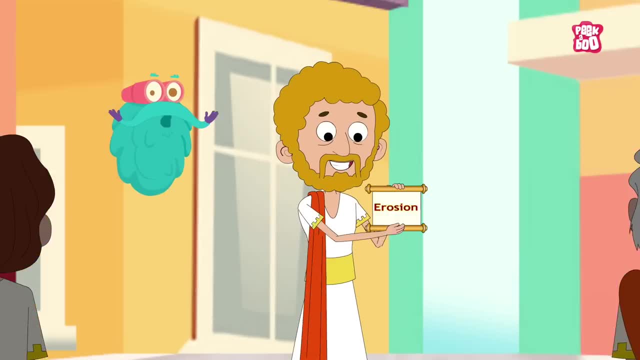 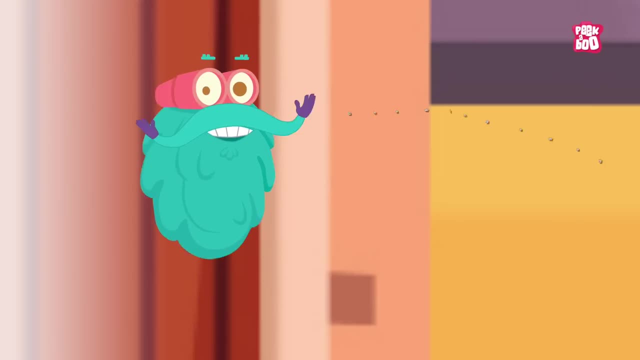 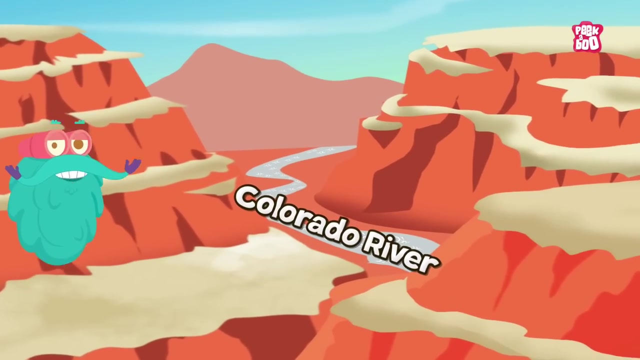 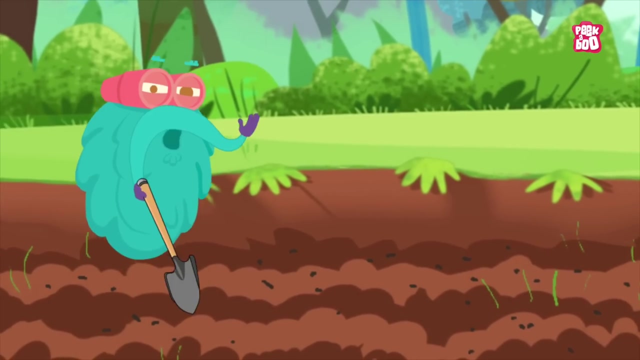 Trivia Time. Did you know the word erosion comes from the Latin word Erosionem, which means gnawing away? Also, scientists estimate that the Colorado River has been eroding the Grand Canyon for many millions of years. Hope you learned something new in today's episode. 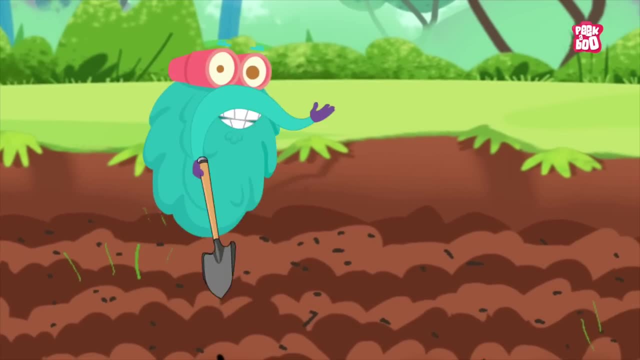 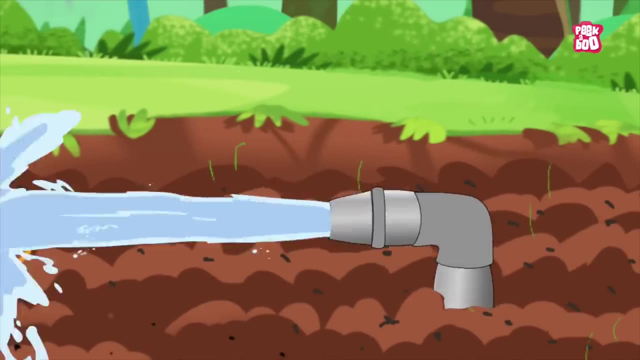 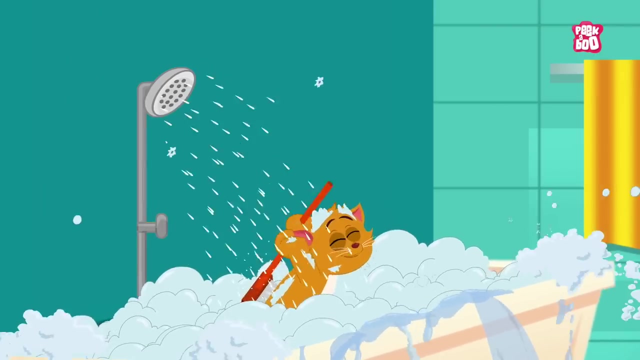 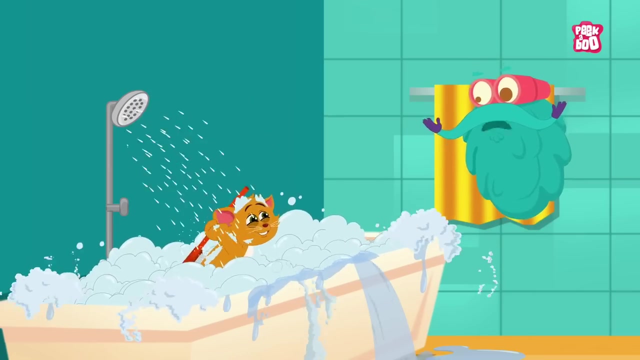 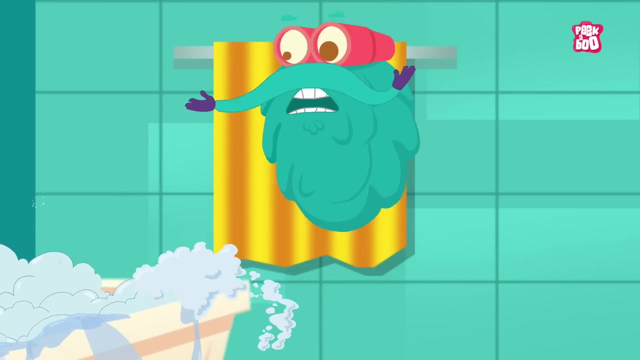 Until next time it's me, Dr Binox, Zooming Out. Ah, never mind. Kitty needs a little help. Well, make sure you don't waste much water or any other natural resources. little kitty, It is vital to save them. 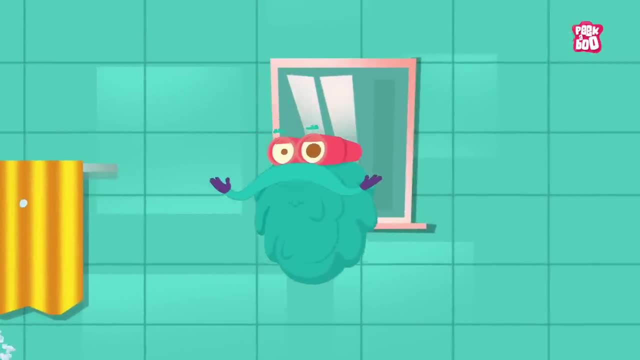 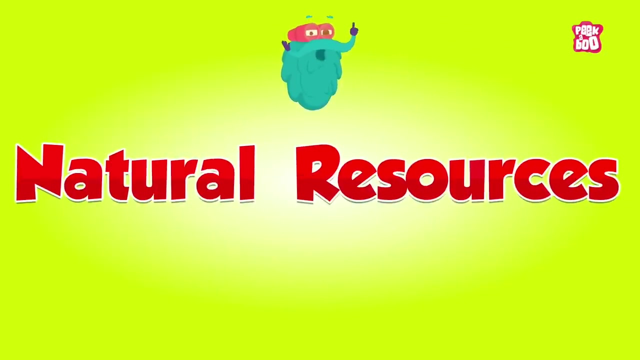 Let me explain. Hey friends, it's a topic we must all learn about, not only to get good grades, but to save the world. So let's zoom in. So what do we mean by the word natural resources? Well, the answer is in the word itself. 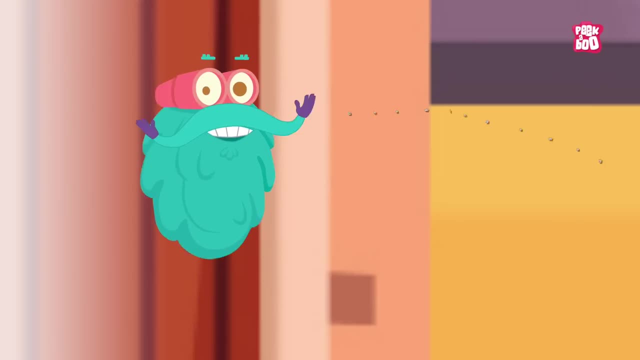 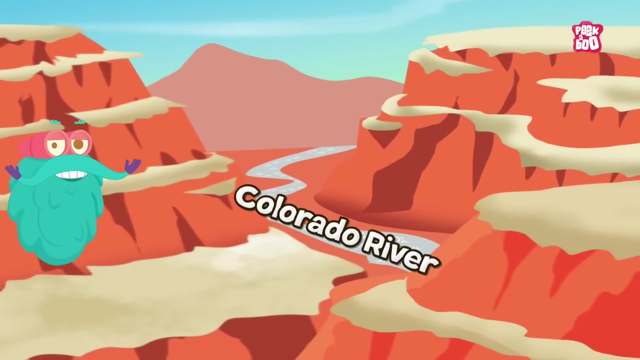 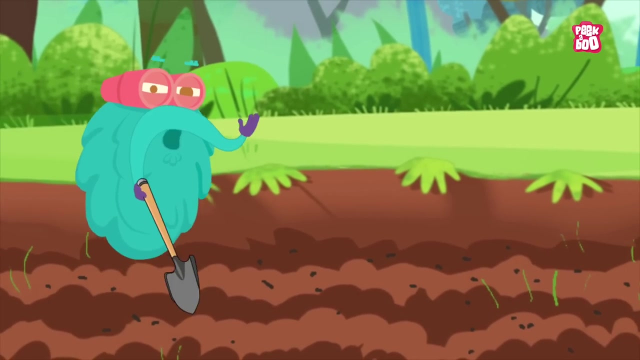 Erosionem, which means gnawing away. Also, scientists estimate that the Colorado River has been eroding the Grand Canyon for many millions of years. Hope you learned something new in today's episode. Until next time. 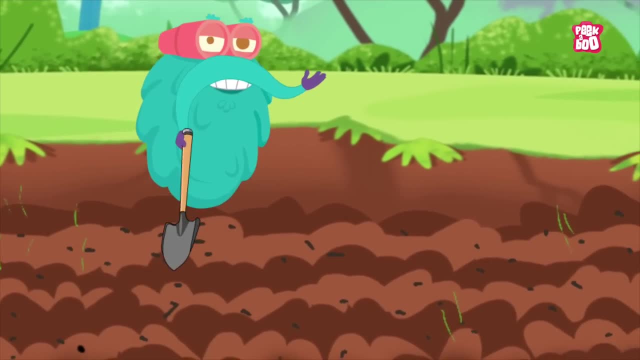 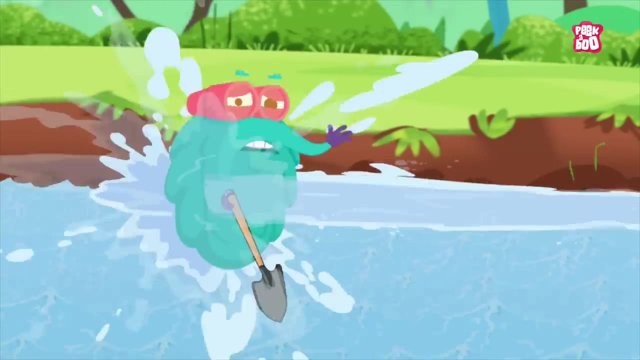 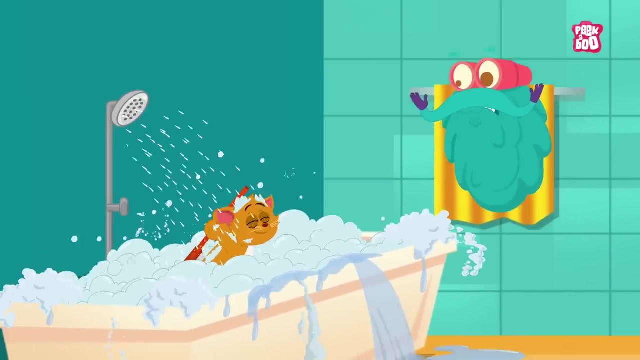 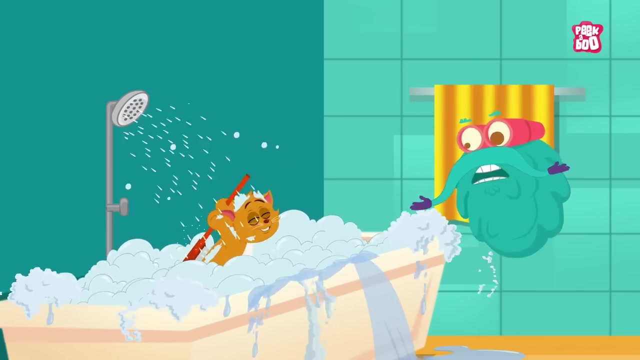 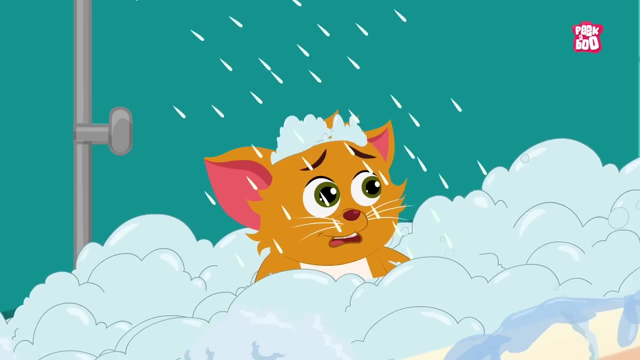 it's me, Dr Binox, Zooming Out. Ah, never mind. Kitty needs a long bath. Well, make sure you don't waste much water or any other natural resources. little kitty, It is vital to save them. Let me explain. 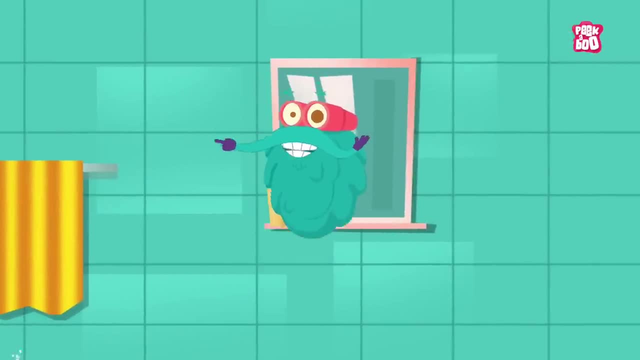 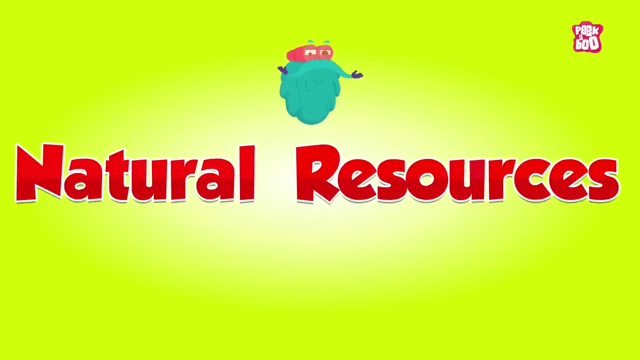 Hey friends, it's a topic we must all learn about, not only to get good grades, but to save the world. So let's zoom in. So what do we mean by the word natural resources? Well, the answer. 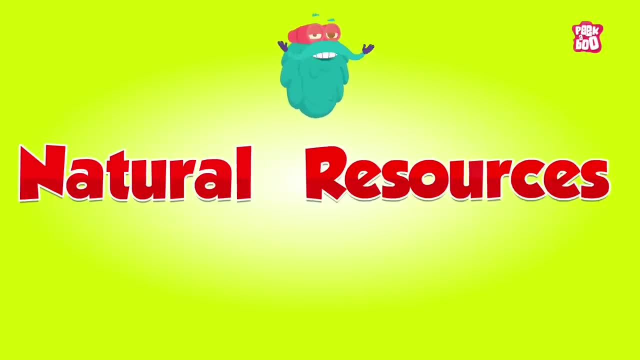 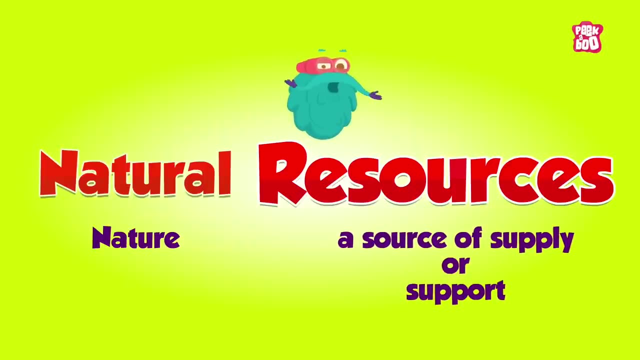 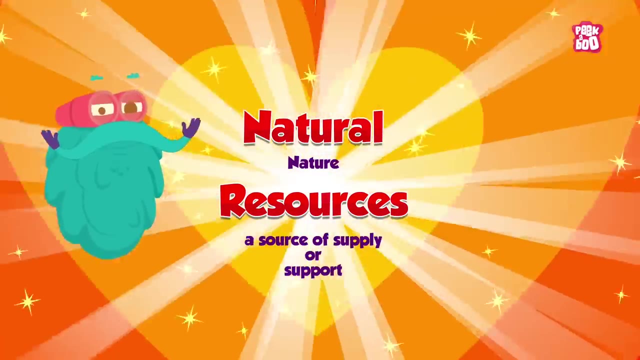 is in the word itself. Yes, natural refers to Mother Nature, and resources stands for a source of supply or support, So when we put these words together, it simply means anything that is supplied by Mother Nature that can be used. 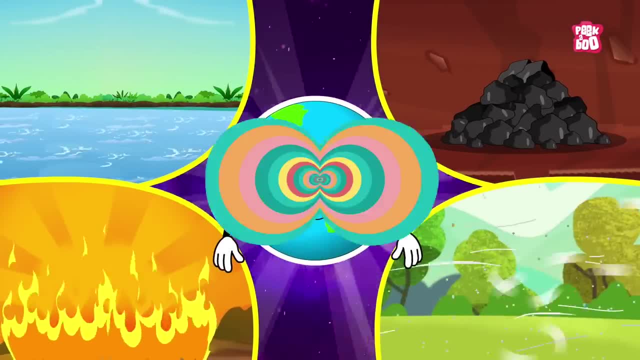 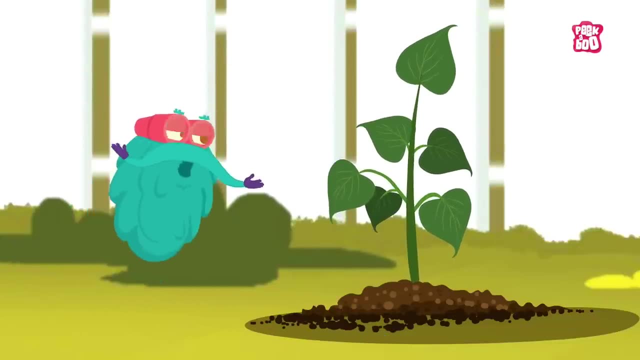 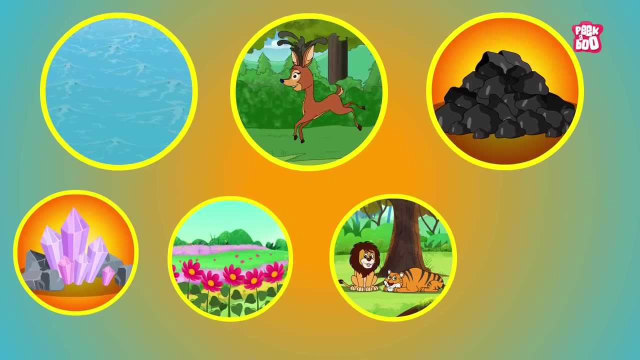 by the living beings. Natural resources are present on our planet on their own and do not need any human activity for their creation. Common examples of natural resources include water, forests, fossil fuels, minerals, plants, animals and even air. 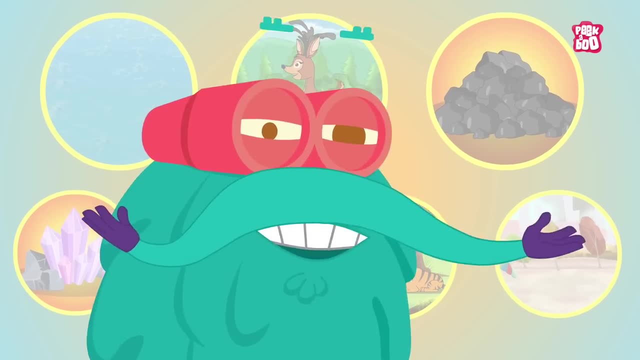 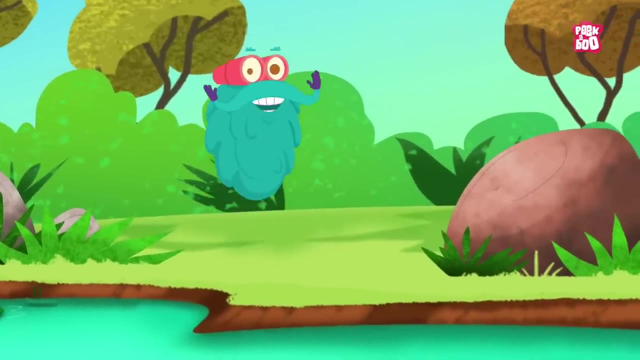 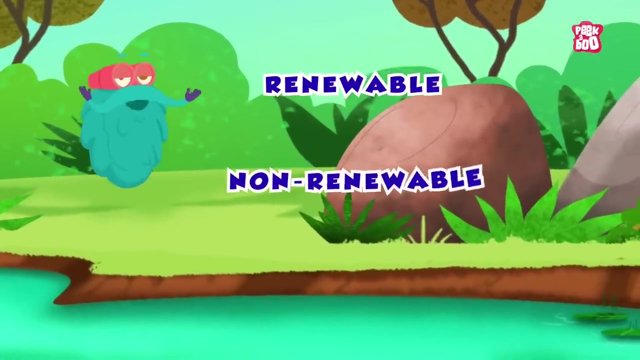 which are a must for our development and survival, And based on their available amount and durability. these resources are classified into two types: renewable and non-renewable natural resources. Let us look at them in detail. 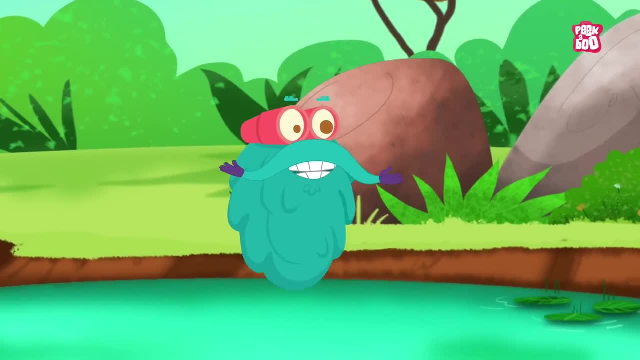 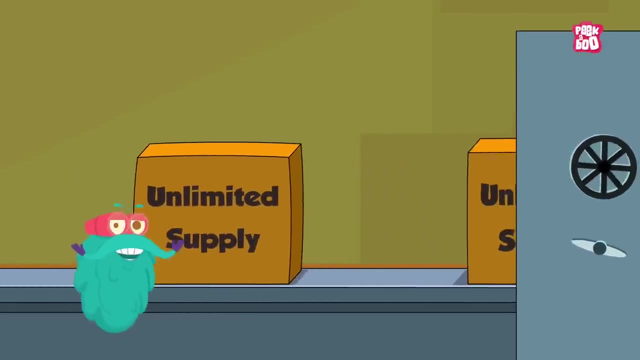 Natural resources that have an unlimited supply and can be used again and again are called renewable or inexhaustible resources. For example, air, sunlight and water are renewable or inexhaustible resources. 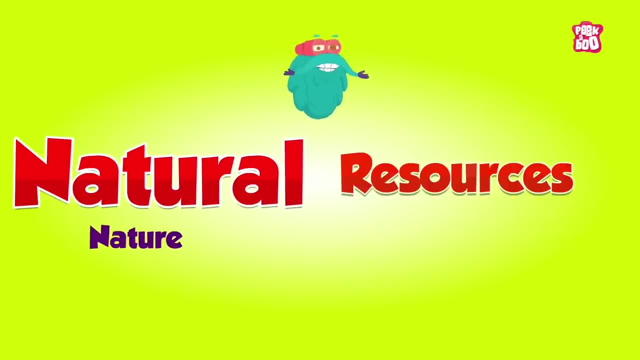 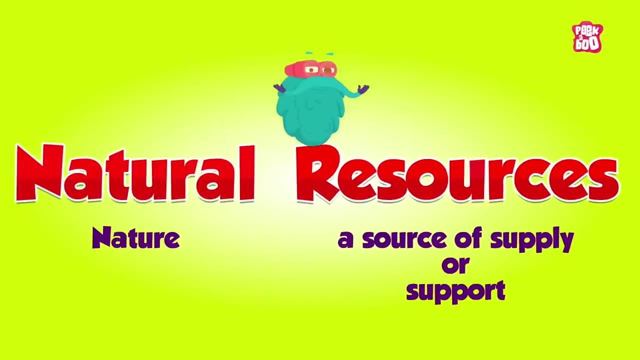 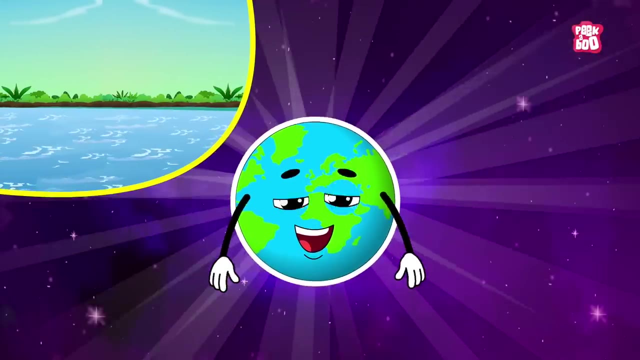 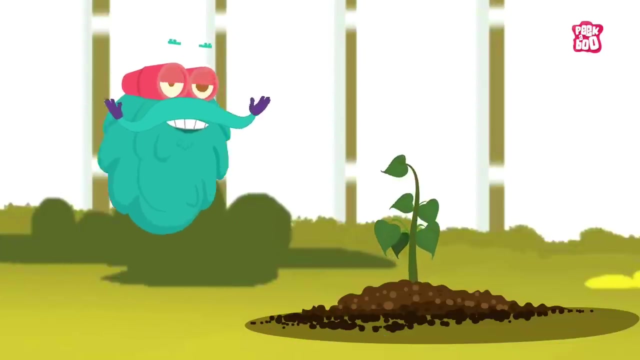 Yes, natural refers to Mother Nature, and resources stands for a source of supply or support, So when we put these words together, it simply means anything that is supplied by Mother Nature that can be used by the living beings. Natural resources are present on our planet on their own. 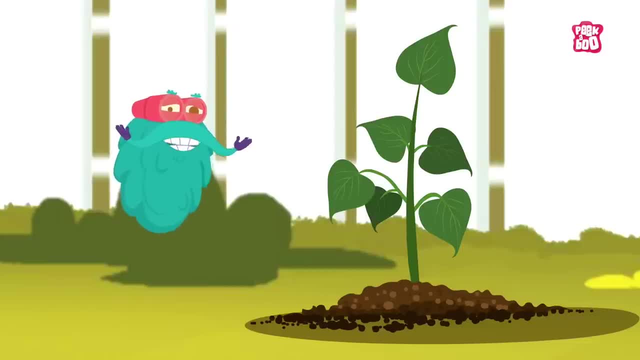 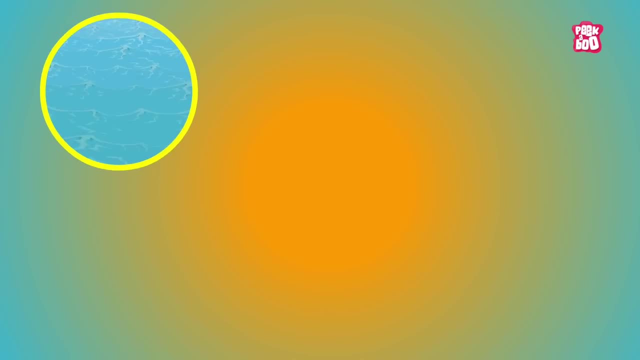 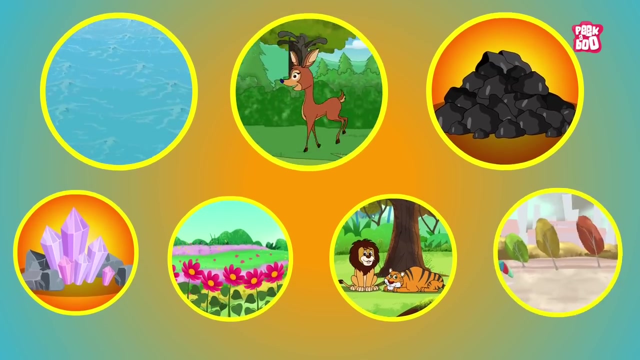 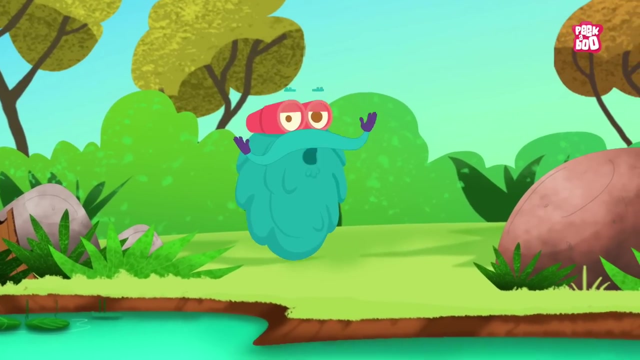 and do not need any human activity for their creation. Common examples of natural resources include water, forests, fossil fuels, minerals, plants, animals and even air, which are a must for our development and survival And based on their available amount and durability. 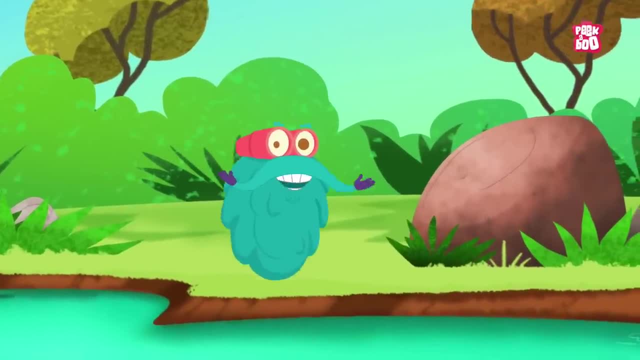 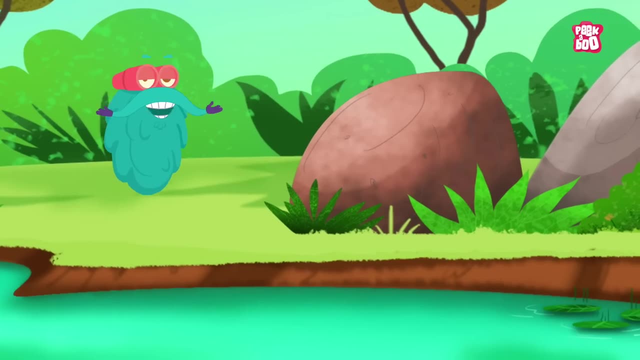 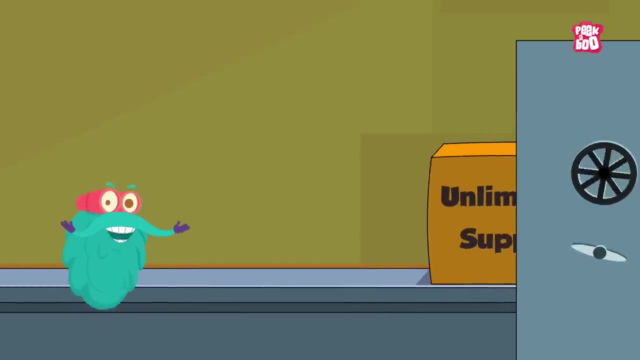 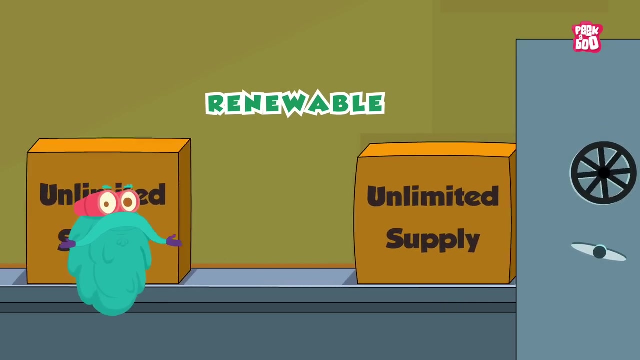 these resources are classified into two types: renewable and non-renewable natural resources. Let us look at them in detail. Natural resources that have an unlimited supply and can be used again and again are called renewable or inexhaustible resources, For example. 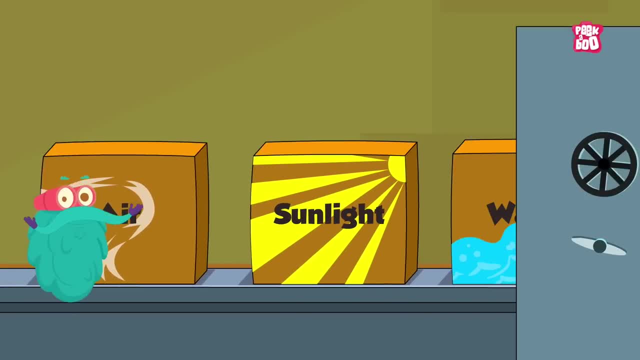 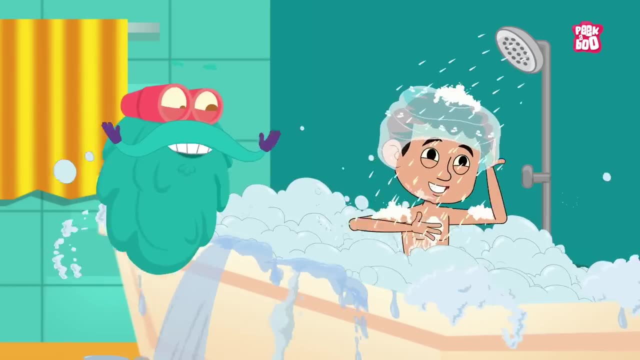 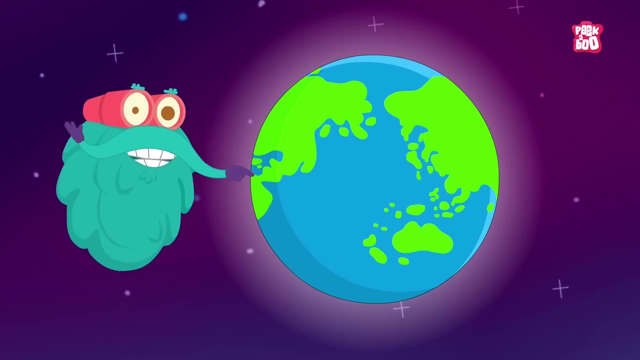 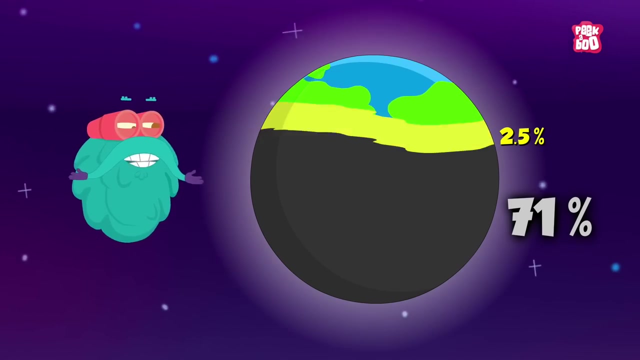 air, sunlight and water are renewable resources. However, in some cases, water is not renewable easily and cannot be used once it gets chemically polluted. On top of that, out of 71% of total water available on Earth, only 2.5% of all 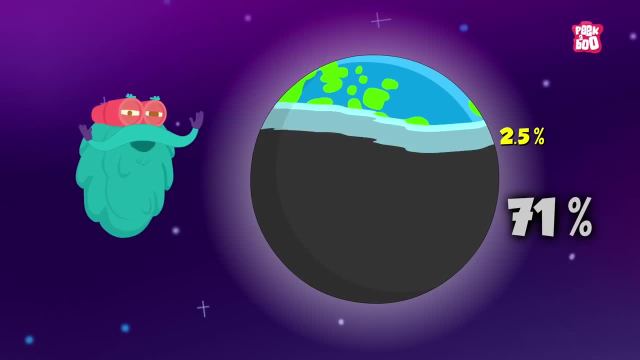 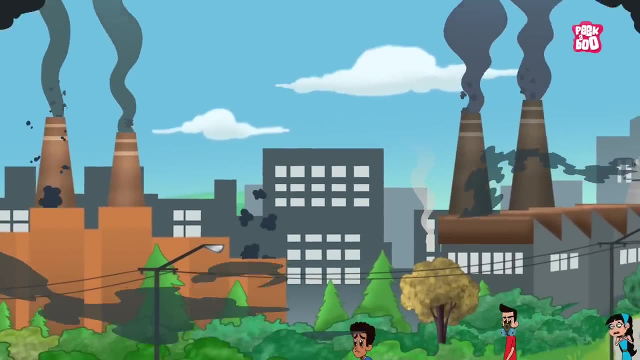 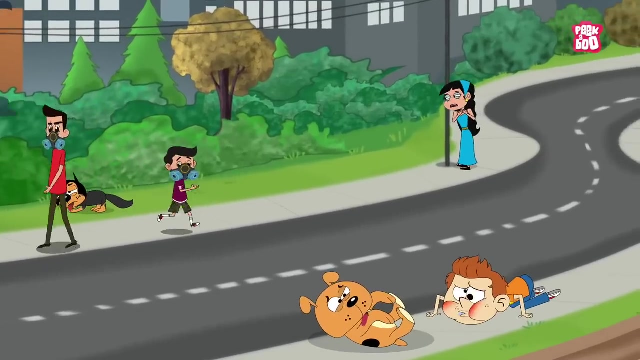 is fresh water, and only 0.3% of all of that is available on the surface. At the same time, even polluted air can be hazardous to all living beings, and therefore it is vital to take measures to reduce air pollution Now. 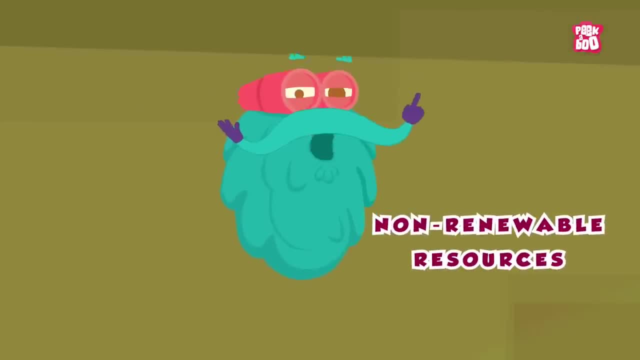 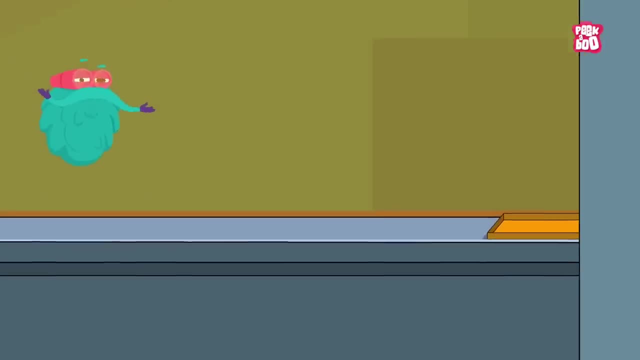 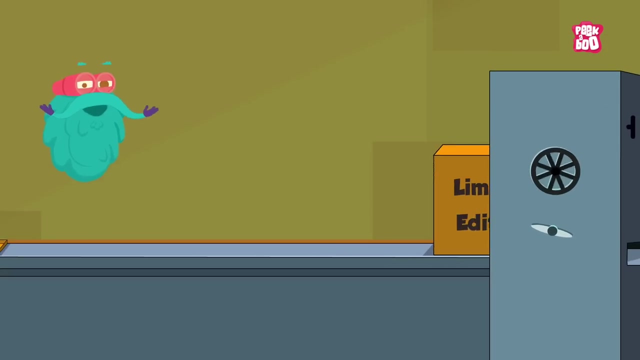 let us look into the definition of non-renewable resources. It simply means resources that are available in limited quantities or that do not grow and come back or take a very long time to come back. One of the cons of non-renewable resources is: 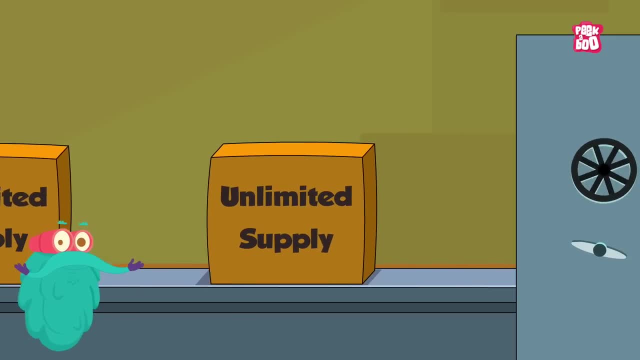 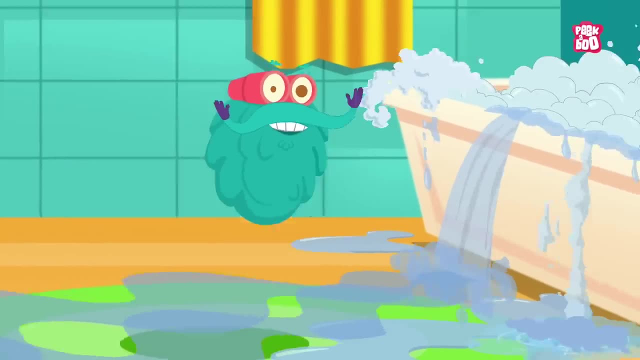 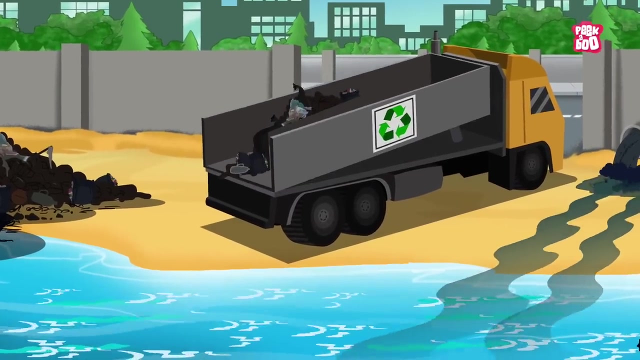 For example, air, sunlight and water are renewable or water are renewable resources. However, in some cases, water is not renewable easily and cannot be used once it gets chemically polluted On top of that. 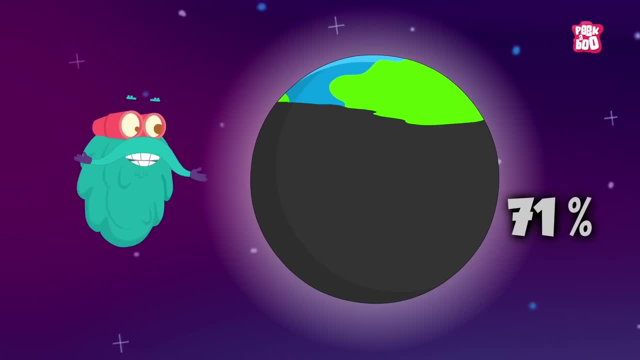 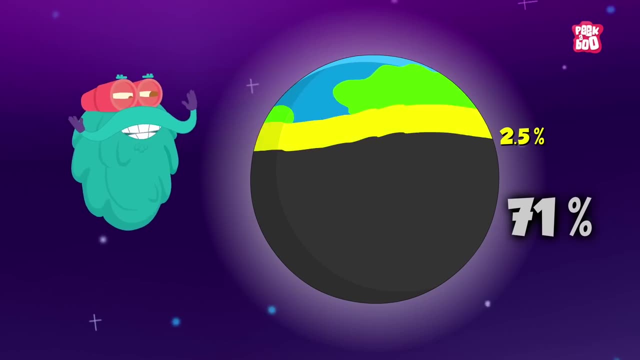 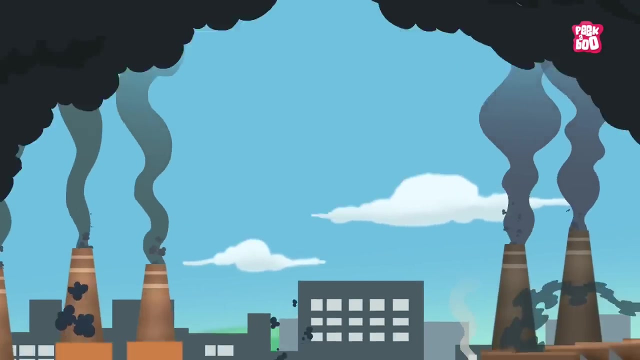 out of 71% of total water available on earth, only 2.5% of all is fresh water and only 0.3% of that is available on the surface. At the same time, even polluted air. 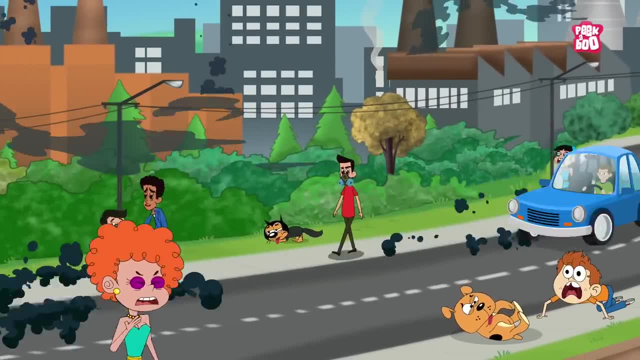 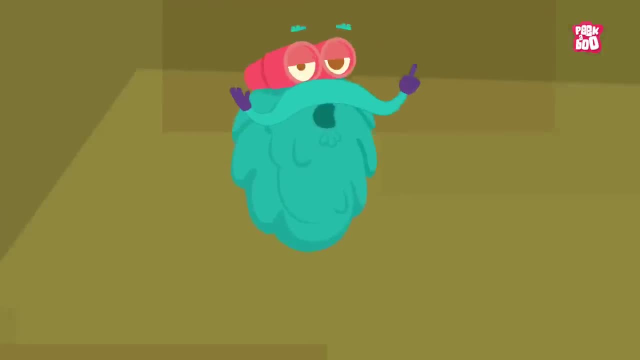 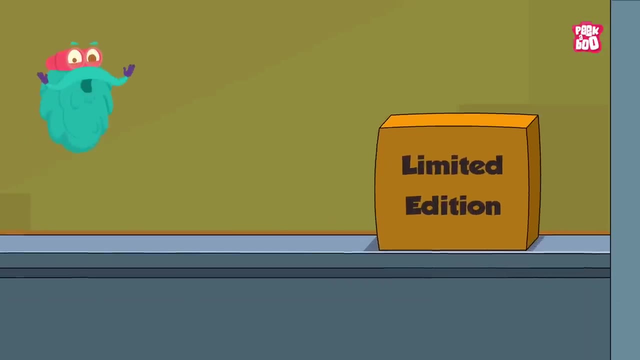 can be hazardous to all living beings and therefore it is vital to take measures to reduce air pollution. Now let us look into the definition of non-renewable resources. It simply means resources that are available. in limited quantities or that do not grow and come back or take a very long time to come back. One of the cons of non-renewable resources is if we don't preserve them. 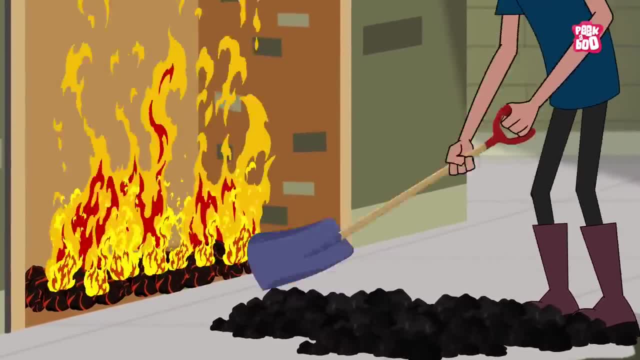 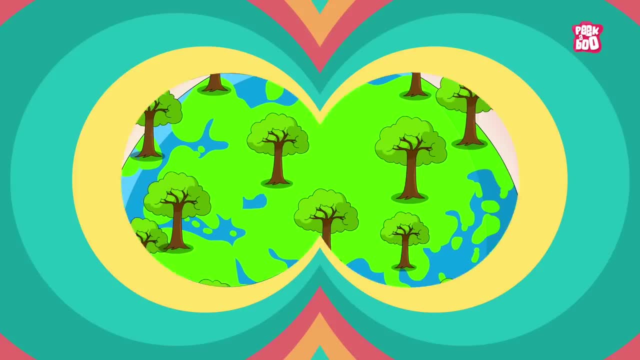 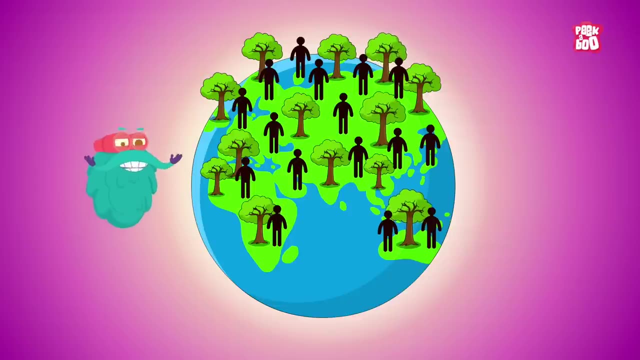 and waste them unnecessarily, due to which they might go extinct once and for all. Yes, as the human population is increasing at an alarming rate, we are using more and more natural resources. 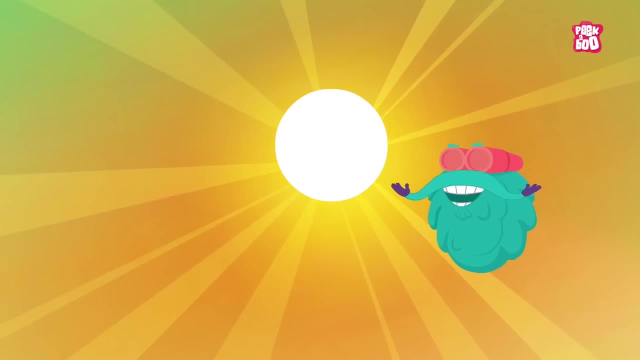 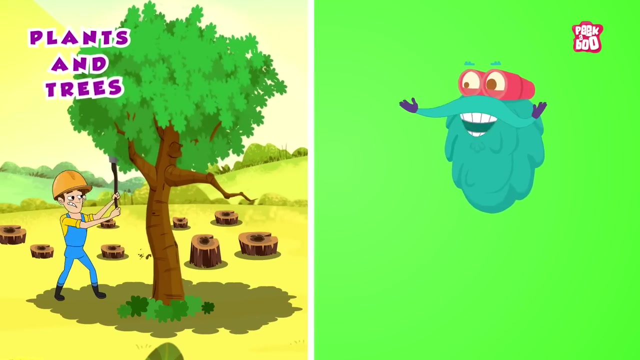 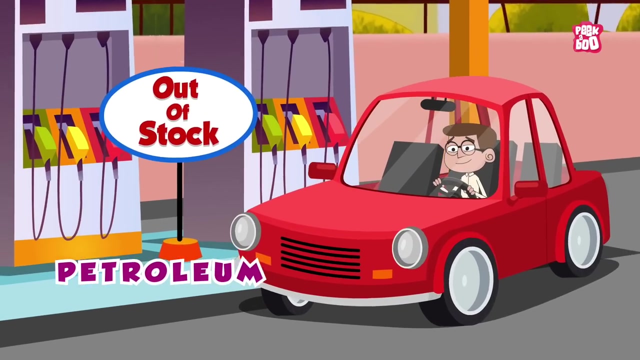 At this speed, science and technology will come when nature will not be able to supply us with resources such as plants and trees, animals, soil and fossil fuels such as coal, petroleum and natural 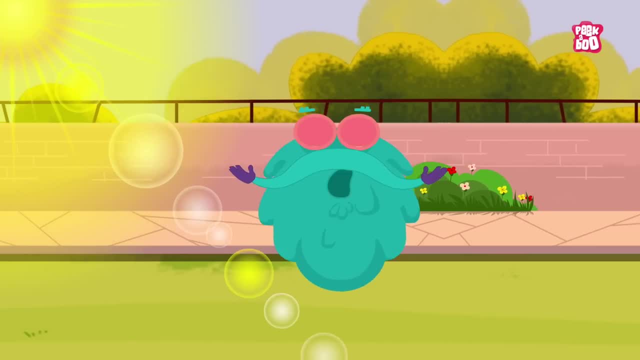 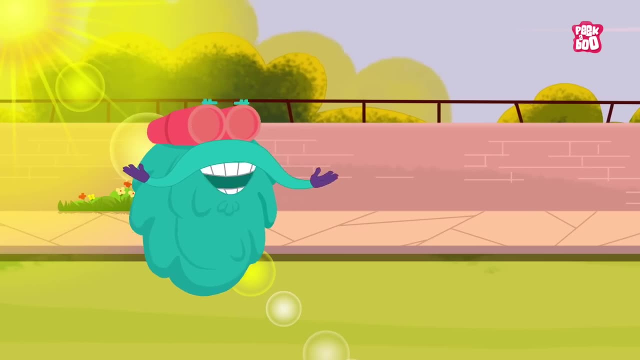 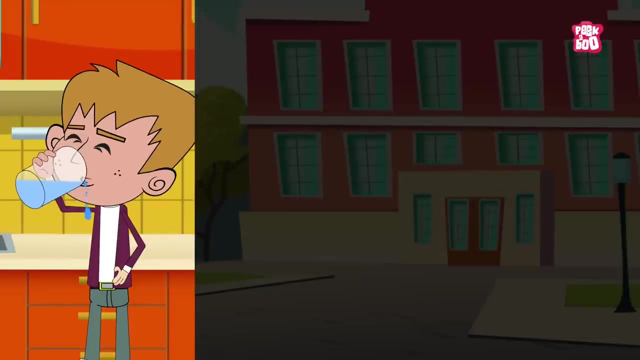 gas. Thus, these non-renewable resources can go exhausted, and for that reason they are also called exhaustible natural resources. Also, remember my friends: natural resources are very vital. 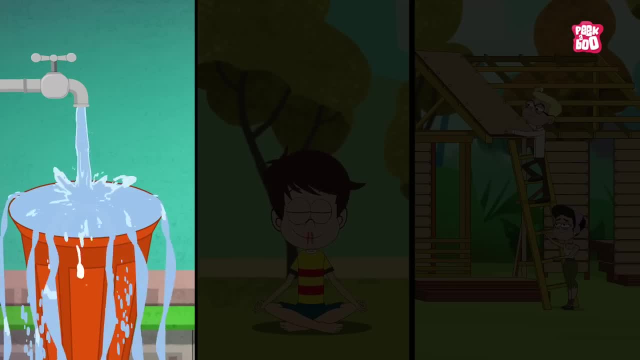 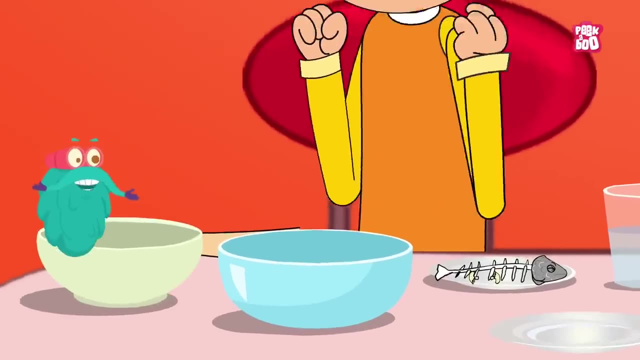 for human survival. So if they are not monitored carefully, there will come a time when there will be no food for the coming generation to eat, no material to build houses and even energy. 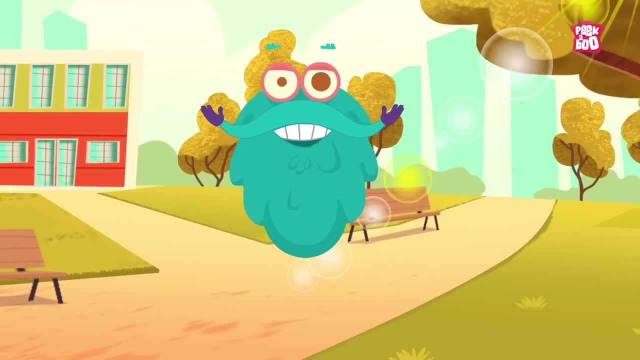 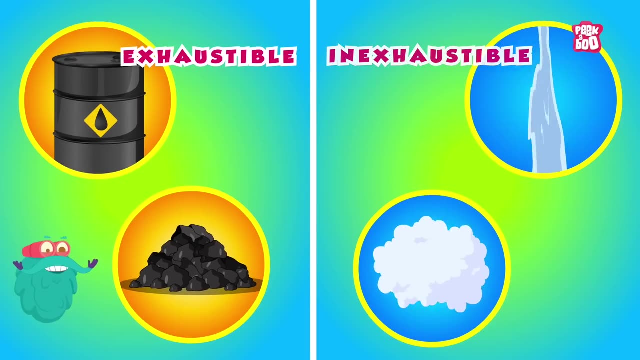 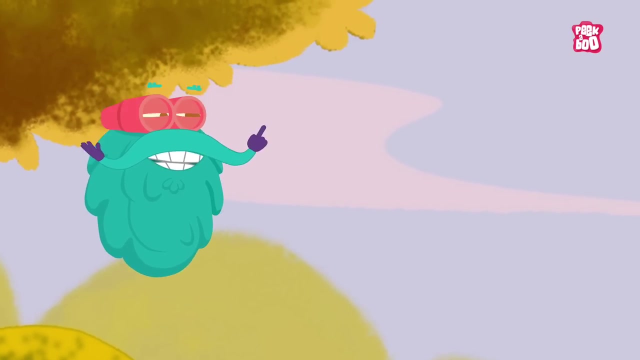 to run machines. Hence it is essential to know the difference between exhaustible and inexhaustible natural resources, and to practice sustainable development. This is nothing but the development that meets. 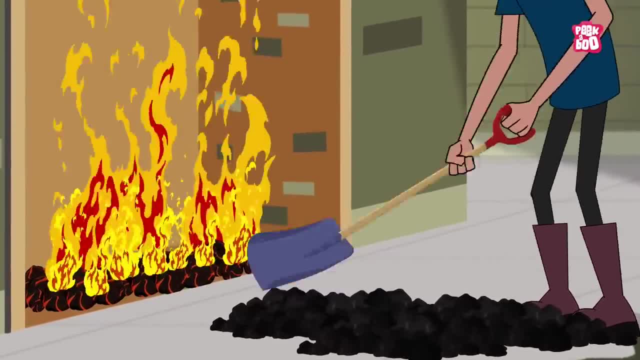 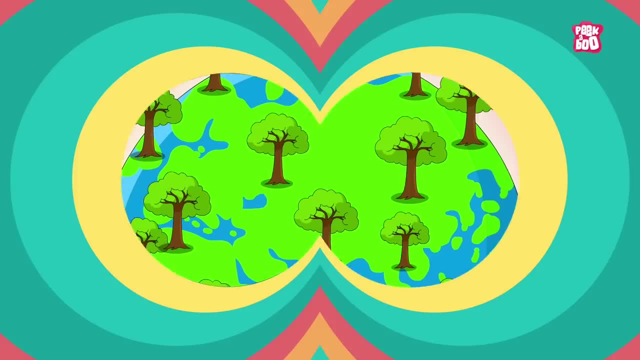 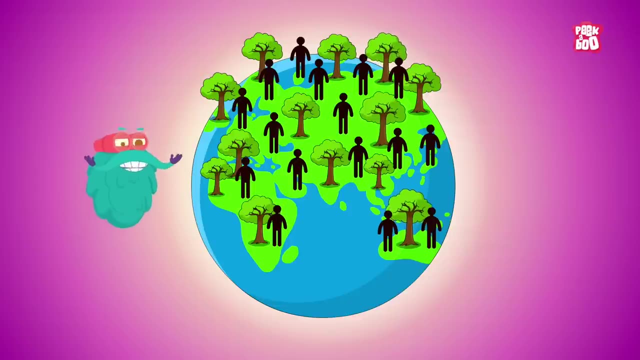 if we don't preserve them and waste them unnecessarily, due to which they might go extinct once and for all. Yes, as the human population is increasing at an alarming rate, we are using more and more natural resources At this speed. soon a day will come. 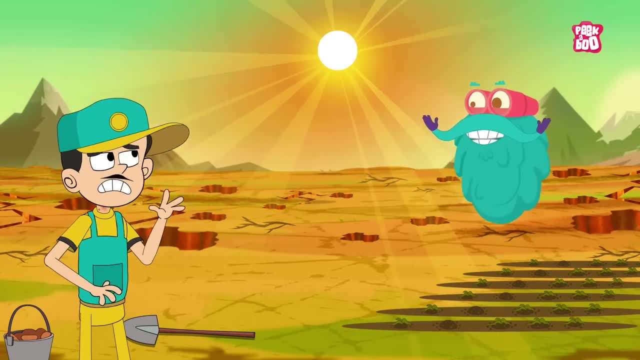 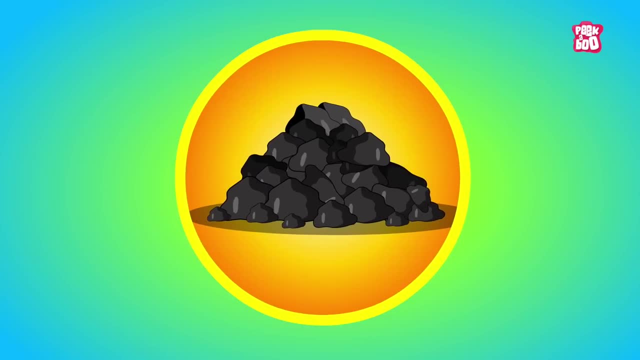 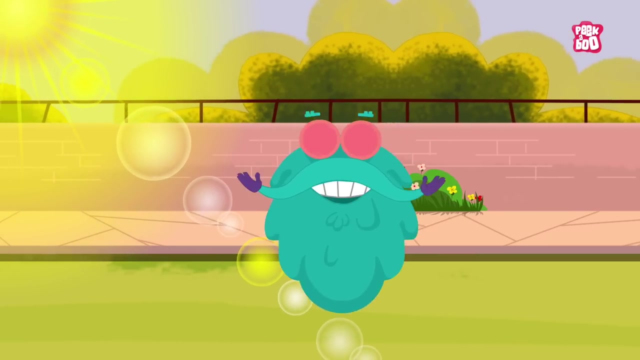 when nature will not be able to supply us with resources such as plants and trees, animals, soil and fossil fuels such as coal, petroleum and natural gas. Thus, these non-renewable resources can go exhausted, And for that reason they are also called. 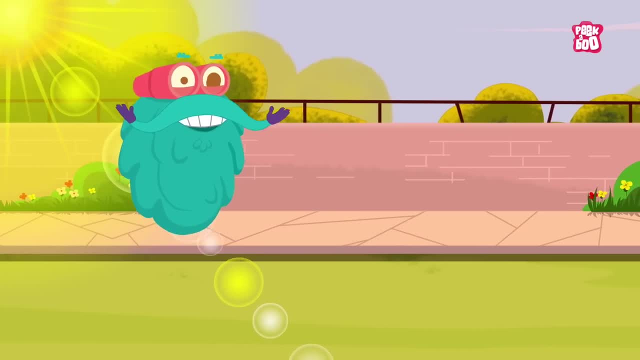 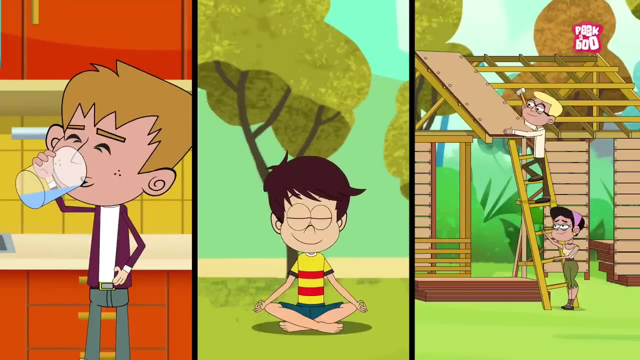 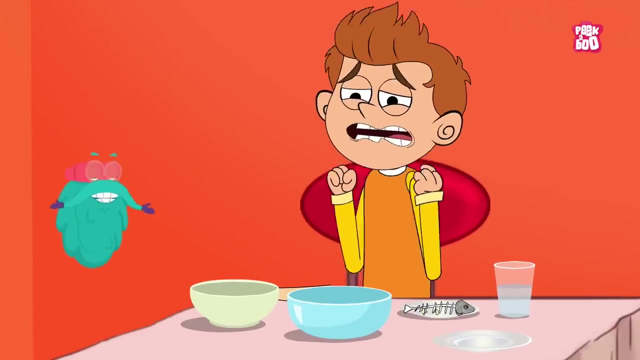 Exhaustible Natural Resources. Also, remember my friends, natural resources are very vital for human survival. So if they are not monitored carefully, there will come a time when there will be no food for the coming generation to eat, no material to build houses. 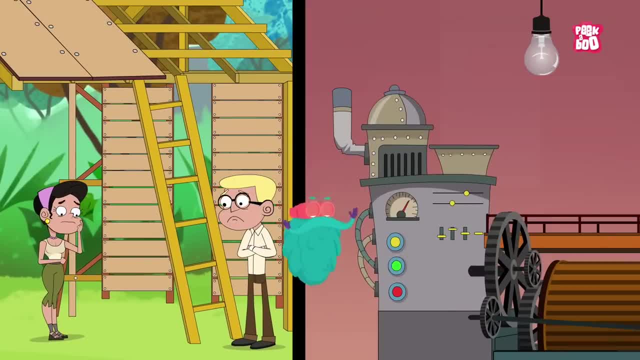 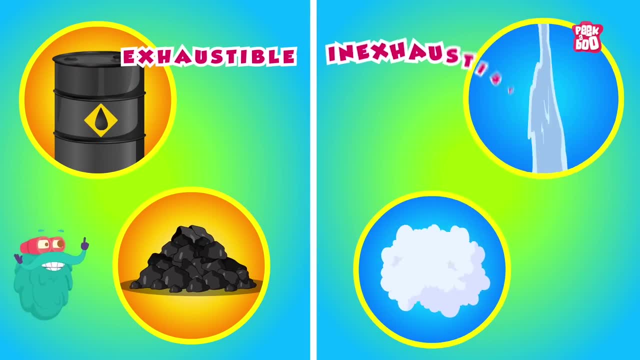 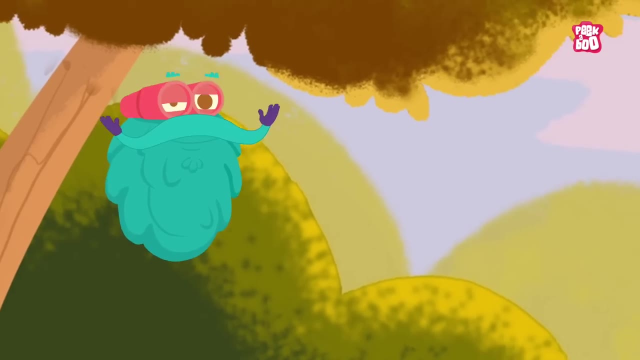 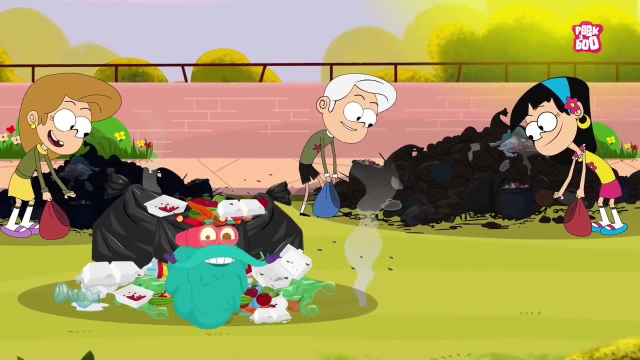 and even energy to run machines. Hence it is essential to know the difference between exhaustible and inexhaustible resources, and to practice sustainable development. This is nothing but the development that meets the needs of the present generation without compromising the ability of future generations. 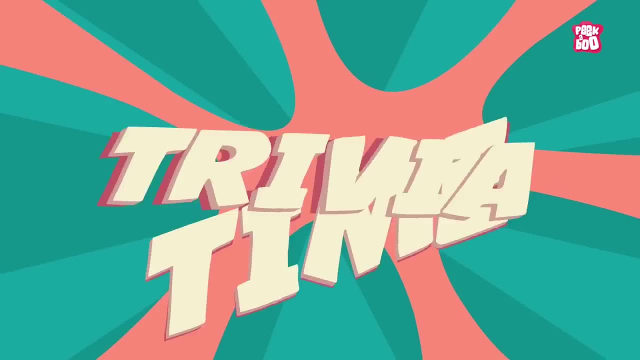 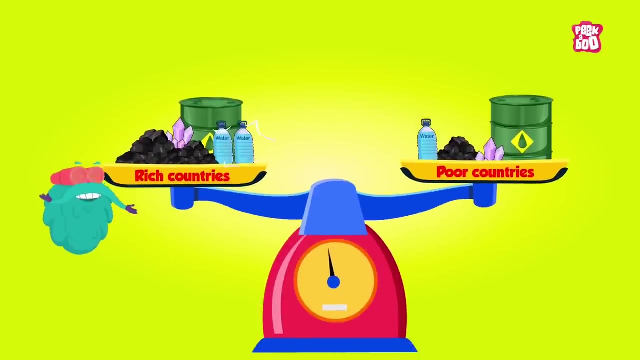 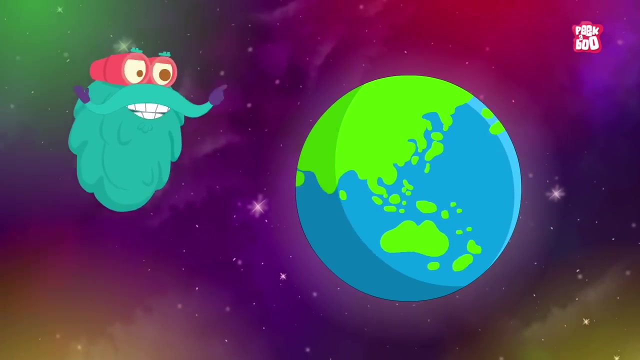 to meet their own needs. Did you know that people in rich countries consume up to 10 times more natural resources than those in the poorer countries? Yes, on average, an inhabitant of North America consumes around 90 kilograms of resources each day. 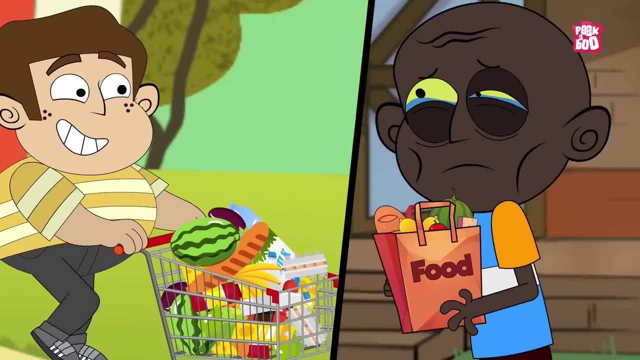 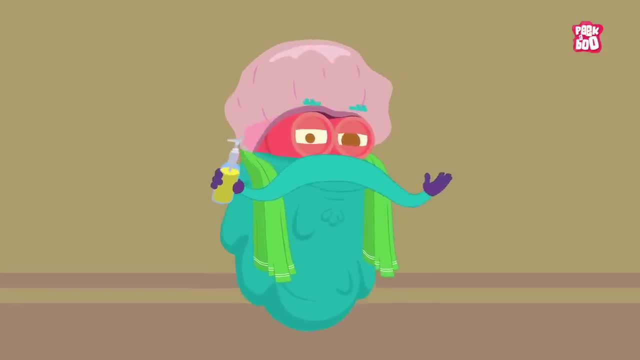 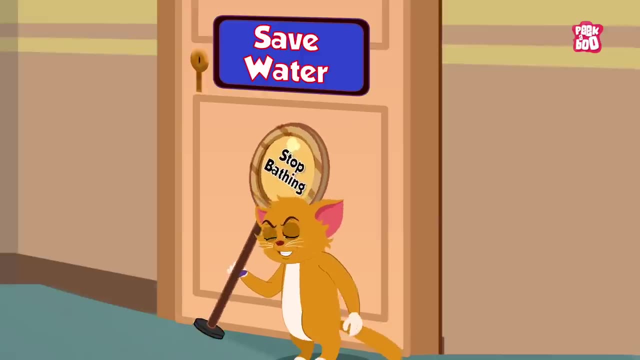 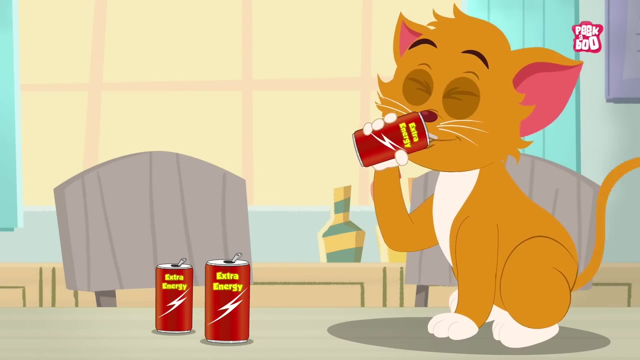 while in Africa people consume only around 10 kilograms per day. Hope you learned something new today. Until next time it's me, Dr Binox Zooming Out. Ah, Never mind. Oh, What are you drinking, little kitty? 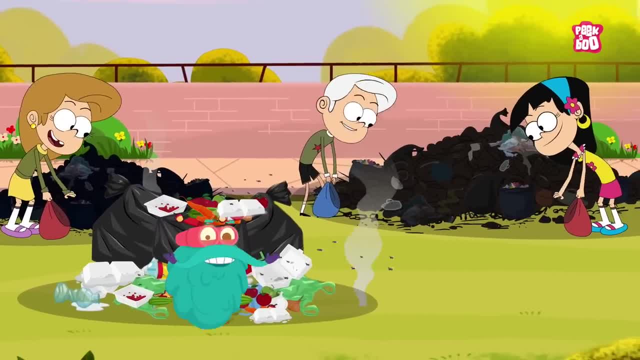 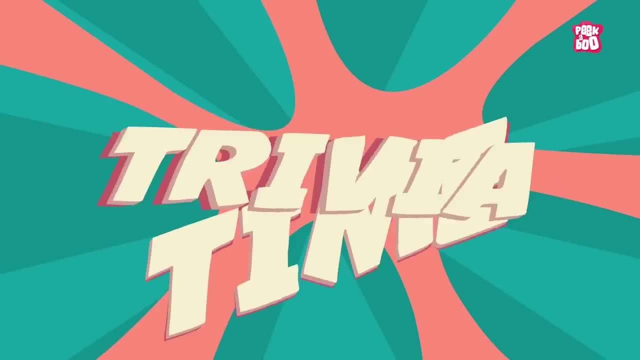 the needs of the present generation without compromising the ability of future generations to meet their own needs. Trivia Time. Did you know people in rich countries consume up to 10 times? 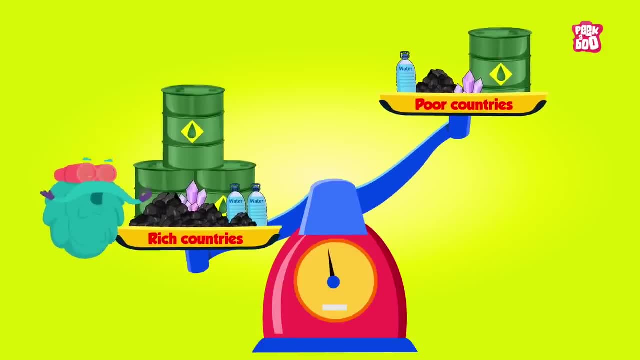 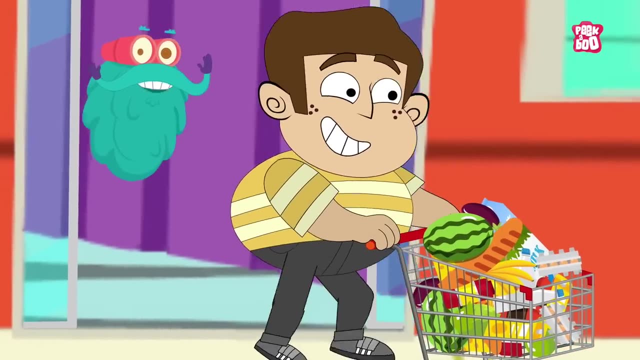 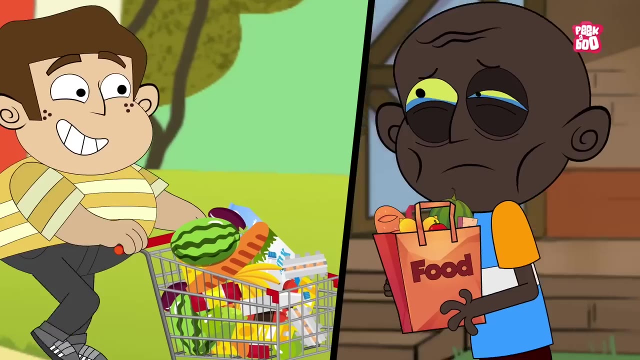 more natural resources than those in the poorer countries. Yes, on average, an inhabitant of North America consumes around 90 kilograms of resources each day, While in Africa, people consume only around 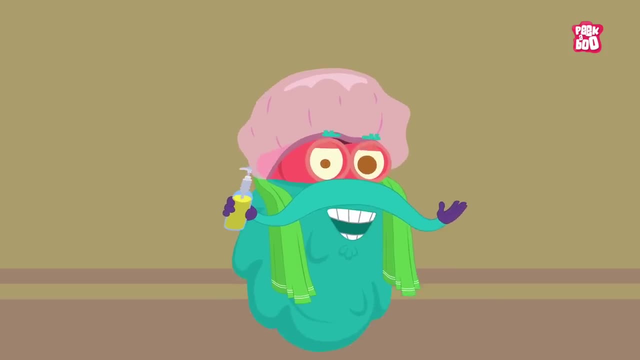 10 kilograms per day. Hope you learnt something new today. Until next time it's me Dr Binox Zooming Out. Ah, Never mind. Oh, What are you drinking, little kitty Energy? 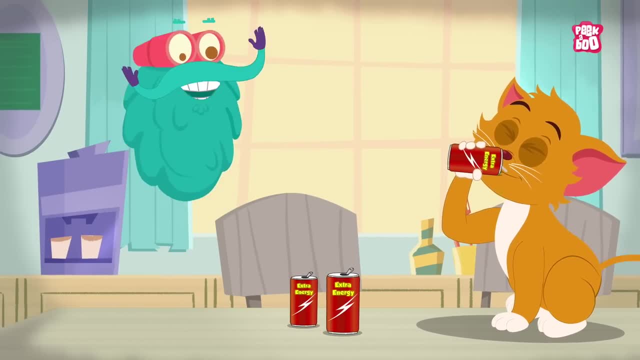 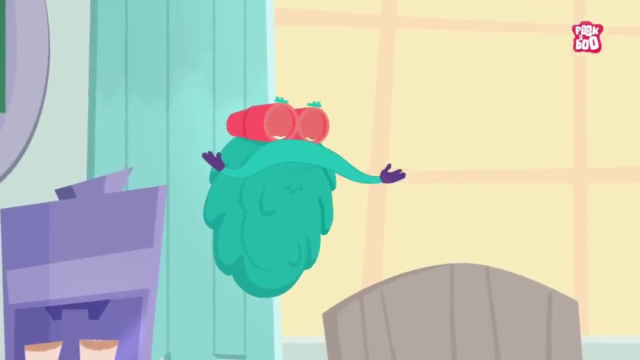 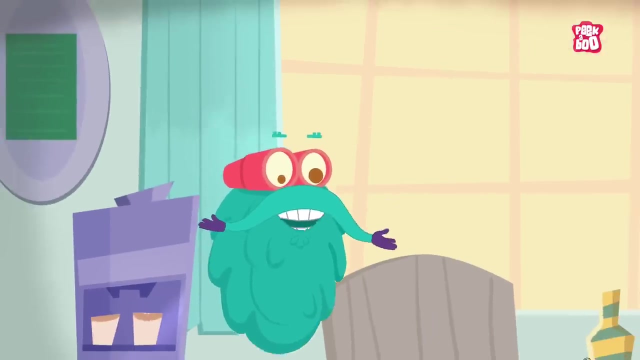 Hmm, It's better you sip some natural sources of energy than artificial ones. Why, That's an excellent question. So in today's episode, let me take you to this energetic 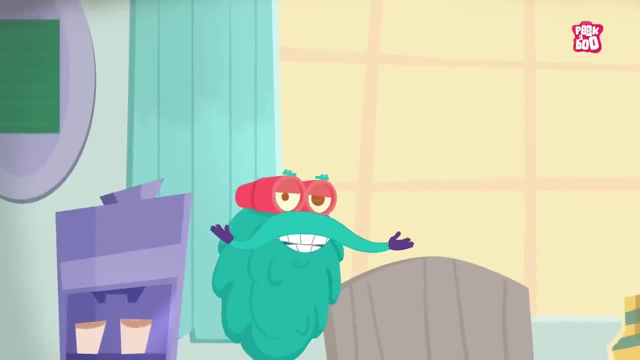 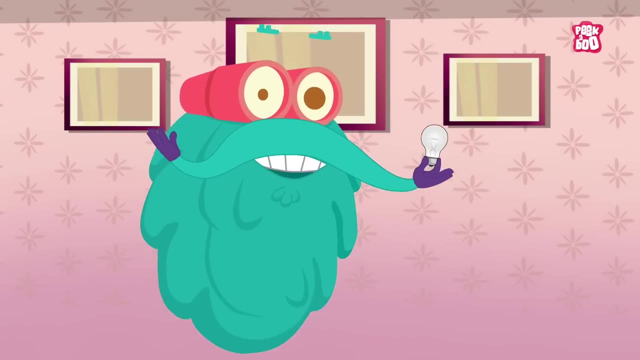 world of energy, which is the world of energy, and look at the sources of energy. Zoom in. Before we look into the energy sources, let us see what energy is in the first place. 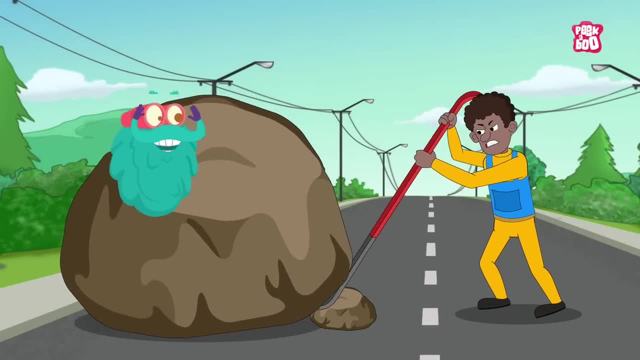 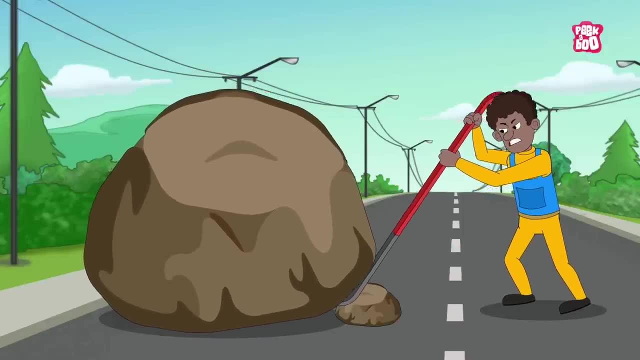 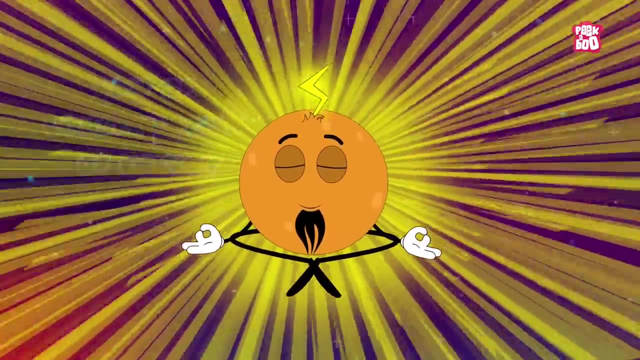 Well, according to the classical definition, energy is the ability to do work. But the vital question is: from where do we get so much energy? Well, according to the conservation of energy. 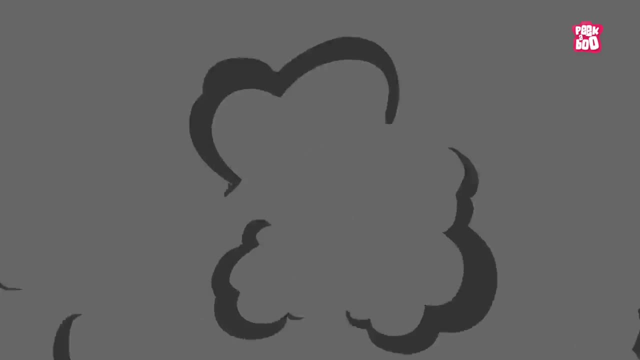 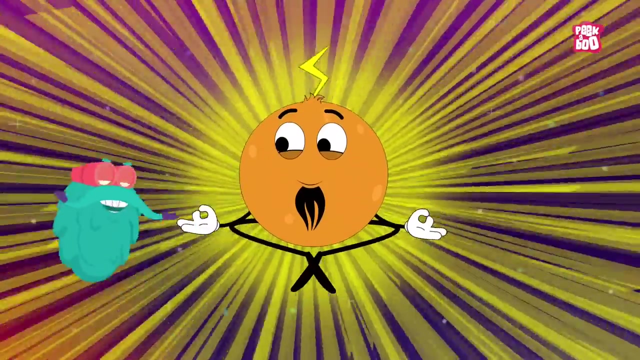 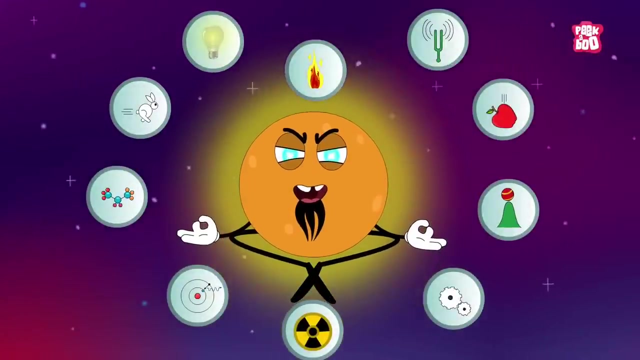 energy can neither be created nor be destroyed. It can only be wasted. Sorry, bad joke, But it may be transformed from one form to another, And if you take all forms of energy, 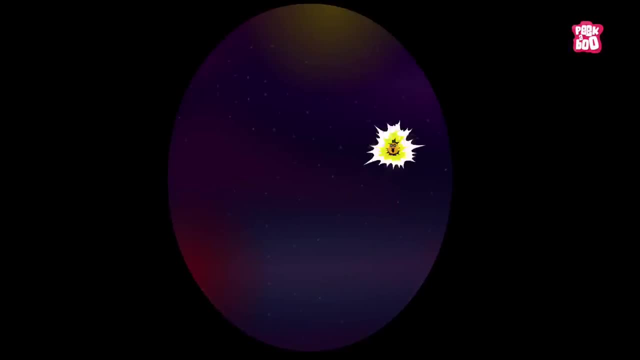 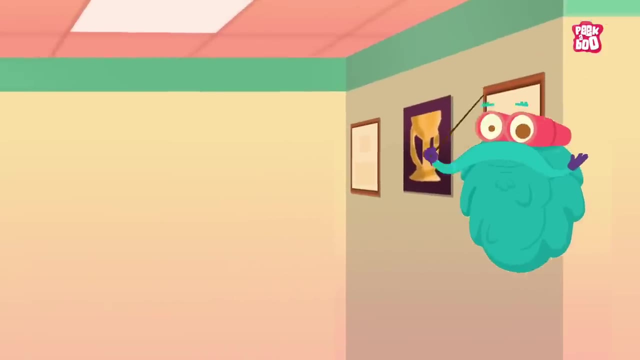 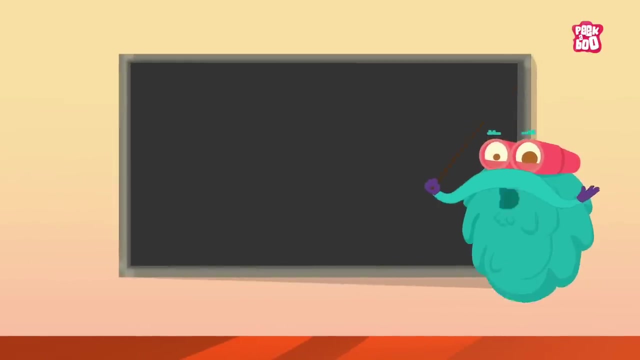 into account. the total energy of an isolated or closed system, like the universe, remains constant. How We can learn more about it? by observing how the sources of energy work, which can 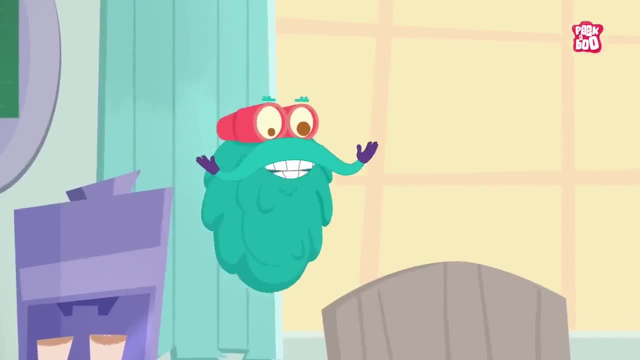 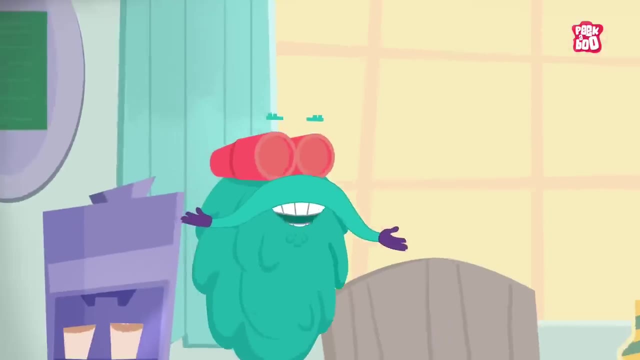 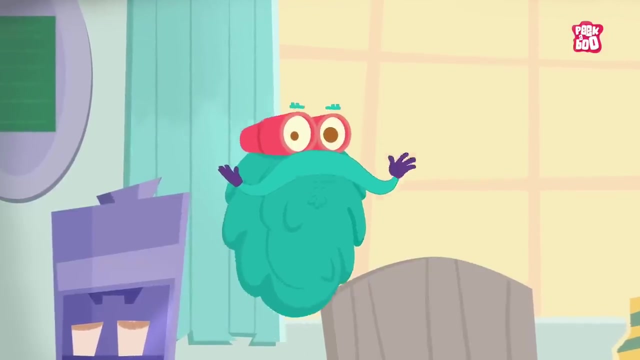 Energy. Hmm, It's better you sip some natural sources of energy than artificial ones. Why? That's an excellent question. So in today's episode, let me take you to this energetic world of energy and look at the sources of energy. 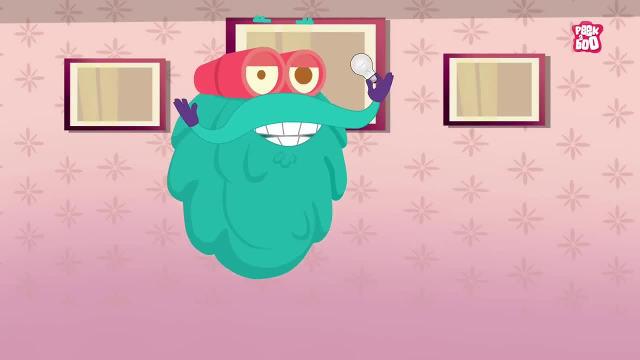 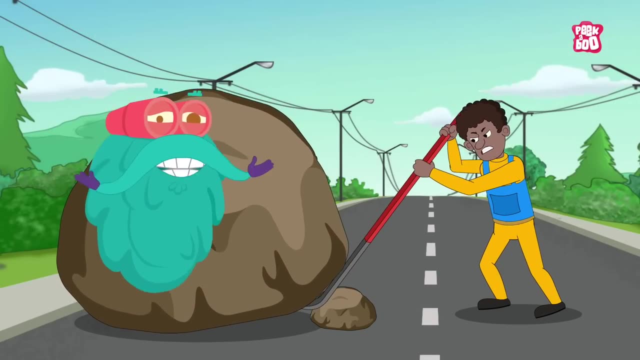 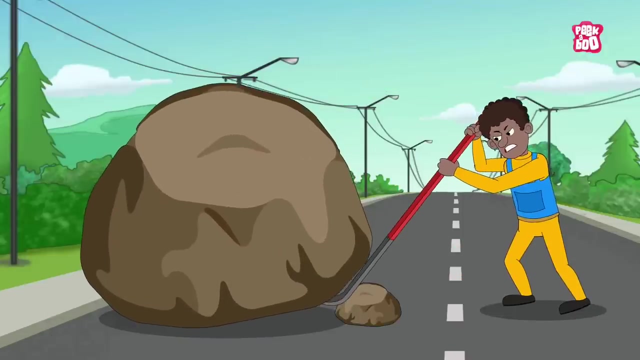 Zoom in. Before we look into the energy sources, let us see what energy is in the first place. Well, according to the classical definition, energy is the ability to do work. But the vital question is: from where do we get so much energy? 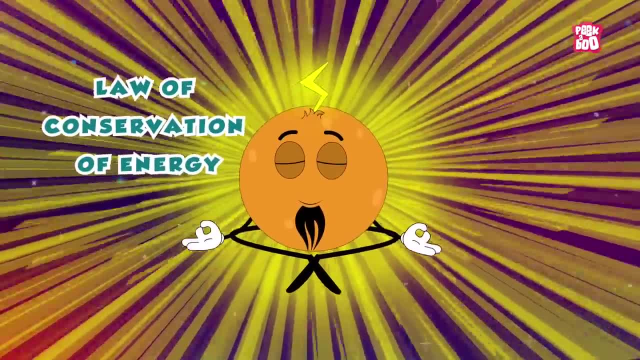 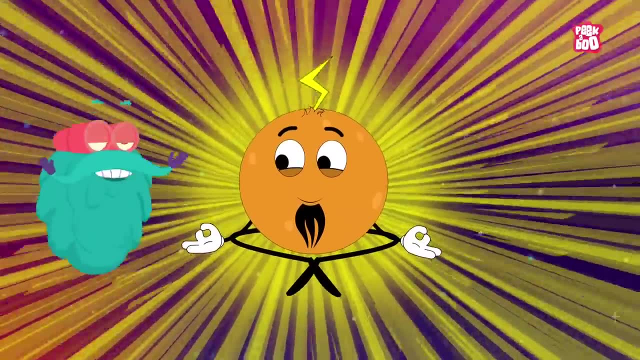 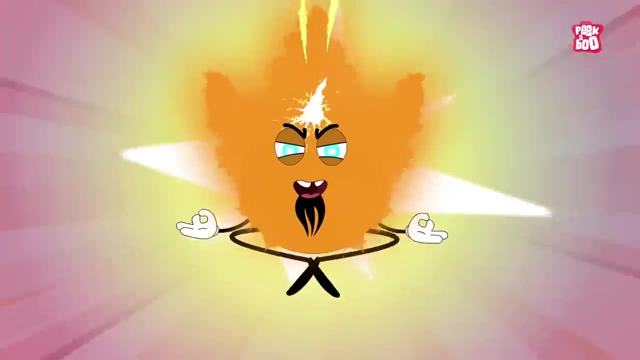 Well, according to the law of conservation of energy, energy can neither be created nor be destroyed. It can only be wasted. Sorry, bad joke, But it may be transformed from one form to another, And if you take all forms of energy into account, 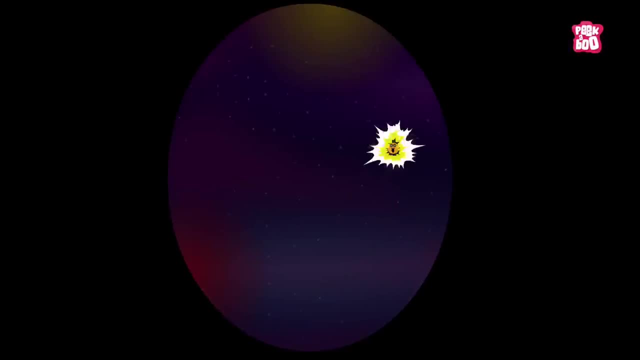 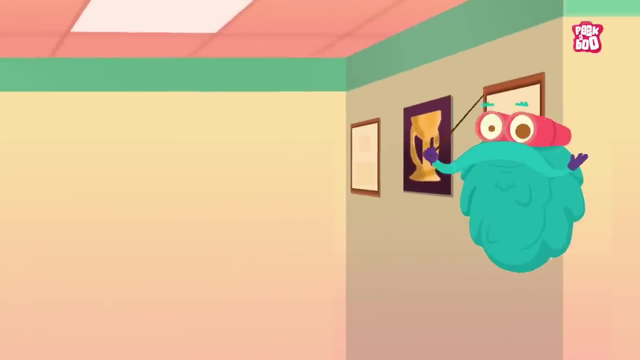 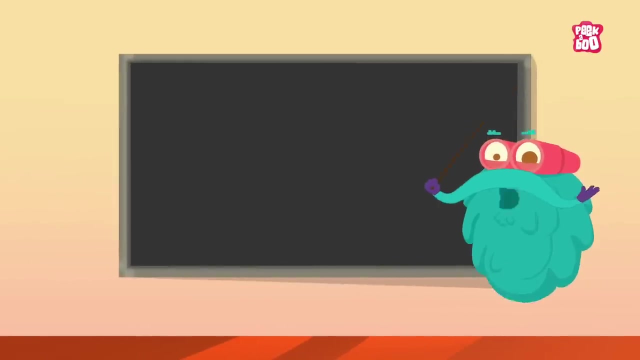 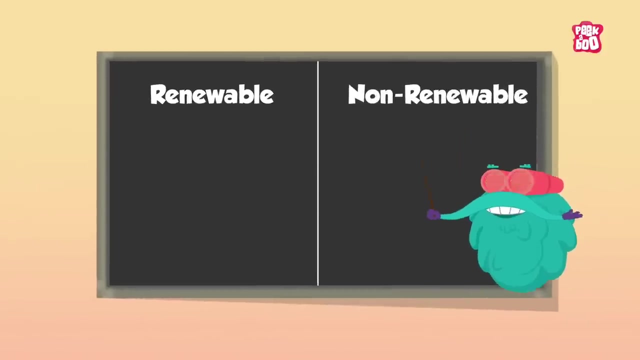 the total energy of an isolated or closed system, like the universe, always remains constant. How We can learn more about it? by observing how the sources of energy work, which can be classified into two forms: renewable and non-renewable sources of energy. And what are they? 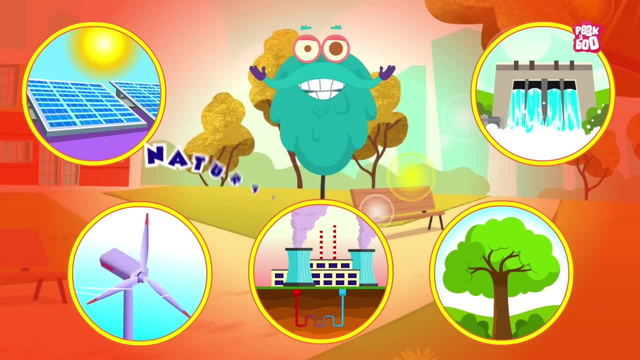 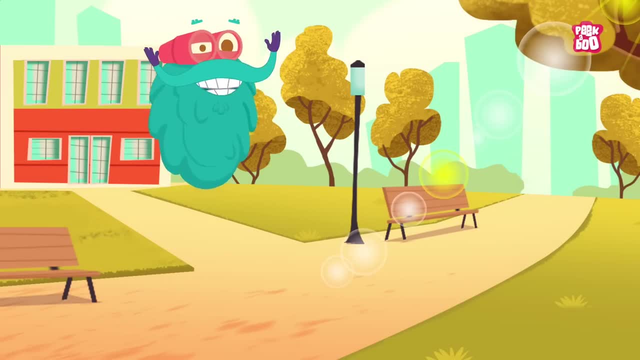 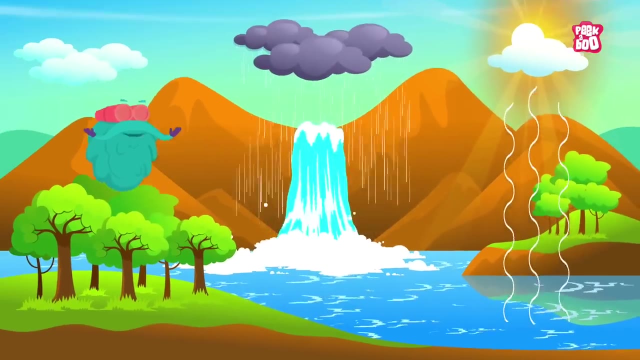 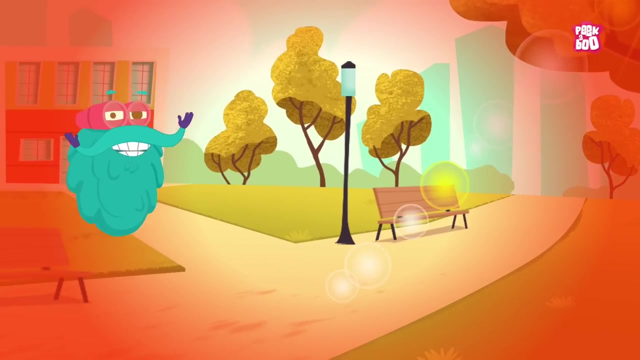 Renewable source is a natural resource that causes no impact on nature. They are available in abundance in nature and are sustainable. These resources of energy can be naturally refilled and are safe for the environment. Good examples of renewable sources of energy are solar energy. 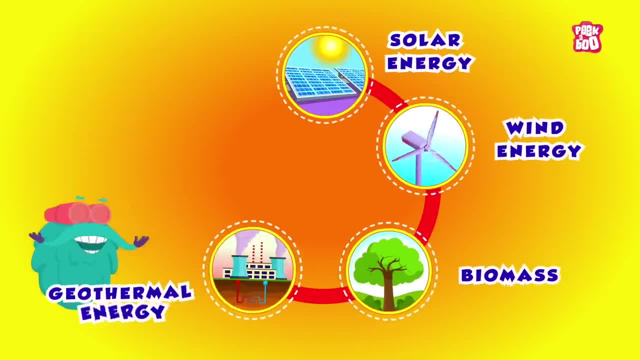 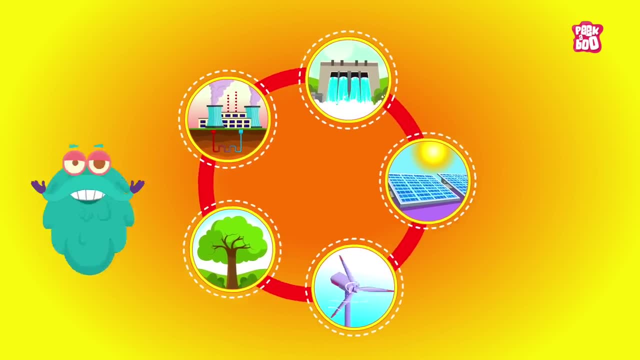 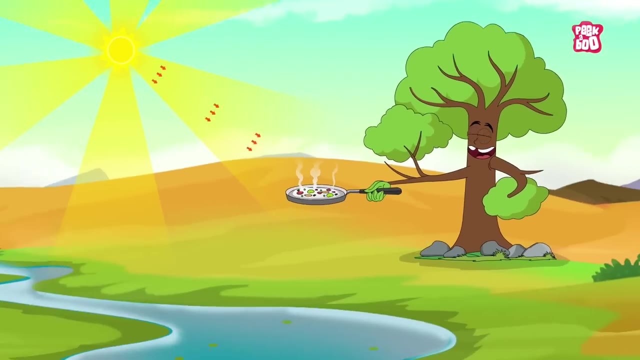 wind energy, biomass, geothermal energy and hydropower energy. So let us look at them one by one, starting with solar energy. The heat and light we receive from the sun are solar energy. This energy is then converted into electric energy. 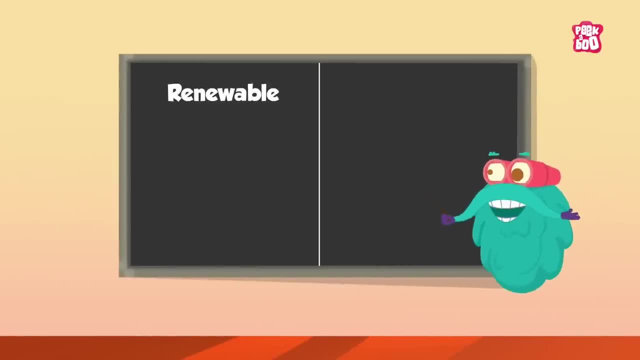 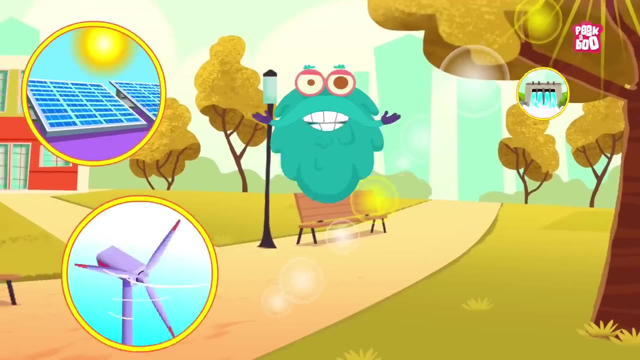 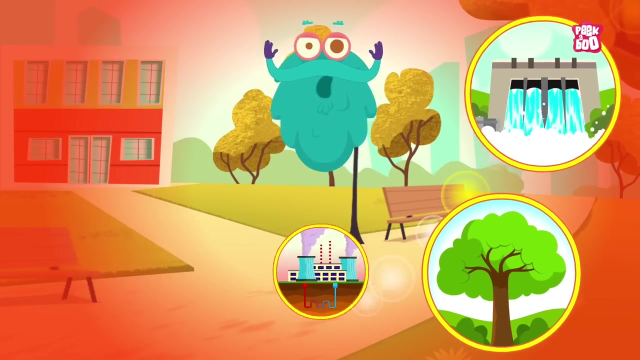 be classified into two forms: renewable and non-renewable sources of energy. And what are they? Renewable source is a natural resource that causes no impact on nature. They are renewable. 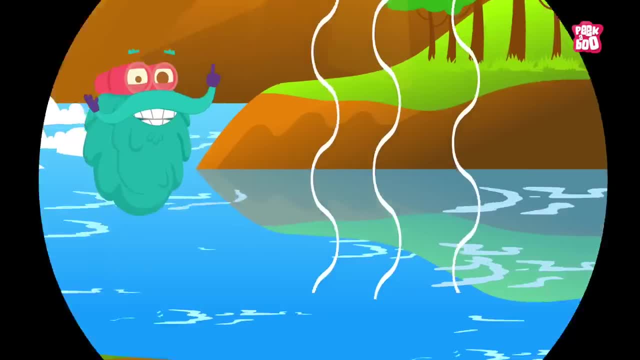 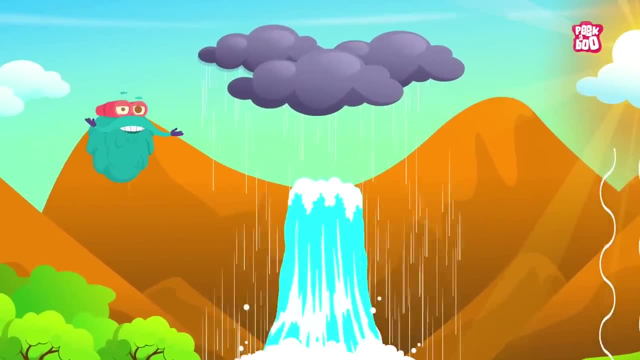 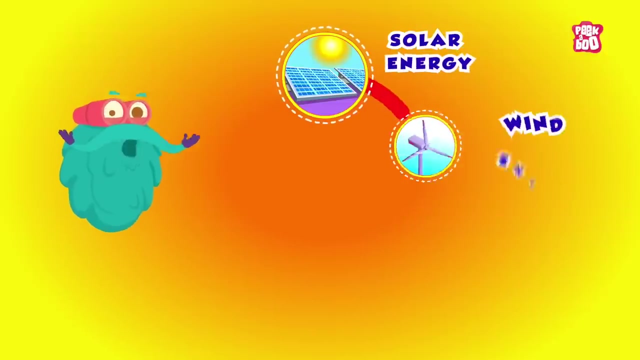 in abundance in nature and are sustainable. These resources of energy can be naturally refilled and are safe for the environment. Good examples of renewable sources of energy are solar energy. 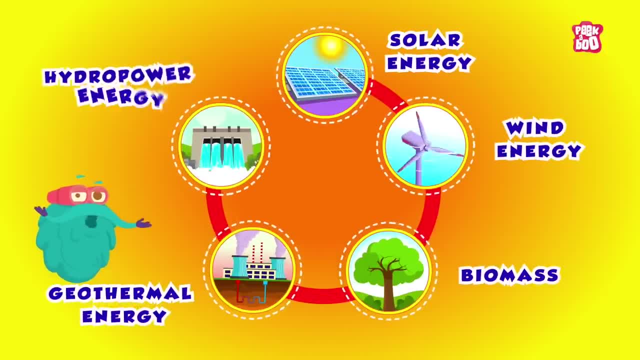 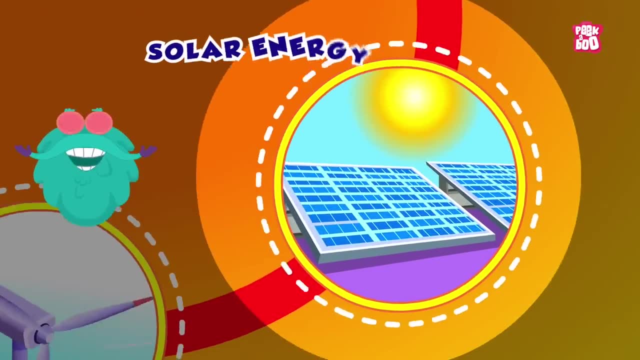 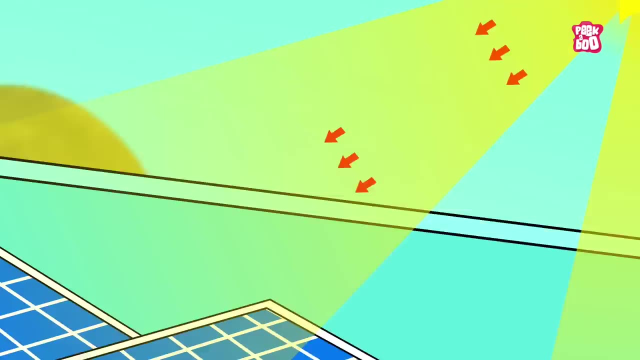 wind energy, biomass, geothermal energy and hydropower energy. So let us look at them. solar energy: The heat and light we receive from the sun are solar energy. This energy. 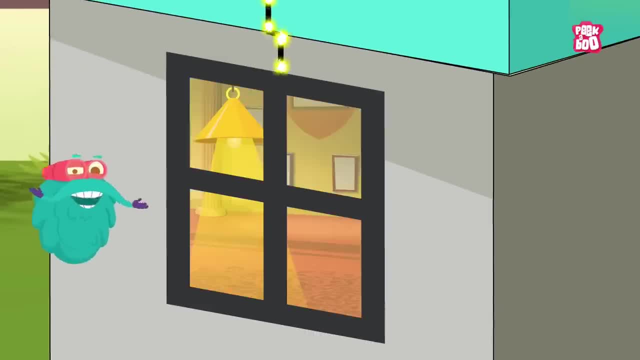 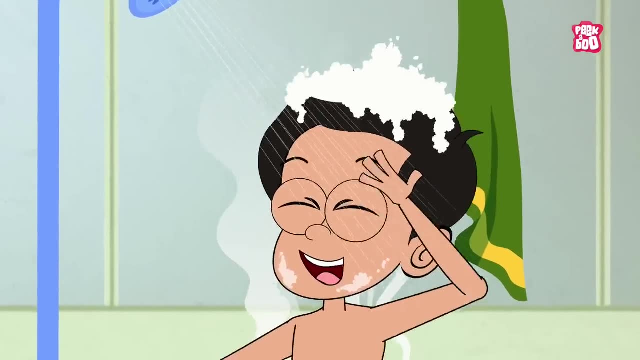 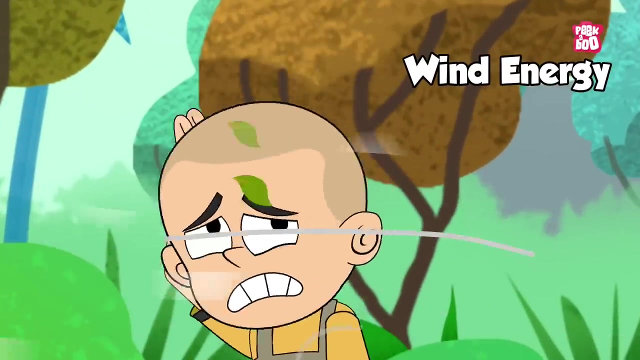 is then converted into electric energy with the help of solar panels. Also, it can be converted to thermal energy to heat our homes or water. Next comes another unlimited source called. 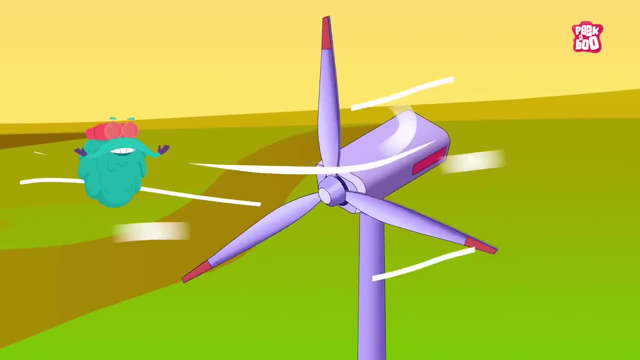 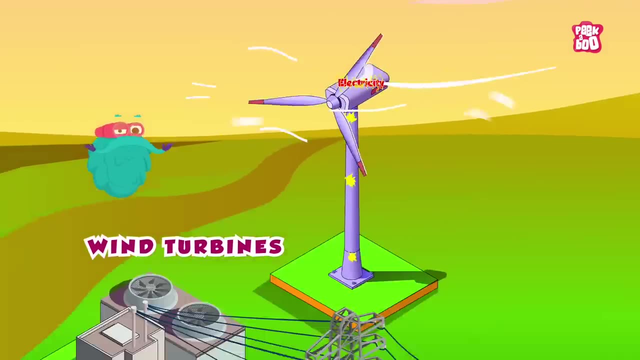 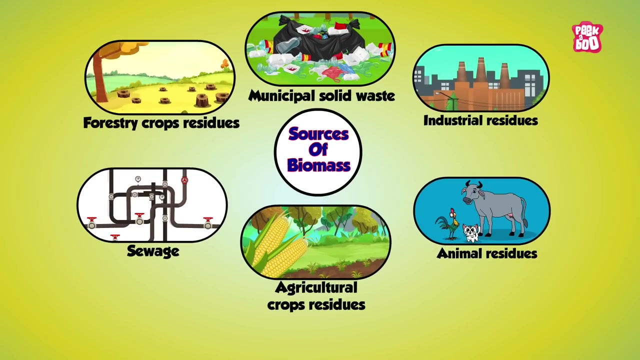 wind, energy, wind. This wind can be harnessed and converted into electricity using manmade structures called wind turbines that can light up our houses and schools. Now let us look into 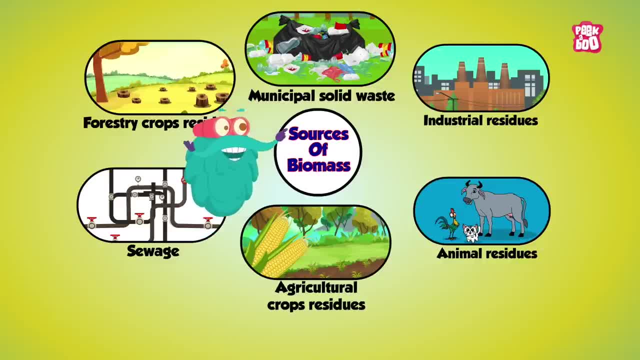 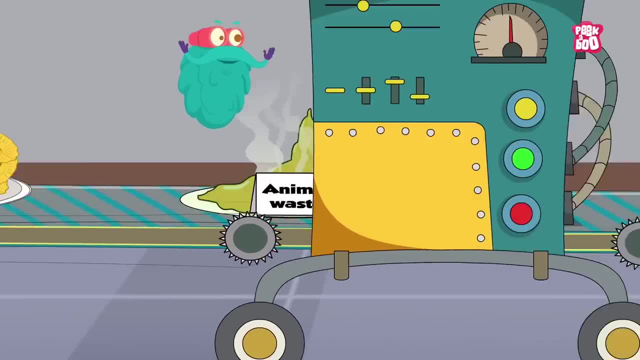 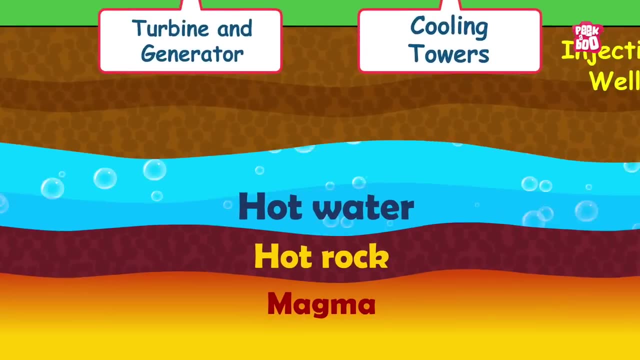 biomass, which is renewable organic matter that comes from plants and animals. Examples of biomass include wood and fuel. Next on the list is geothermal energy that comes from the heat. 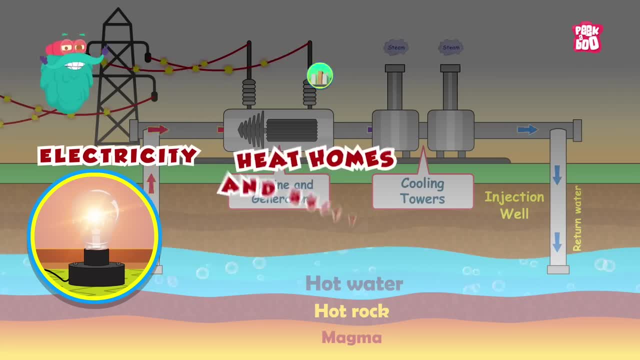 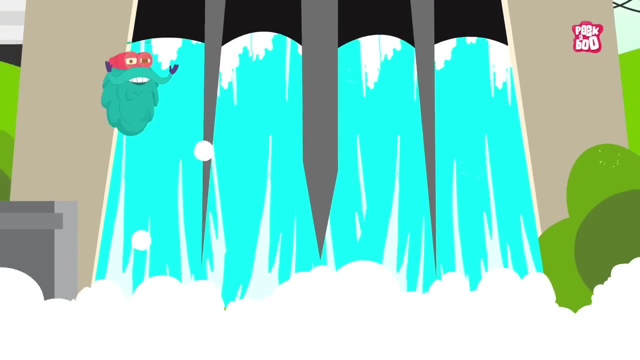 inside the earth. It can be used to produce electricity, heat homes and buildings and provide hot water. Speaking of water, moving water can also produce energy in the form of hydro power that can. 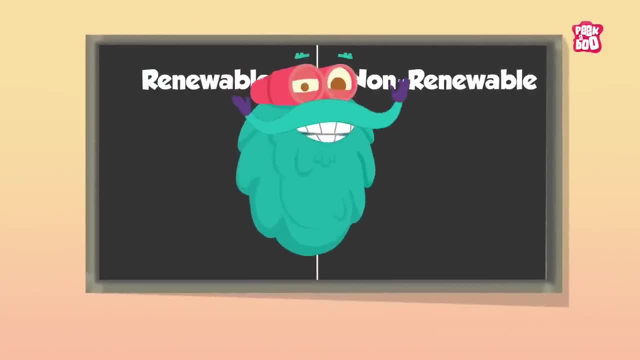 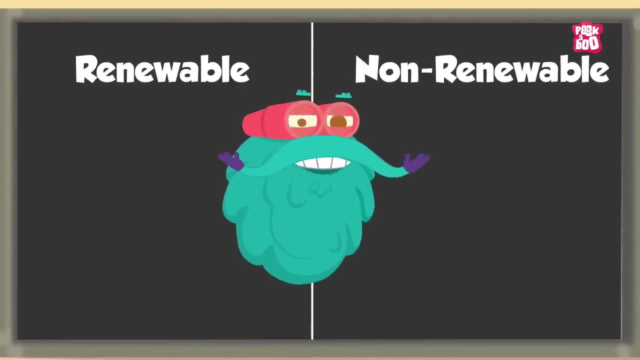 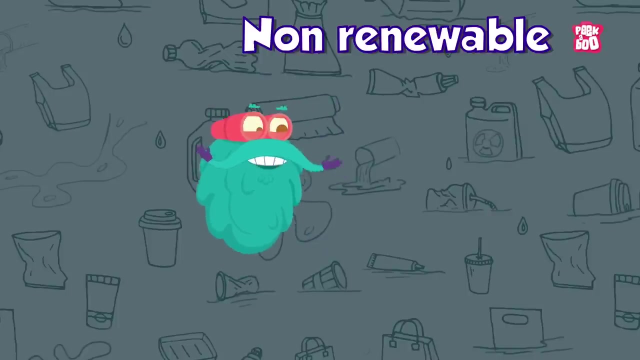 generate electricity. It is one of the oldest sources of renewable energy that is available in plenty on earth, But what is limited is non-renewable sources of energy that can. 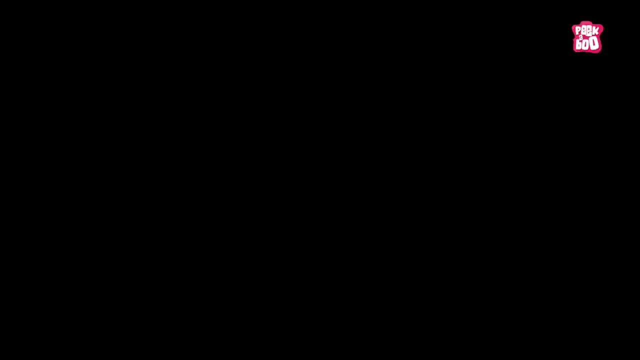 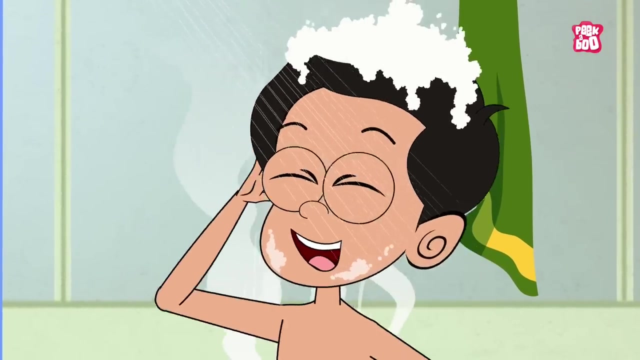 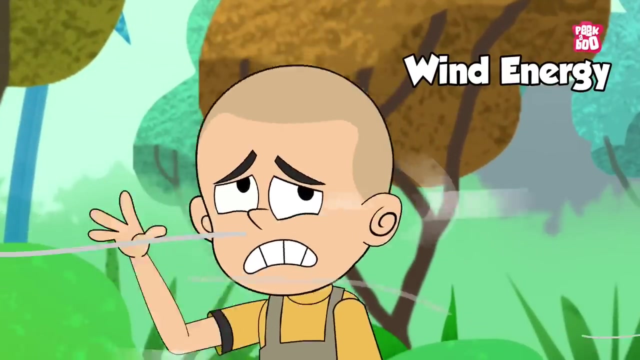 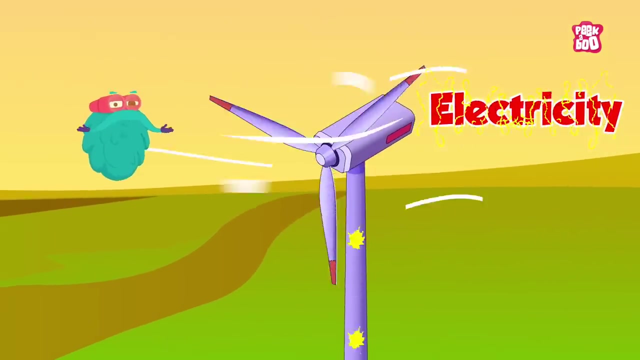 with the help of solar panels. Also, it can be converted to thermal energy to heat our homes or water. Next comes another unlimited source called wind energy, which is produced through the wind. This wind can be harnessed and converted into electricity using man-made structures called wind turbines. 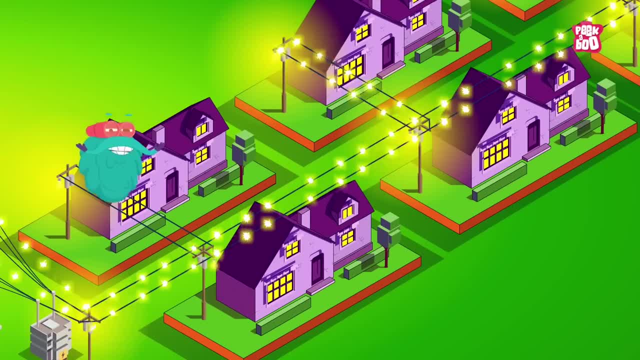 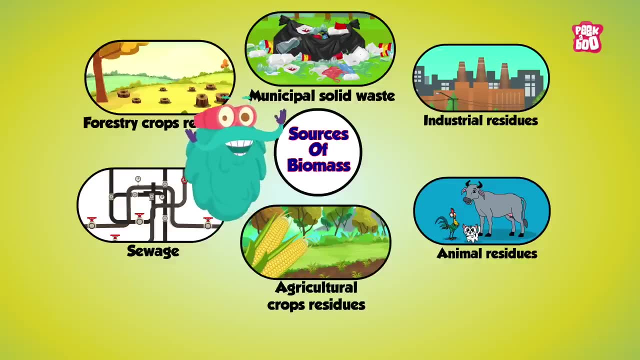 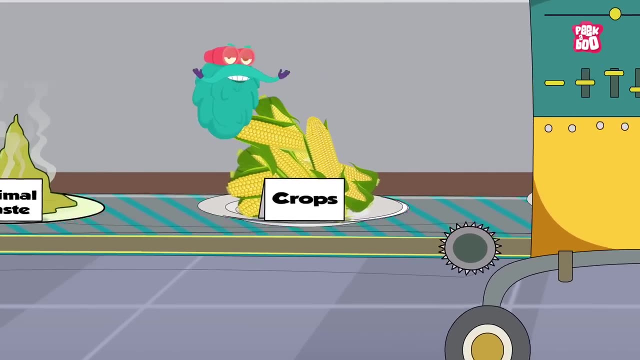 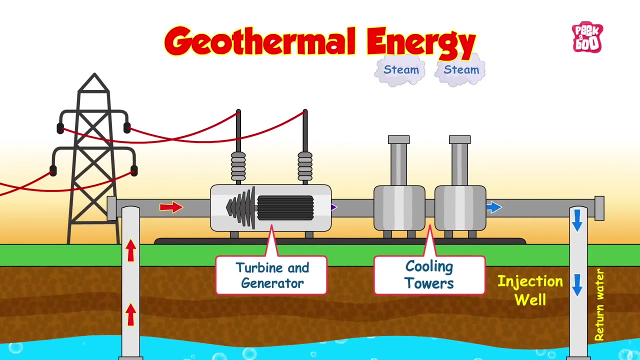 that can light up our houses and schools. Now let us look into biomass, which is renewable organic matter that comes from plants and animals. Examples of biomass include wood crops and animal waste that can be turned into fuel. Next on the list is geothermal energy. 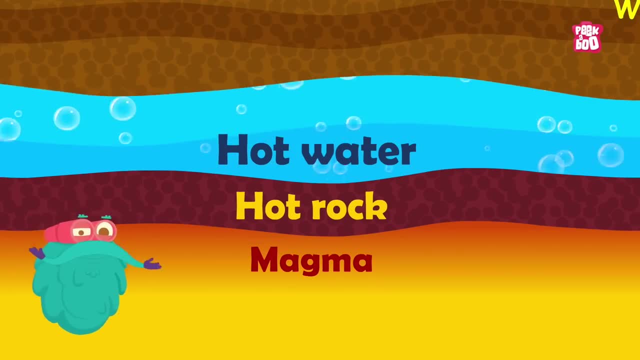 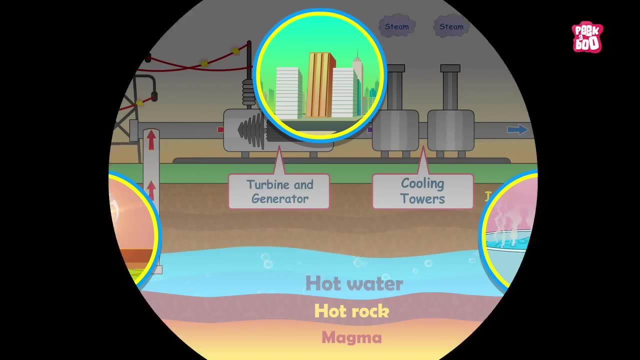 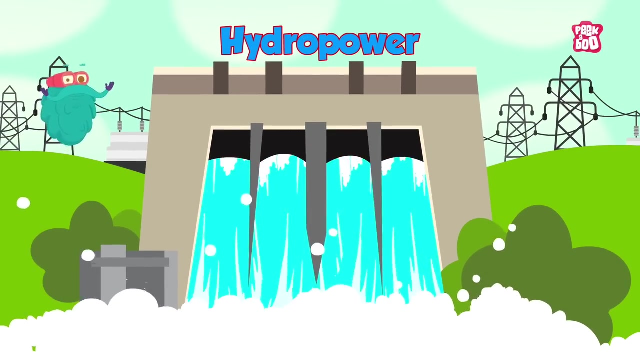 that comes from the heat inside the earth. It can be used to produce electricity, heat homes and buildings and provide hot water. Speaking of water, moving water can also produce electricity in the form of hydro power that can generate electricity. It is one of the oldest. 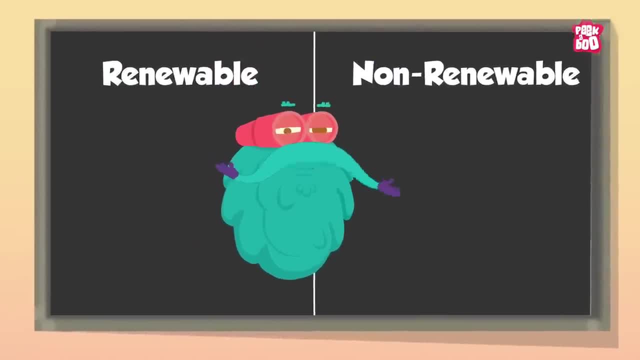 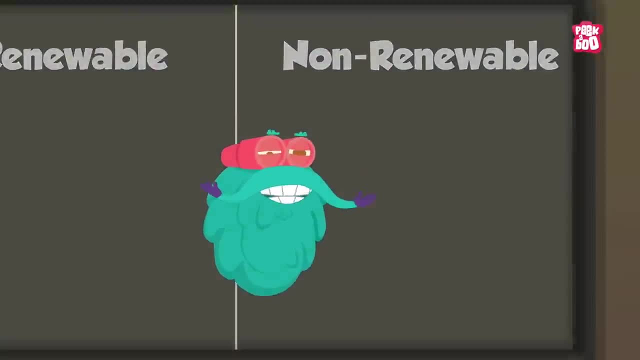 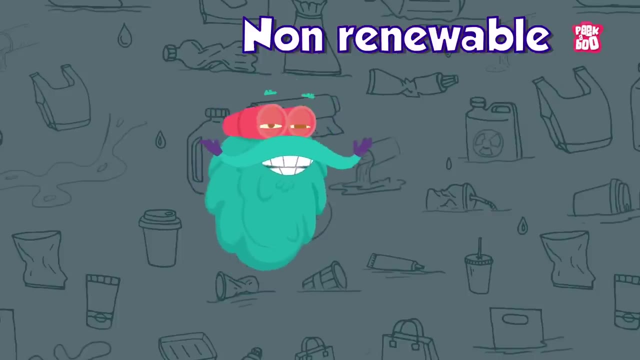 and largest sources of renewable energy. that is available in plenty on earth, But what is limited is non-renewable sources of energy that can run out of supply as time passes. Some examples of these are natural gas, coal, petroleum, nuclear energy. 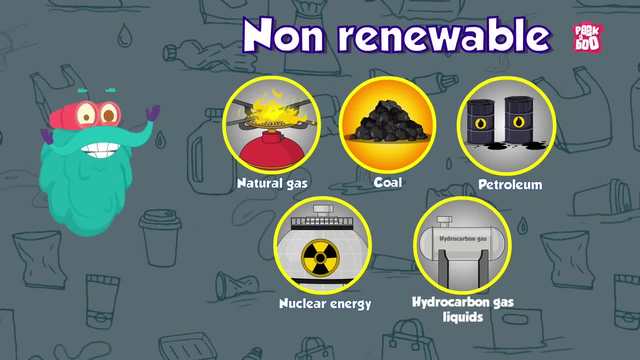 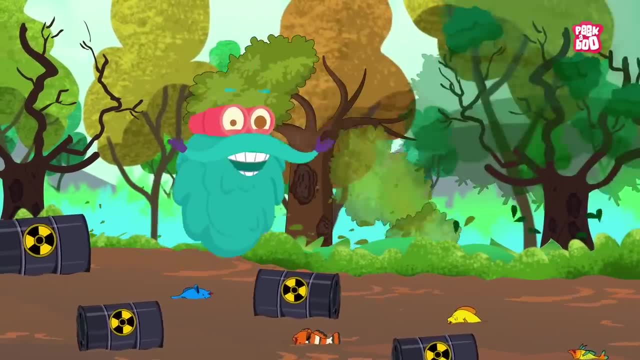 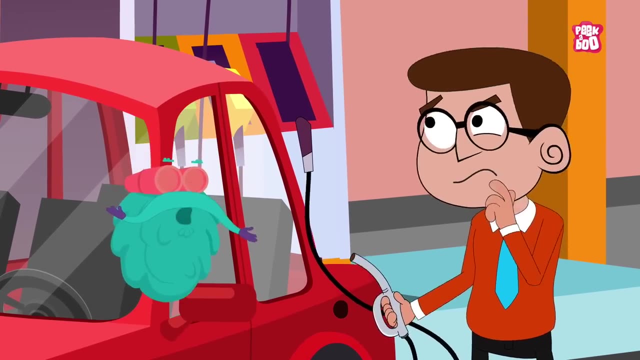 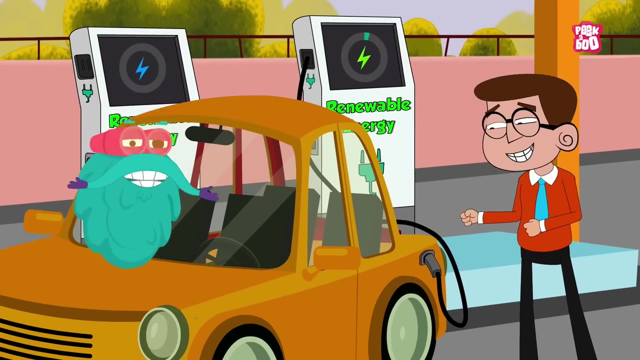 and hydrocarbon gas liquids. These are not only exhaustible, but can have an impact on the environment by causing pollution, So it is vital to limit our dependency on non-renewable sources of energy and find an alternative solution with the help of renewable source of energy. 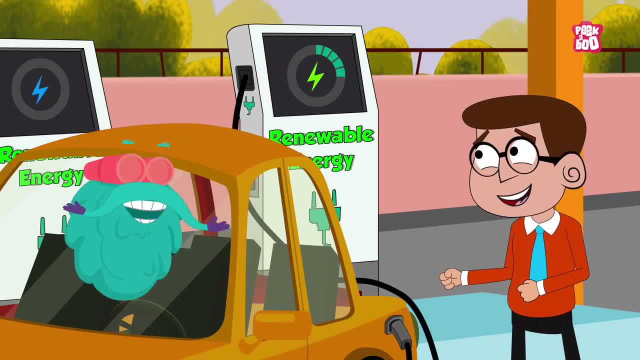 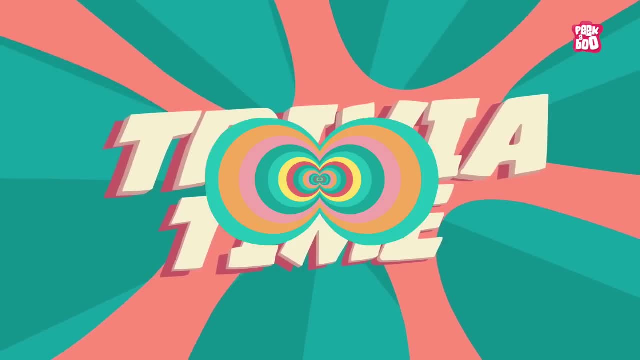 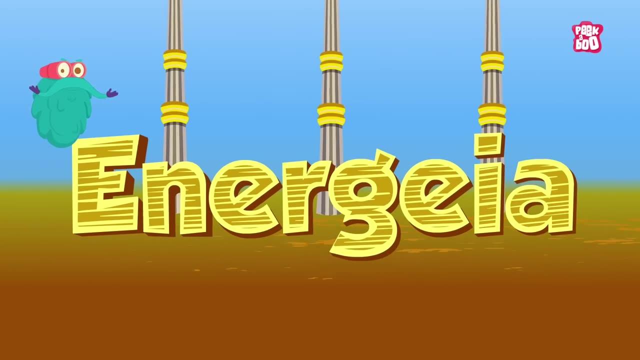 as a way to help reduce and avoid carbon dioxide emissions for a better and safer future. Trivia Time. Did you know the word energy is derived from the ancient Greek word Energia? Yes, this word was created by Aristotle in 384 BC. 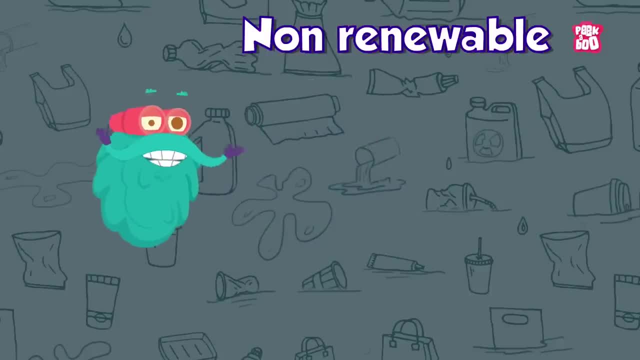 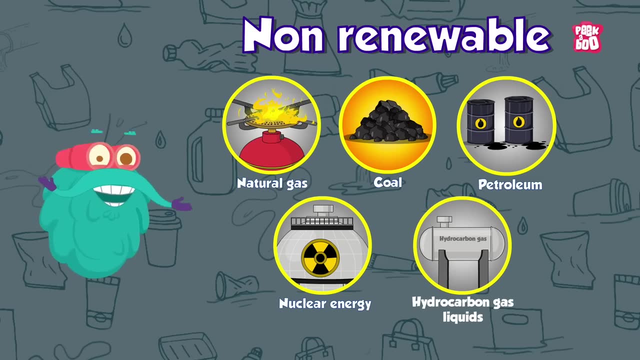 run out of supply as time passes. Some examples of these are natural gas, coal, petroleum, nuclear energy and hydrocarbon gas liquids. These are not only exhaustible, but can have an impact. 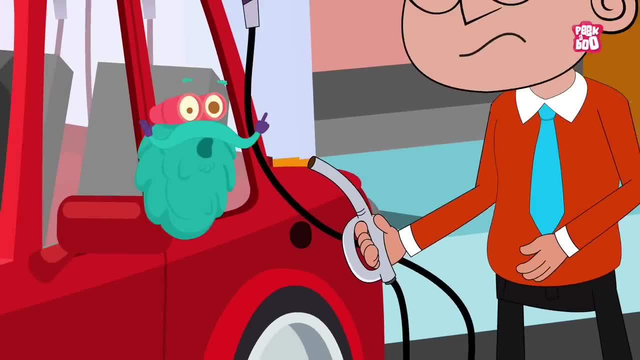 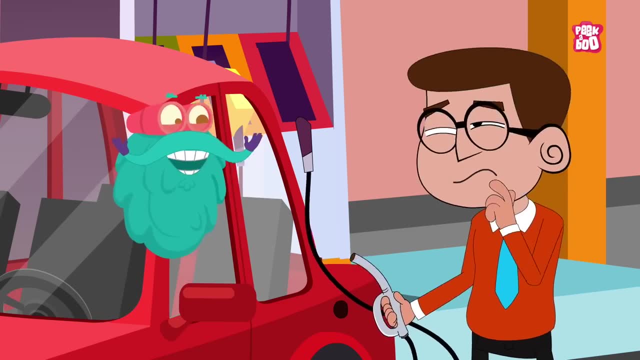 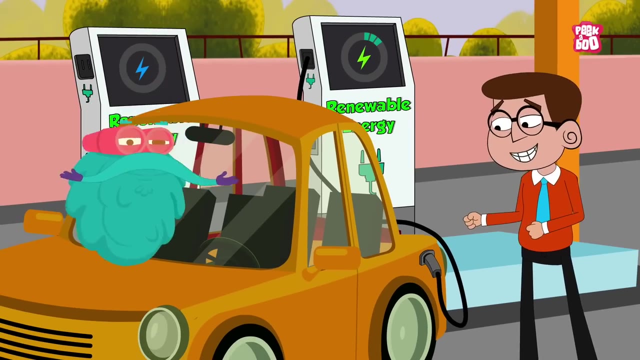 on the environment by causing pollution. So it's vital to limit our dependency on non-renewable sources of energy and find an alternative solution with the help of renewable source of energy. 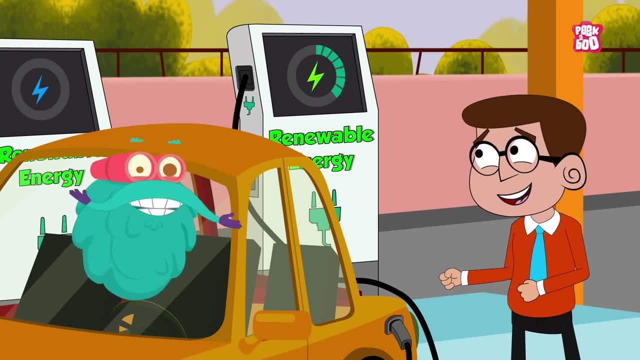 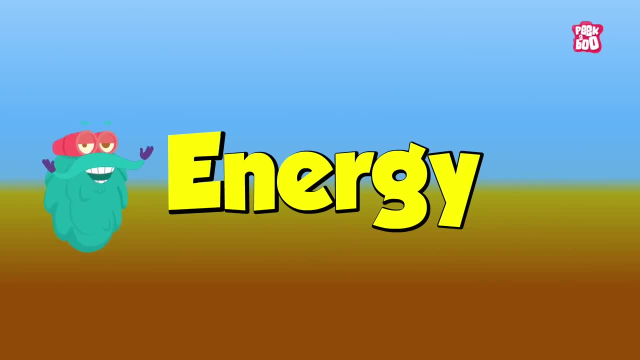 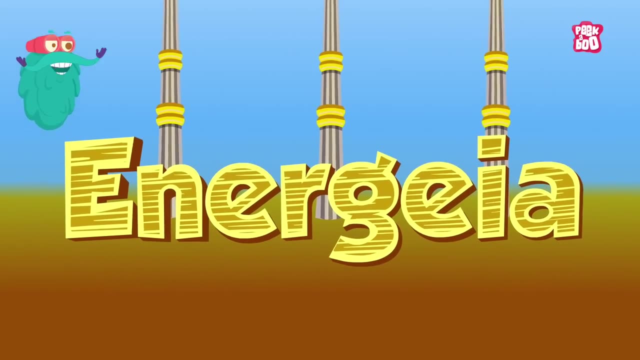 as a way to help reduce and avoid carbon dioxide emissions for a better and safer future. Did you know the word energy is derived from the ancient Greek word energia? Yes, this word. 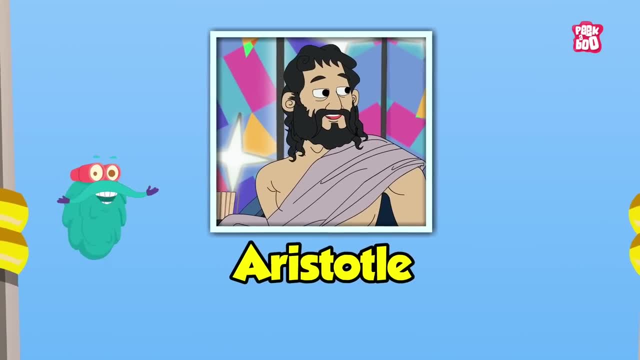 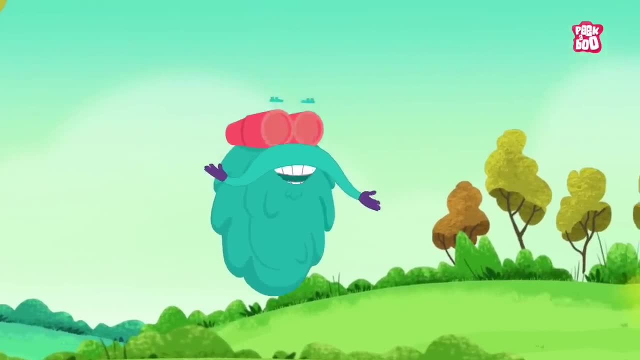 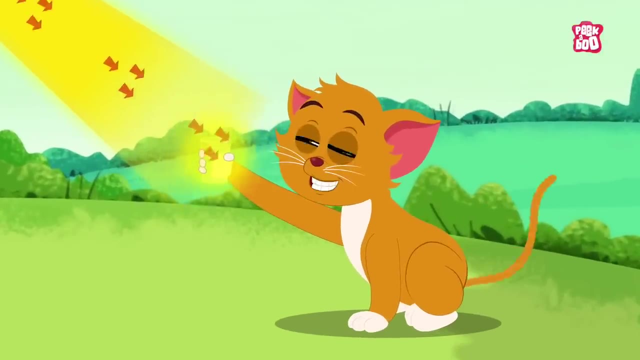 was created by Aristotle in 384, BC. Hope you learned something energetically vital today. Until next time, it's me Dr Binox Zooming Out. Thanks for watching. Please subscribe. 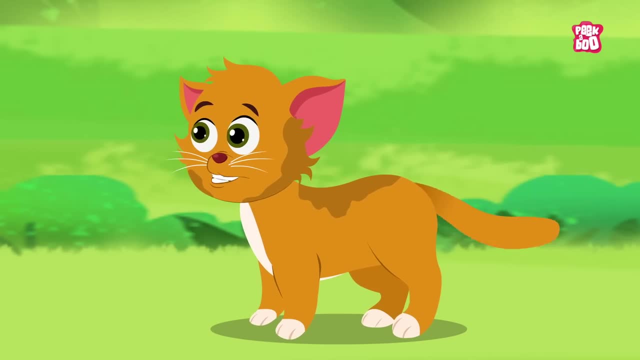 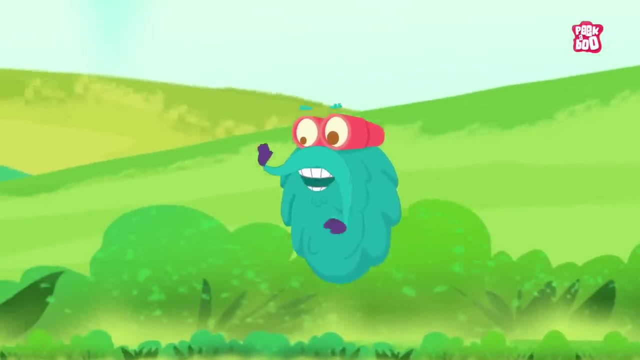 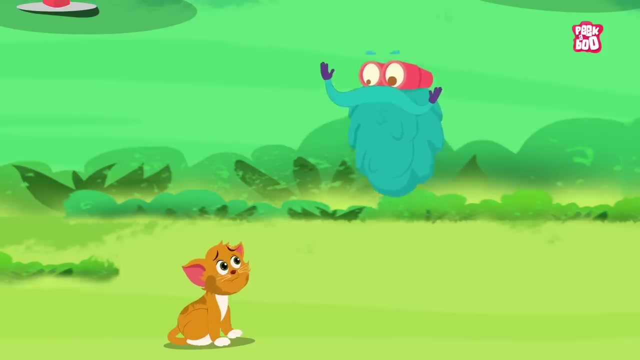 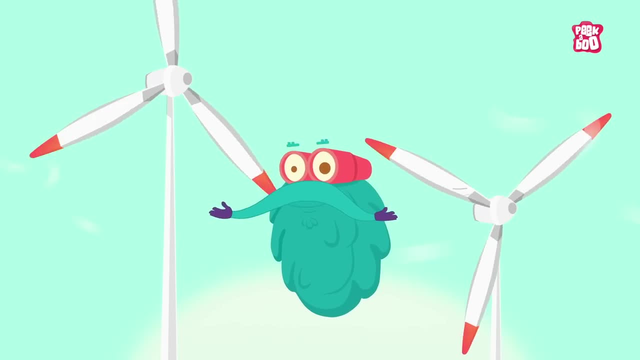 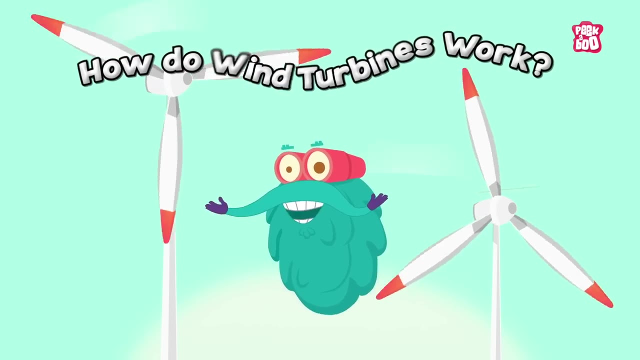 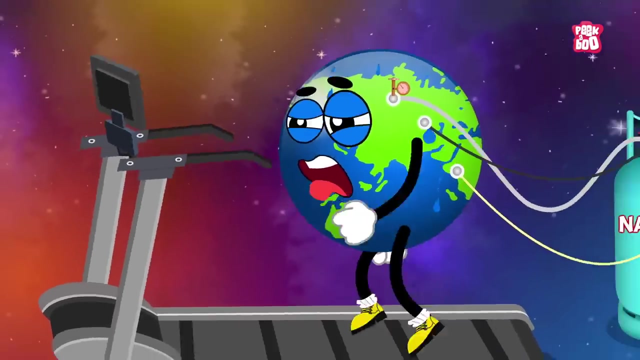 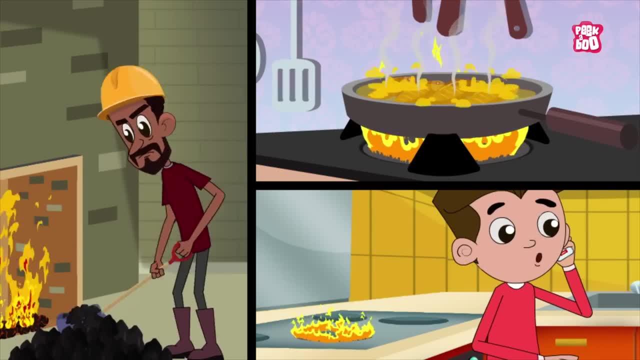 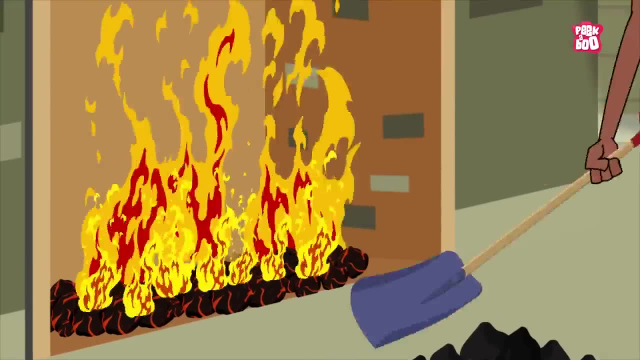 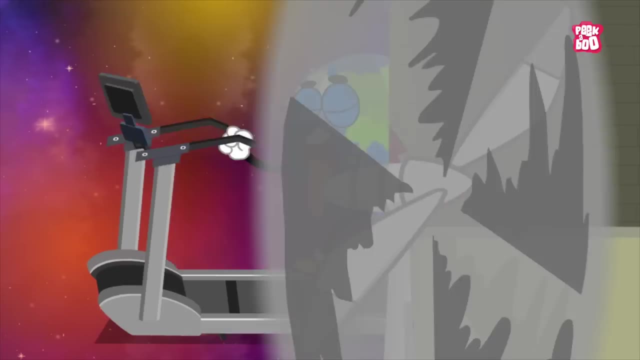 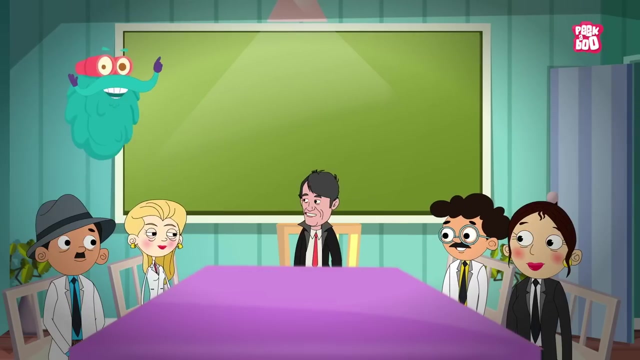 gas, et cetera, and we keep using them as if there is no tomorrow, despite their limited supply. and of these energies, there will come a time when they will go out of stock forever, bringing our world to a standstill. hence, for the past few decades, governments 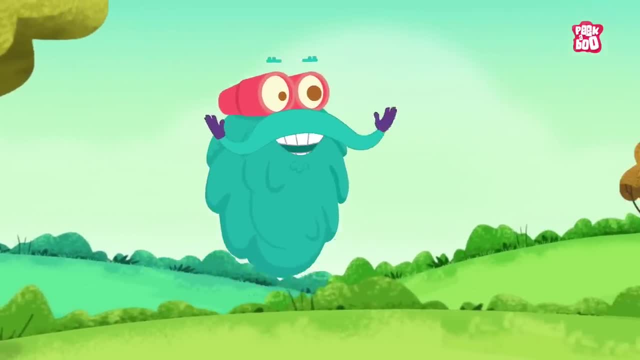 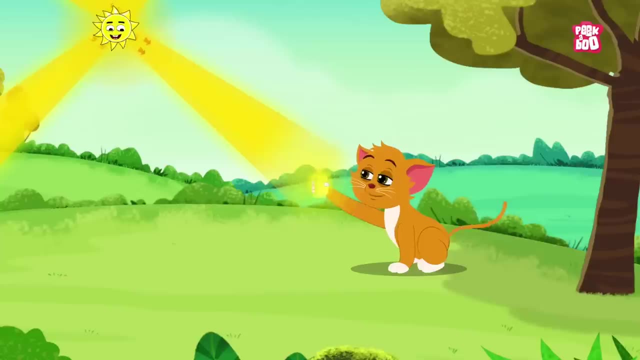 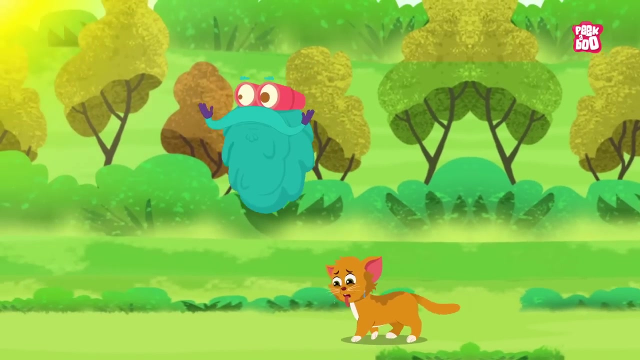 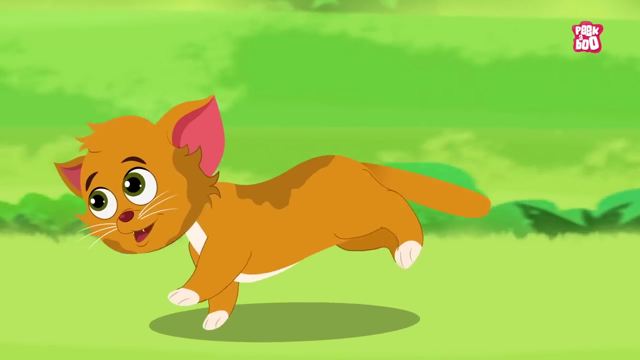 Hope you learnt something energetically vital today. Until next time it's me, Dr Binox, Zooming Out. Kitty drinks natural energy. Never mind, Yay, Fan Fan. Wait, little kitty, this isn't the fan. 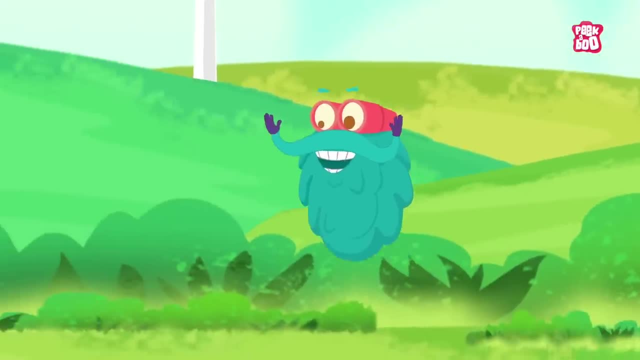 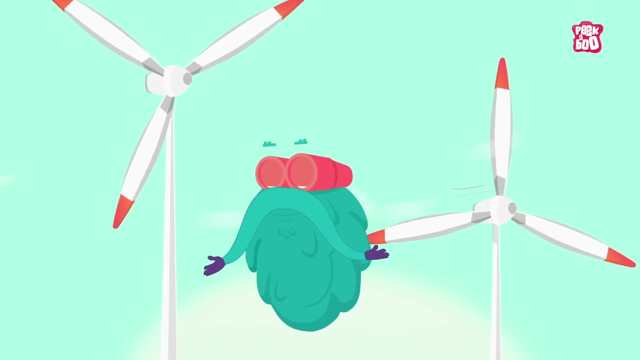 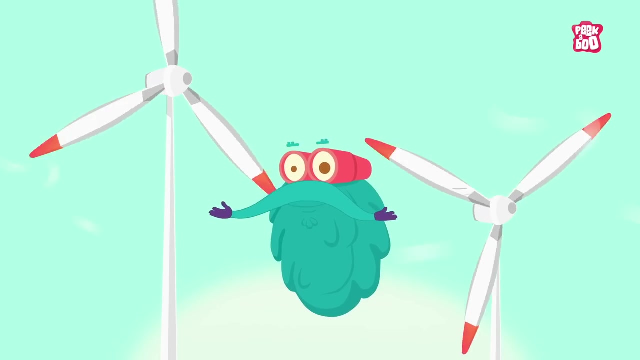 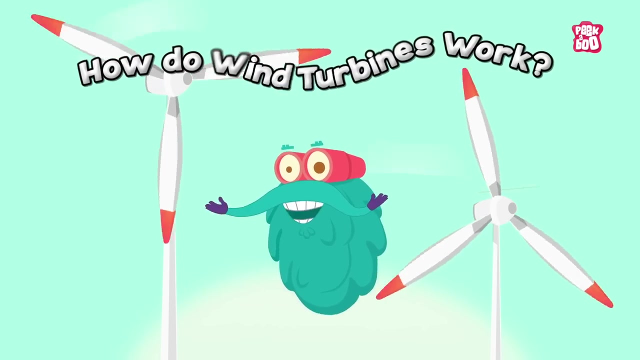 fan, but a fan to run the fan and other devices. Let me explain, Hey friends. so in today's episode let us explore these mechanical forces we called wind turbines, and blow our minds by answering a windy question: How do wind turbines work? 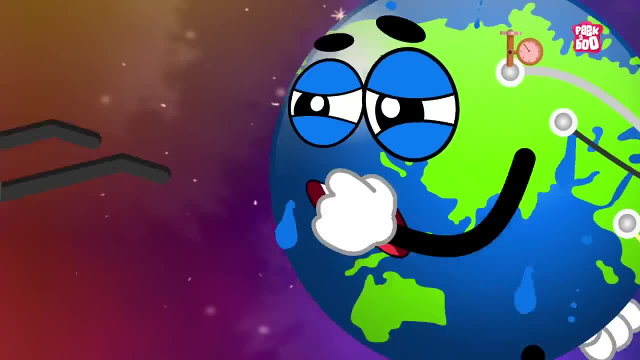 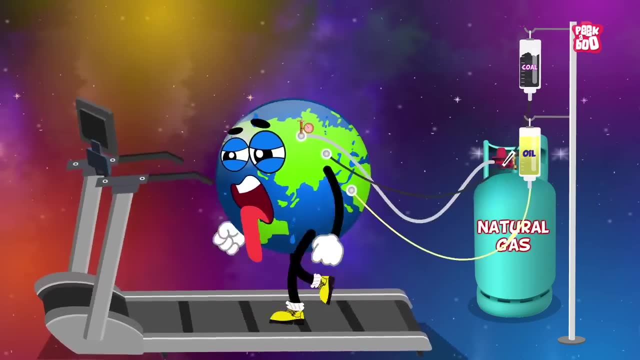 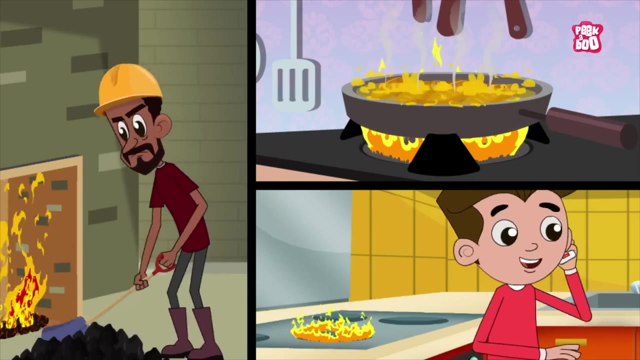 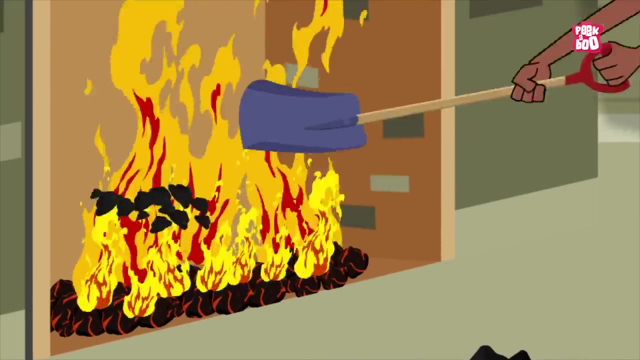 Zoom in. The world runs on sources of energy like coal, oil, petrol gas, etc. And we keep using them as if there is no tomorrow, despite their limited supply and availability. So, because of our excessive usage of these energies, there will come a time. 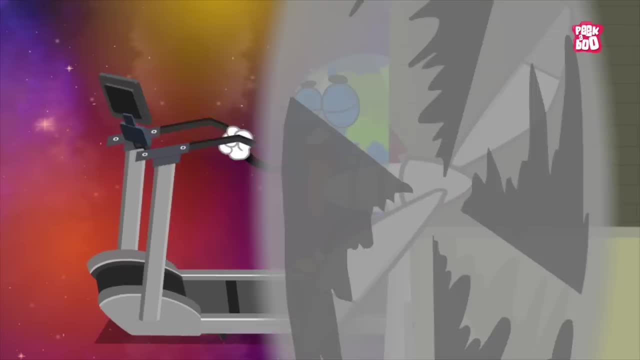 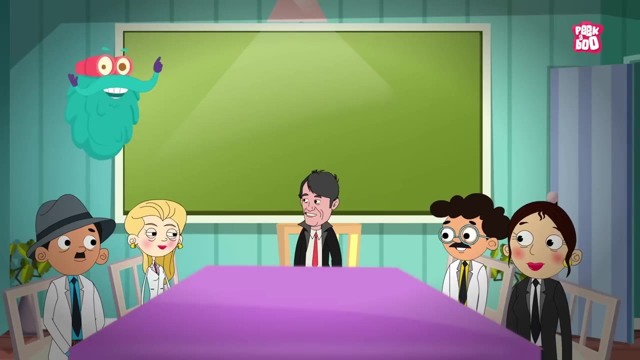 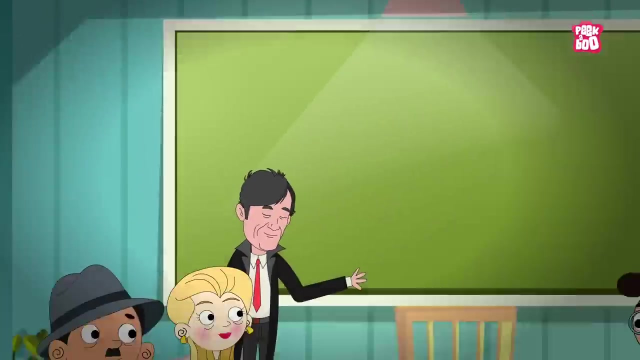 when they will go out of stock forever, bringing our world to a standstill. Hence, for the past few decades, governments around the world have started taking energy-saving initiatives that include the use of renewable sources of energy like solar panels, atomic energy, 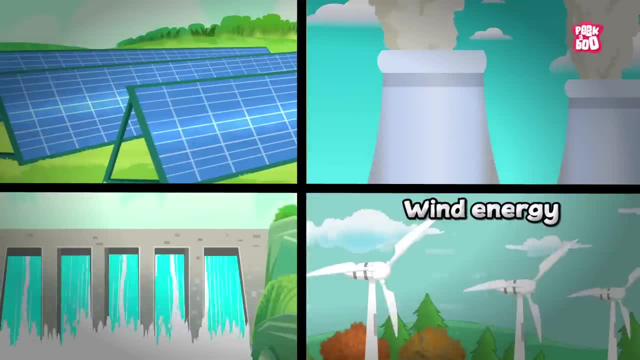 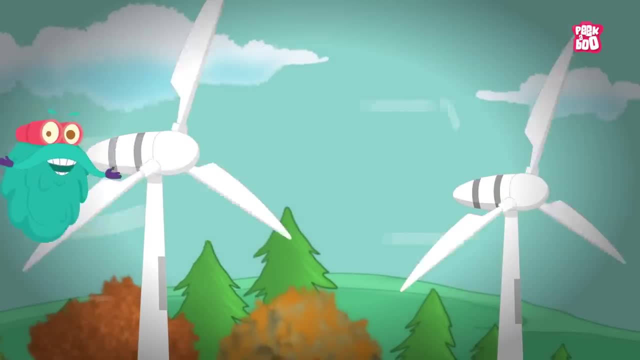 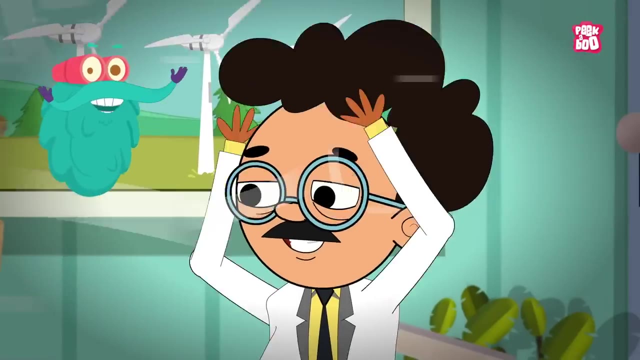 hydrothermal energy, wind energy, etc. And out of these alternatives, using wind turned out to be the most favorable source due to the abundance of air in the environment, which could be renewed every day. Plus, humans have been taming wind power. 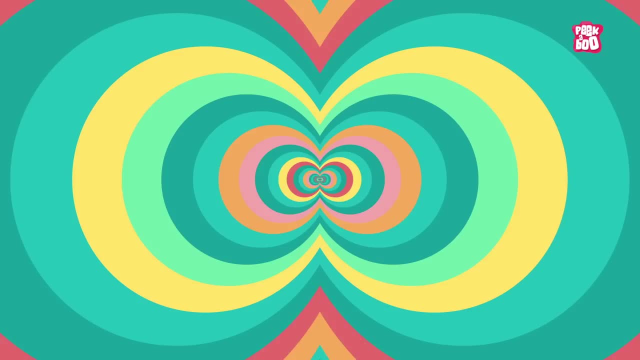 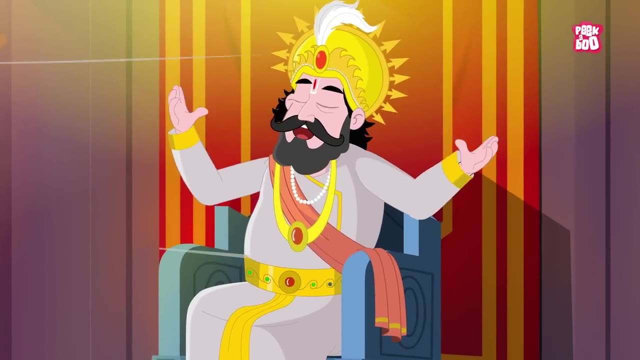 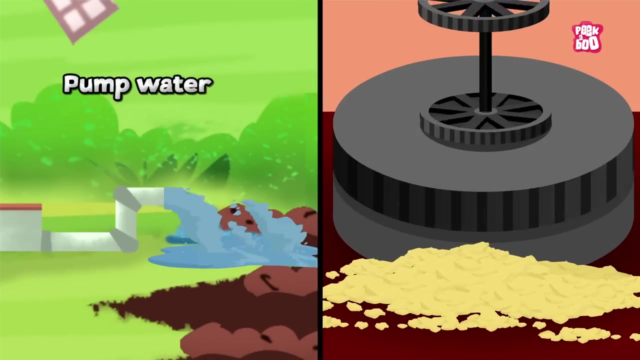 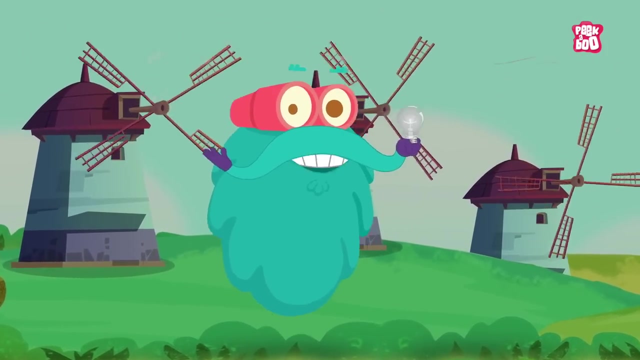 since we started. sailing boats and ships, And architects have used wind-driven natural ventilation in buildings since ancient times. Later, traditional windmills were commonly used to pump water and grind grains. Now the only question was to convert this free-flowing resource into electric energy. 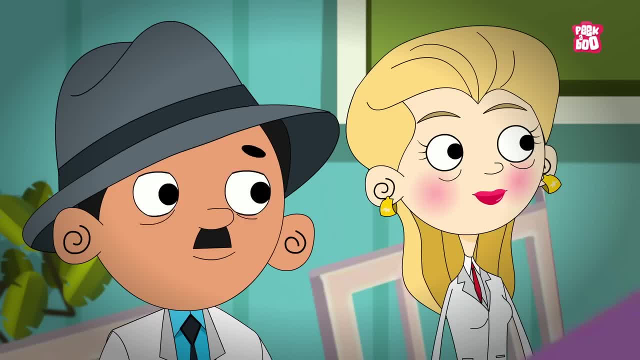 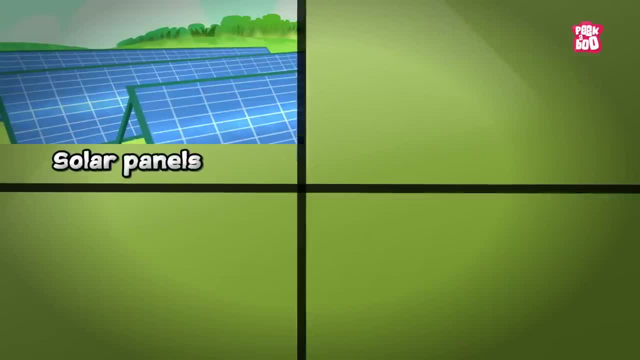 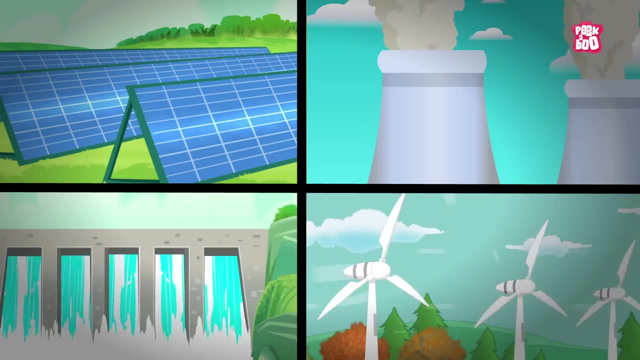 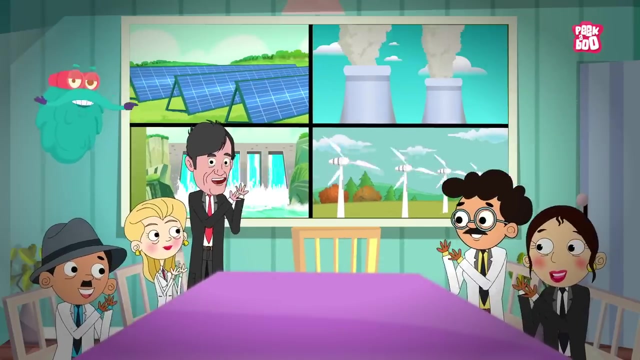 around the world have started taking energy saving initiatives that include the use of renewable sources of energy like solar panels, atomic energy, hydrothermal energy, wind energy, etc. and out of these alternatives, using wind turned out to be the most favorable source due to the abundance of air in. 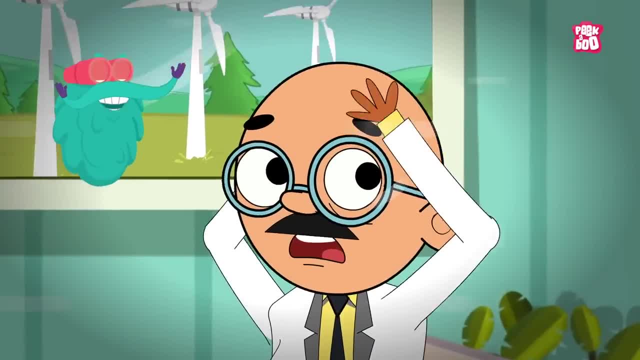 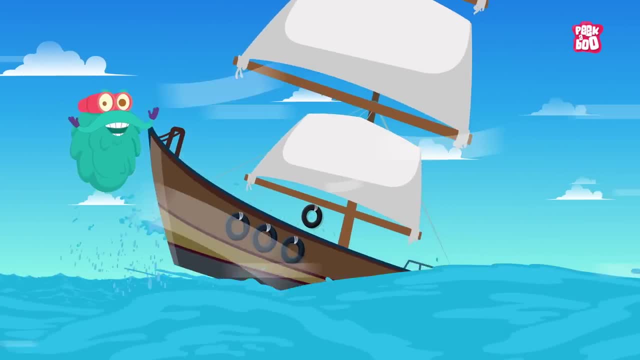 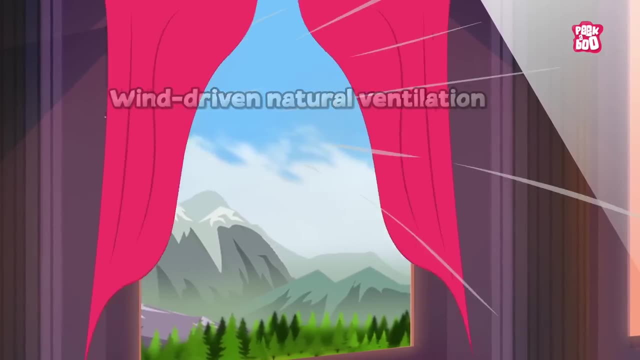 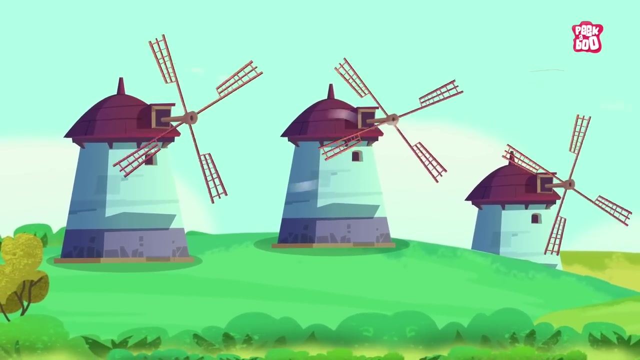 the environment, which could be renewed every day. plus, humans have been taming wind power since we started sailing boats and ships and architects have used wind-driven energy to save the planet. natural ventilation in buildings since ancient times. later, traditional windmills were commonly used to pump water and grind grains. now the only 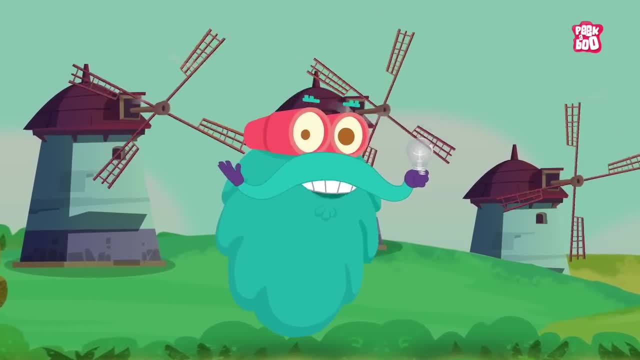 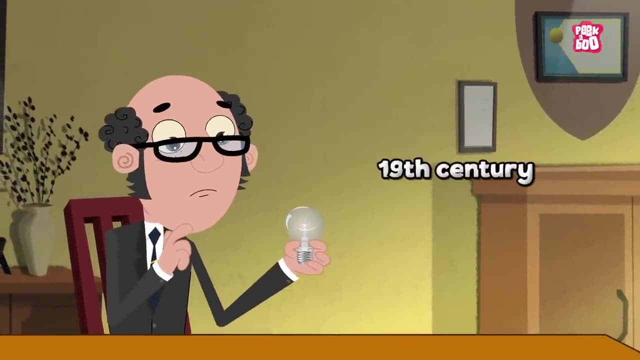 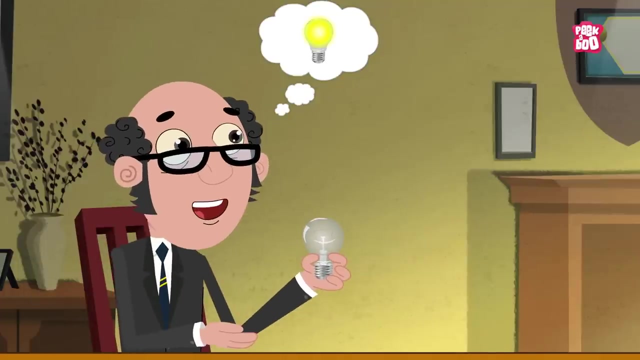 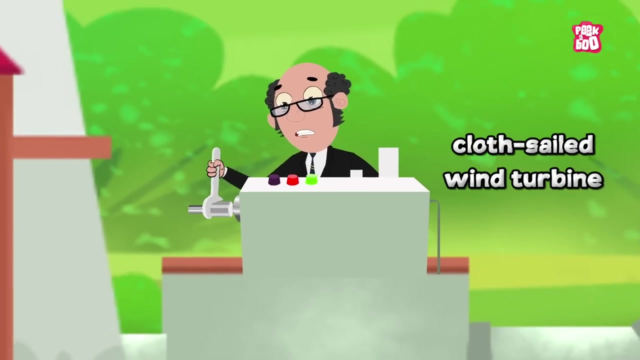 question was to convert this free-flowing resource into electric energy. so in the late 19th century a Scottish electric engineer, Professor James Bush, was one of the first to introduce wind power to the world. he took this challenge and in July 1887 he built a cloth sailed wind turbine in 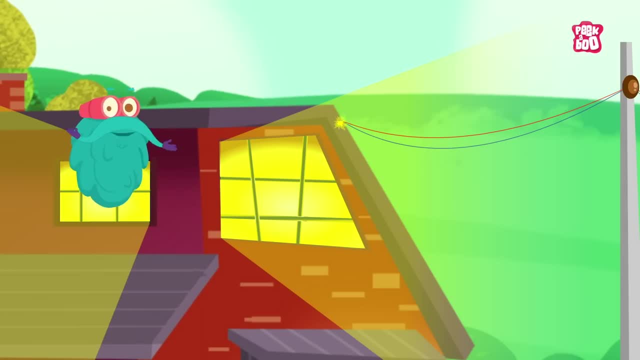 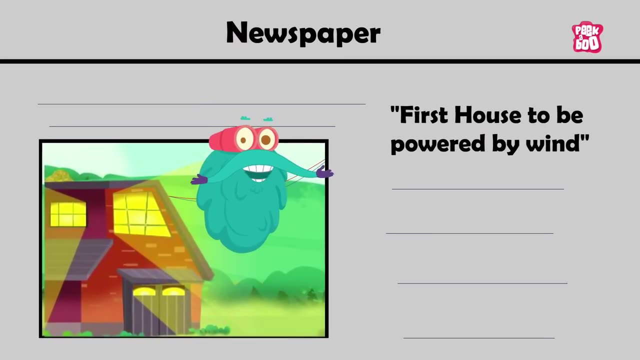 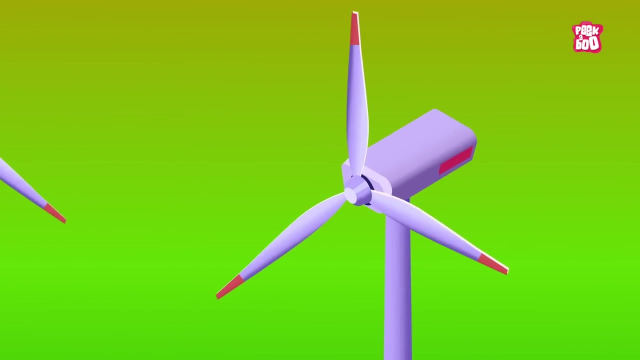 his garden that generated current to power lights in his cottage, which thus became the first house in the world to be powered by wind generated electricity. let me explain how you see. when the wind moves, the kinetic energy of the wind is cut into two, and the energetic 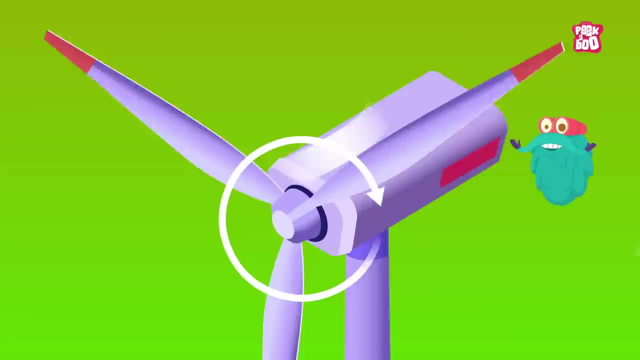 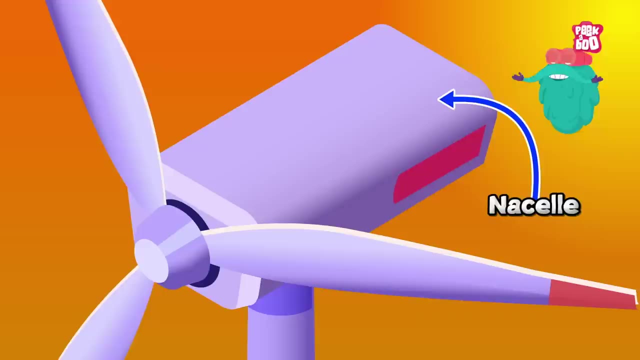 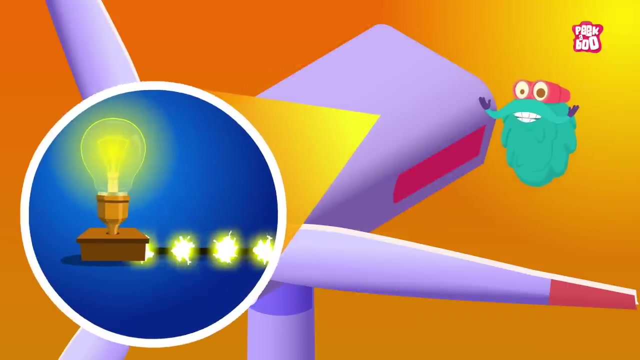 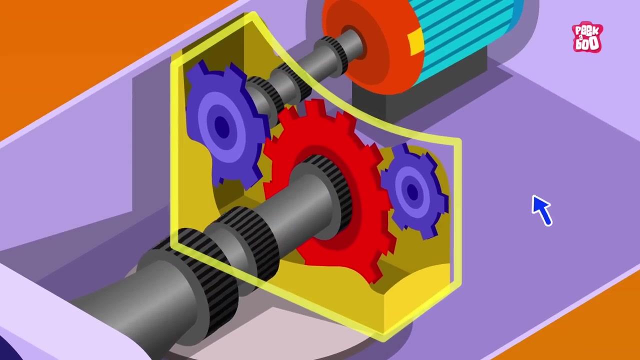 contained in the air currents rotates the turbine's blade. the blades are then attached with a low speed shaft located in the nasal and box, like structure at the top of a wind turbine. but to produce electricity it's essential to increase the speed of the low shift shaft, and that's when the gearbox comes into play. which accelerates thevous mainerten of the boat ability and even increases the speed of goes shaft. and that's when the gearbox comes into play, which accelerates the speed of the sending wind enough to make the wind soft and powerful wind fan not to be in contact with the ship beneath the beginning. 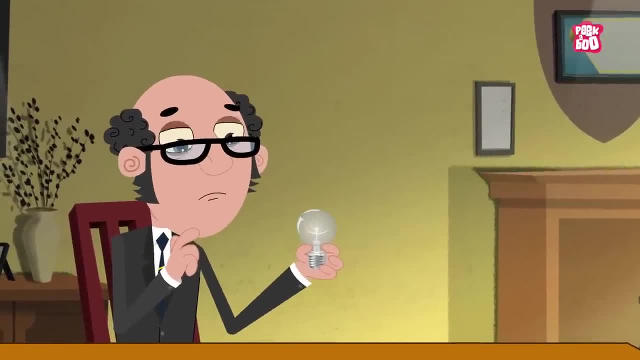 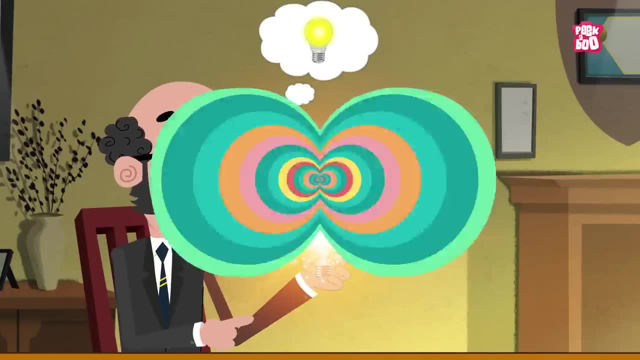 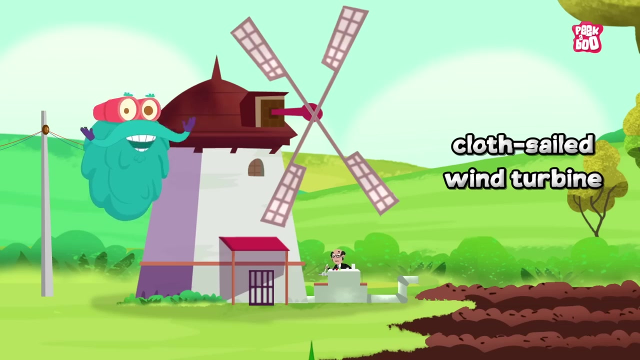 So in the late 19th century a Scottish electric engineer, Professor James Blyth, took this challenge, And in July 1887, he built a cloth-sailed wind turbine in his garden that generated current to power lights in his cottage. 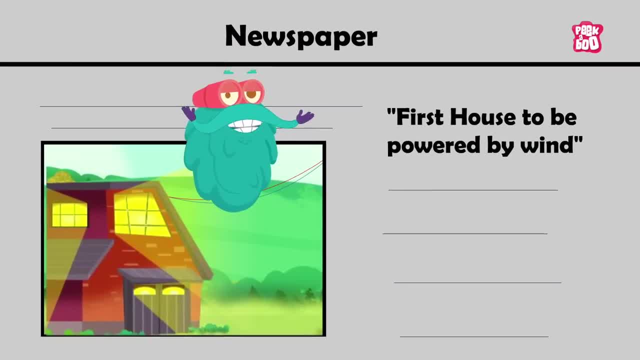 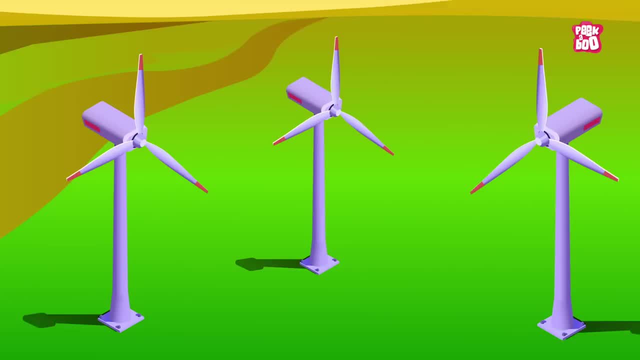 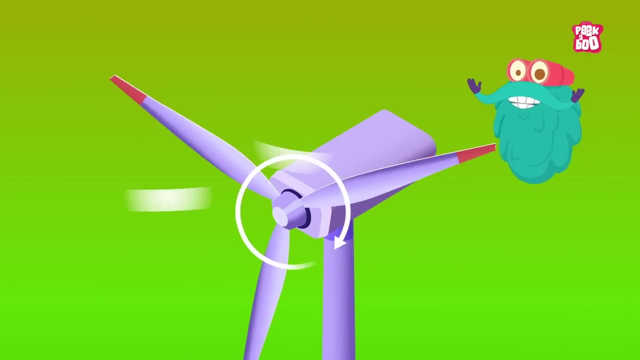 which thus became the first house in the world to be powered by wind-generated electricity. Let me explain how You see. when the wind moves, the kinetic energy contained in the air currents rotates the turbine's blade. The blades are then attached with a low-speed shaft. 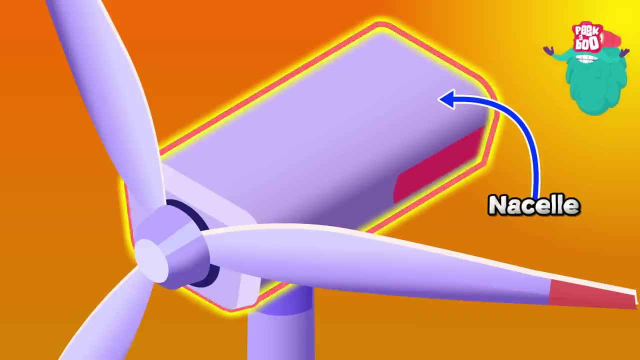 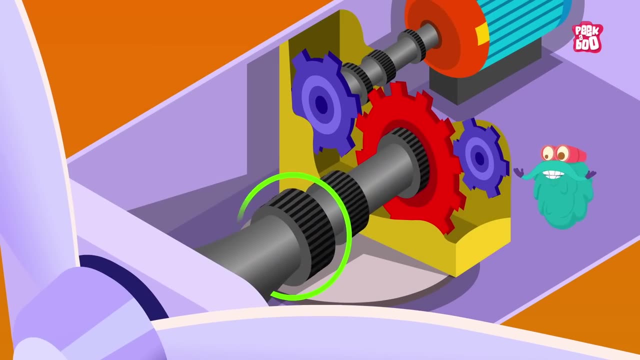 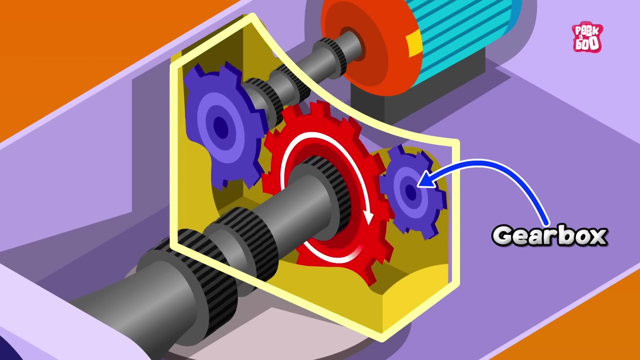 located in the nacelle and box-like structure at the top of a wind turbine. But to produce electricity it's essential to increase the speed of the low-shift shaft, And that's when the gearbox comes into play, which accelerates the speed over 100 times. 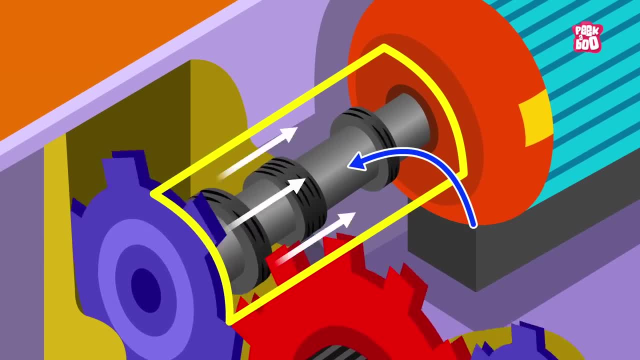 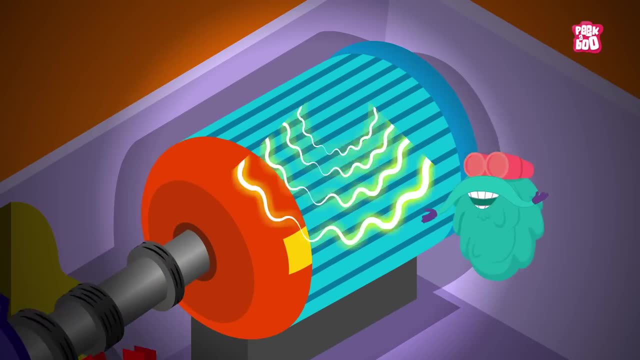 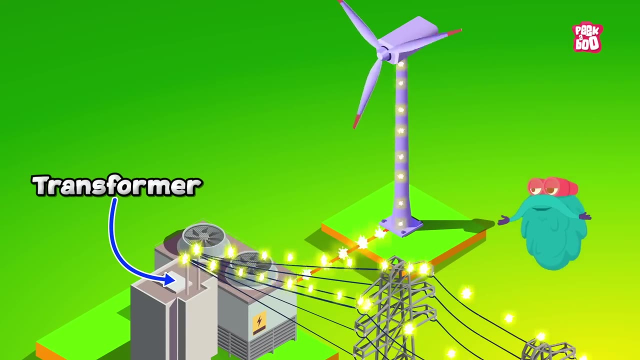 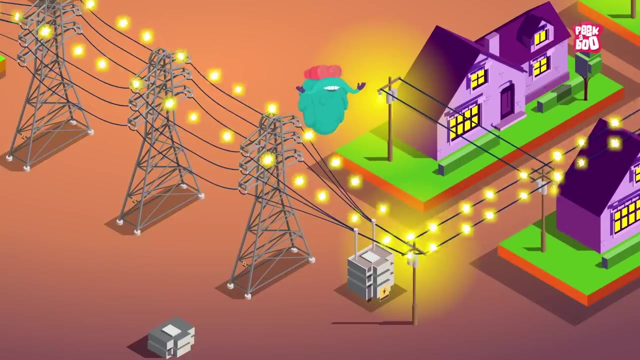 and transfers it to the high-speed shaft, which is connected to a generator that converts the kinetic energy into electricity. This electrical energy then passes through a transformer that steps up the voltage, to be transported on the national grid or used by the local sites to light up the world around us. 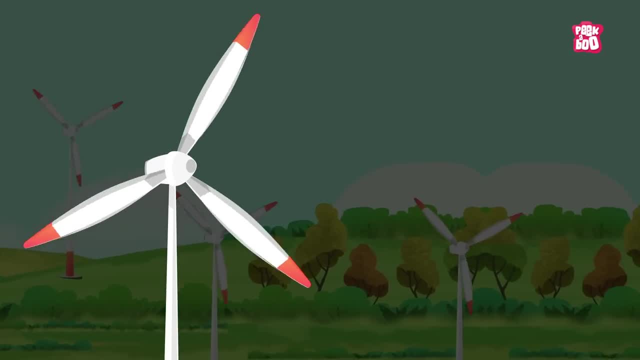 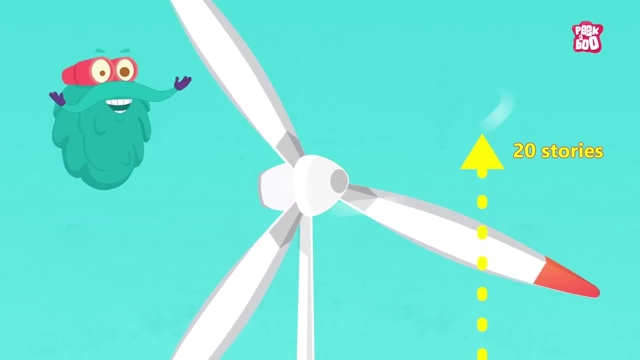 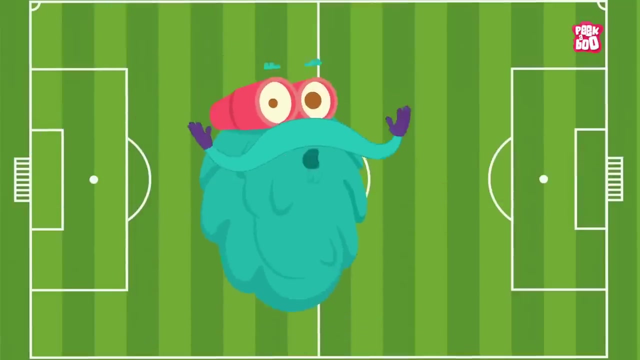 Did you know the largest wind turbine in the world is located in the US, in Hawaii. Yes, it stands 20 stories tall and has blades the length of a football field. That's huge, Really huge. Hope you learned something new today. 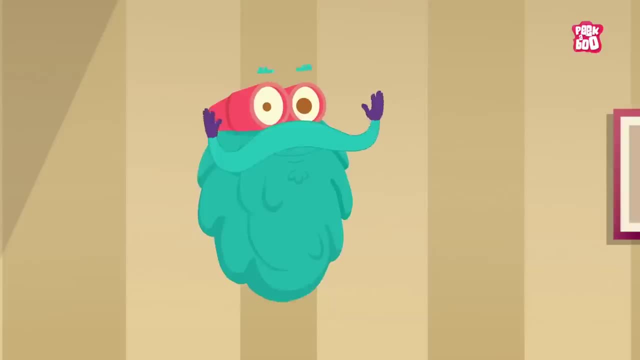 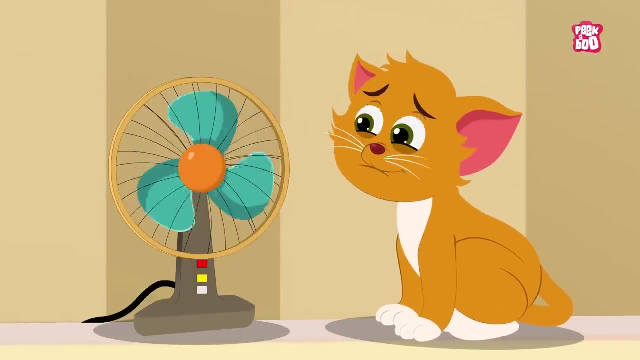 Until next time, it's me, Dr Binox, Zooming Out. Ah, Never mind.